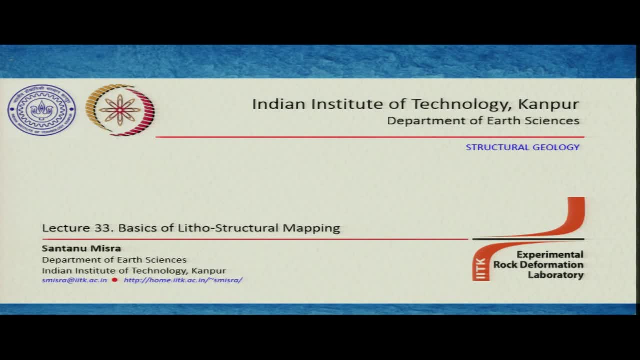 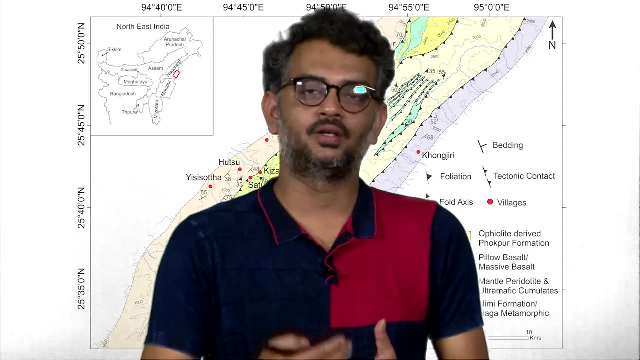 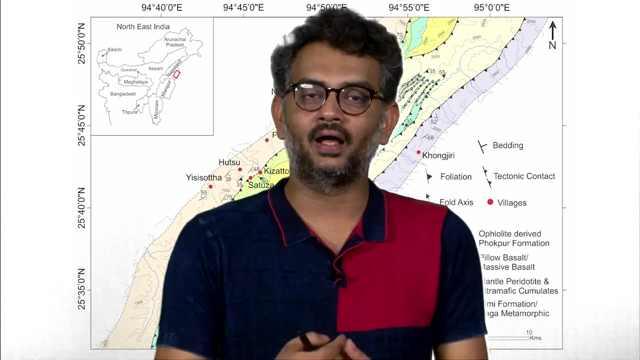 or less, have learnt the basics of structural geology Since the very beginning. we understood the different processes, then we understood stress strain. we learnt how to measure deep and strike different structural elements. Out of that we moved to the rheology, the 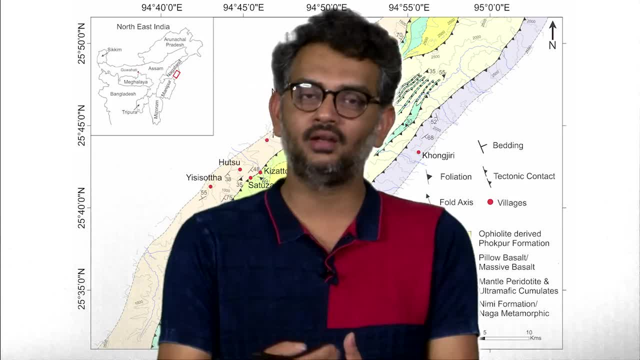 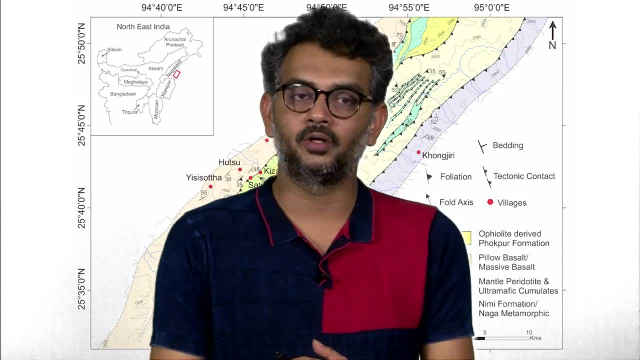 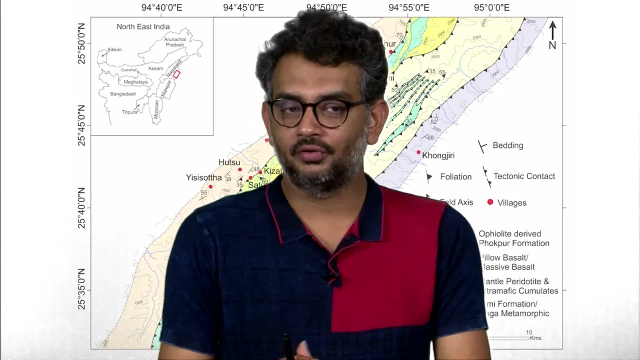 deformation mechanism, We learnt a series of important structures, their characteristics, geometries, how to interpret them, and these included fold, fault joints, buddhinas and so on. In this lecture, we will particularly focus on the basics of litho structural mapping. 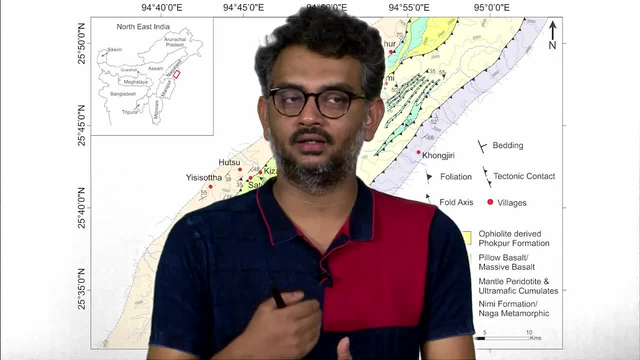 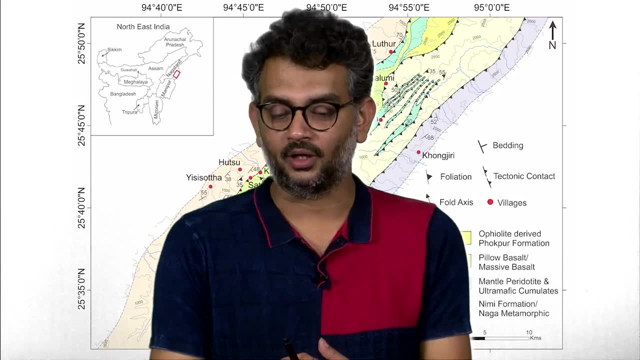 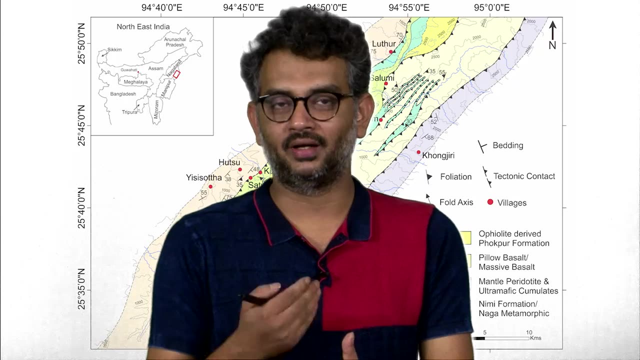 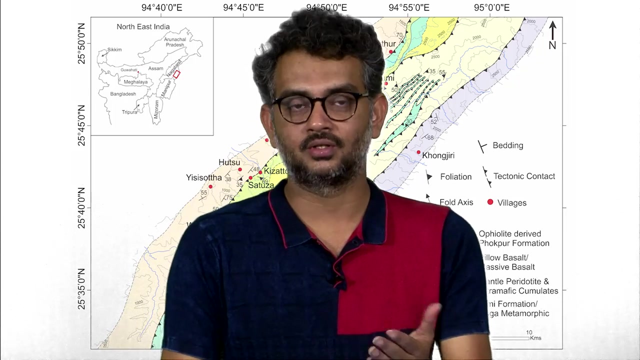 As a geologist, it is very, very important that he or she knows the basics or the methods of geological mapping. Nowadays there are many techniques which are digitized or there are many equipments which are essentially helpful or reduces time, and also you do not have to go to the field always. Some you can use, some satellite images and you can use 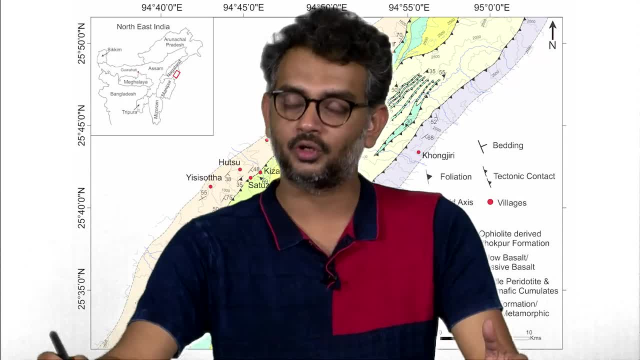 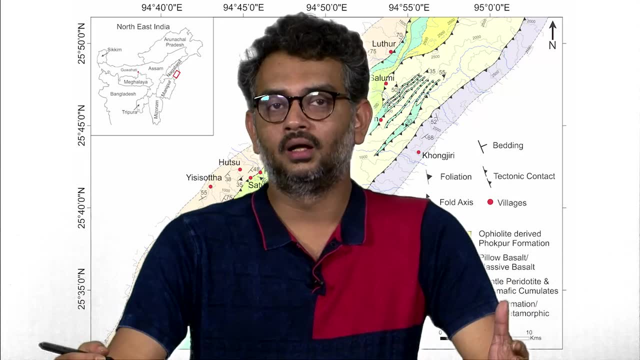 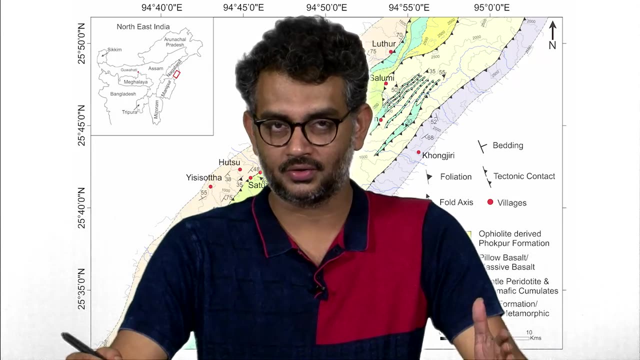 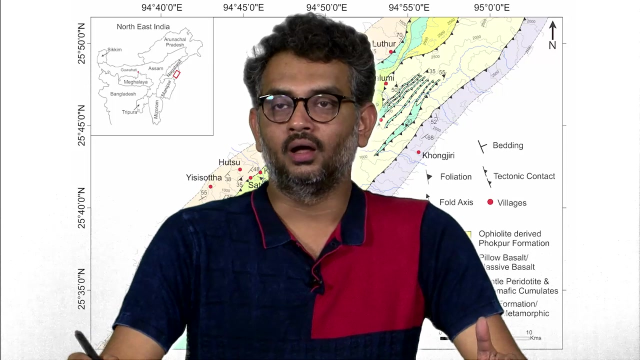 several techniques or modeling techniques, to interpret some very interesting geological features that sometimes you cannot interpret going to the field As an undergraduate student. it is important that you understand the basics of structural geology and its mapping techniques. This lecture will particularly focus on that. Having said this, I must say that structural 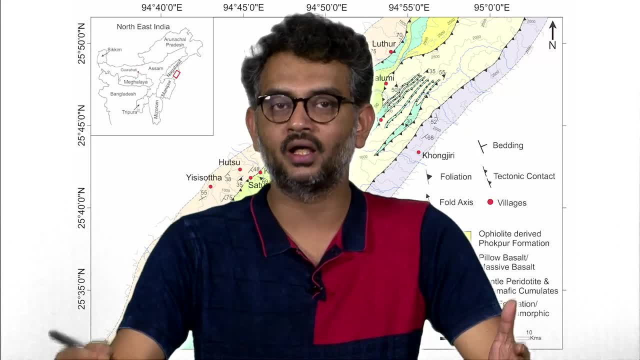 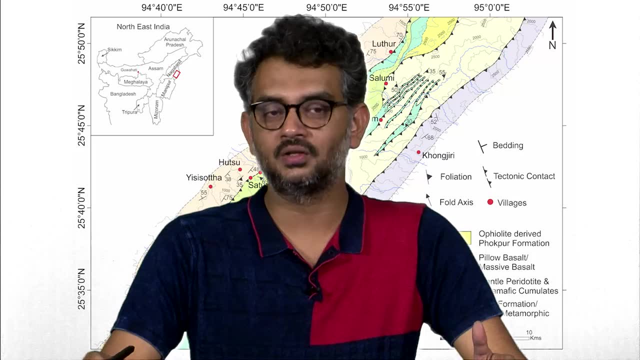 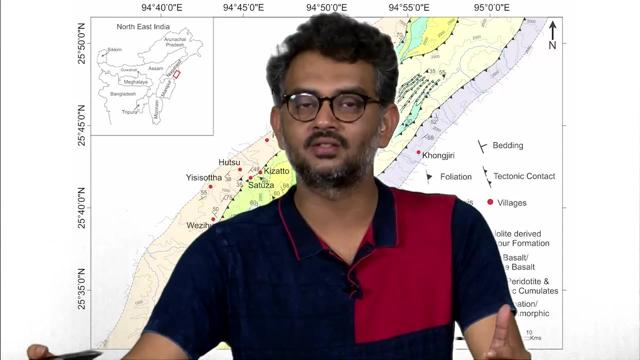 mapping, or geological mapping, is something that one has to learn in the field, and, because this is an online course, it is not possible to demonstrate all these techniques. What I have Included in this lecture is mostly some very basics, in the sense that so far we have learnt. 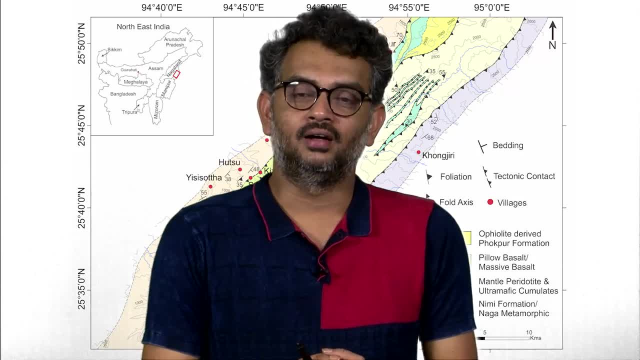 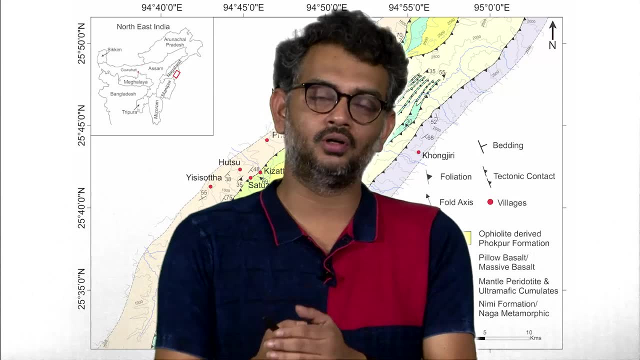 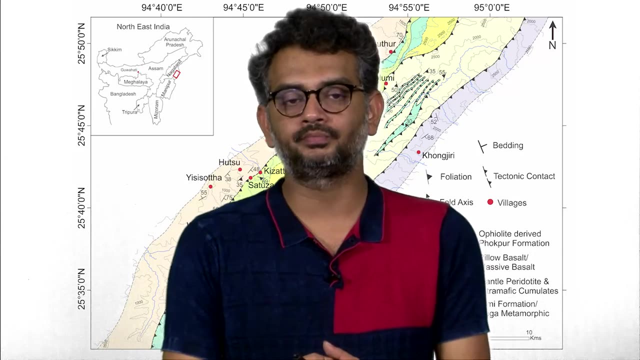 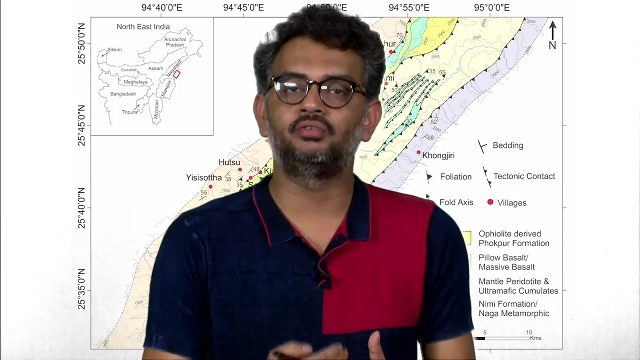 about the structures, their geometries and so on. These we mostly considered about their geometries, their dispositions and so on, and we restricted them inside a block diagram, either in three dimension or two dimensions. Now we have not considered the technology that how they would look like in the field. Well, we have seen some outcrop patterns of 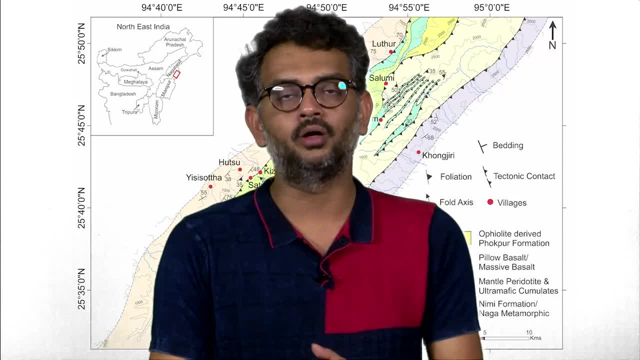 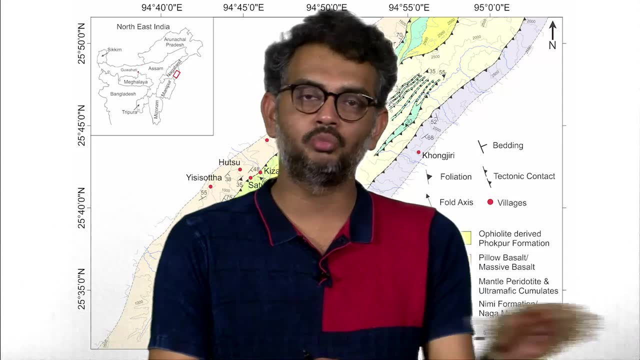 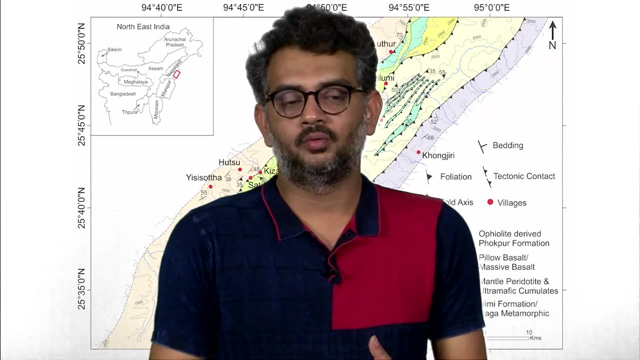 superposed folds and so on. also it we learnt about them in the fault lectures. but again, the surfaces that we constructed, that this would be the map view, was essentially a flat surfaces, is not it? but you know that earth surface is not flat, Even within 10 or 20. 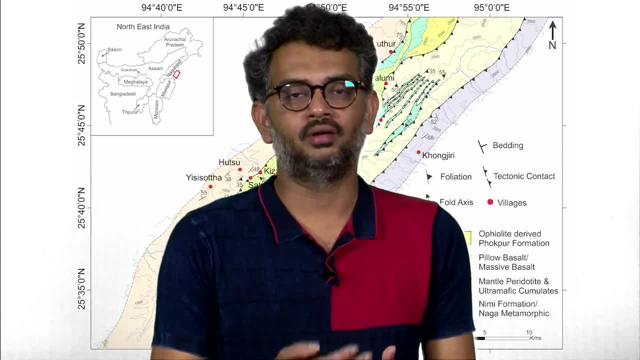 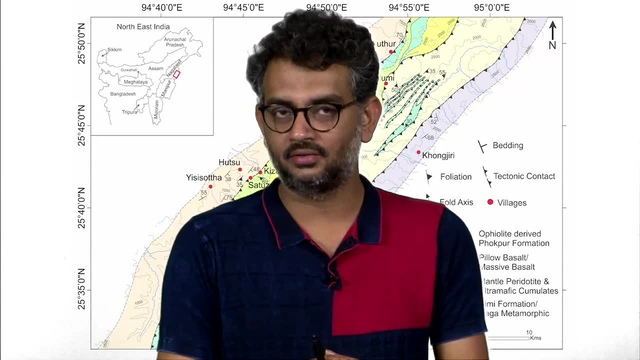 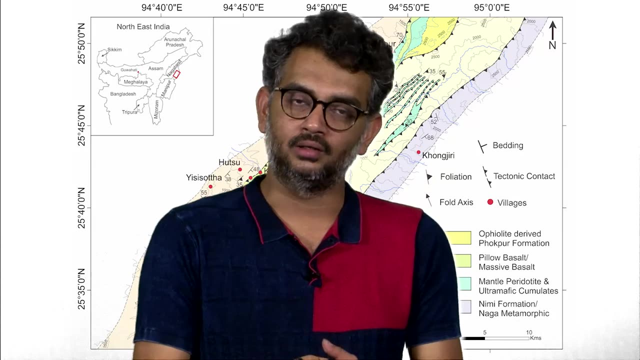 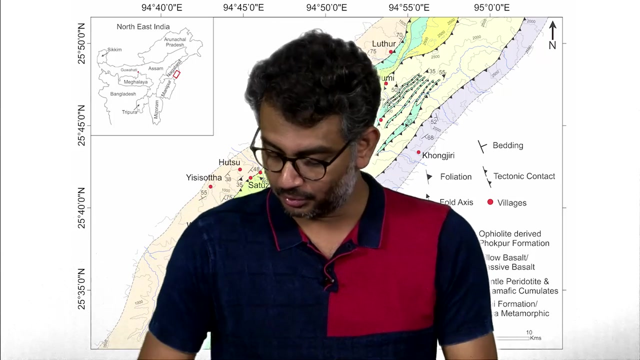 or 15 meters, it can be extremely undulatory and therefore the interaction of the structures with the earth surface is something very important to consider and understand, to particularly figure out the local and regional structures. In this lecture we will mostly focus on that and we will figure out the processes that. 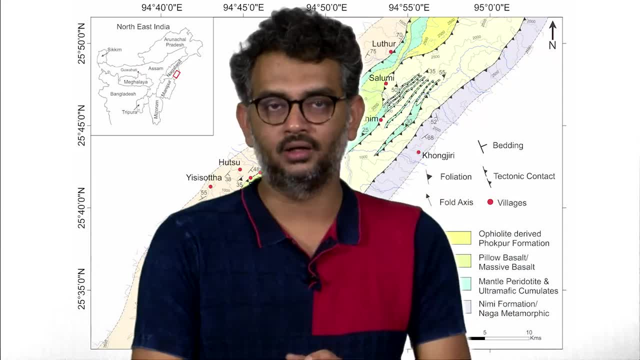 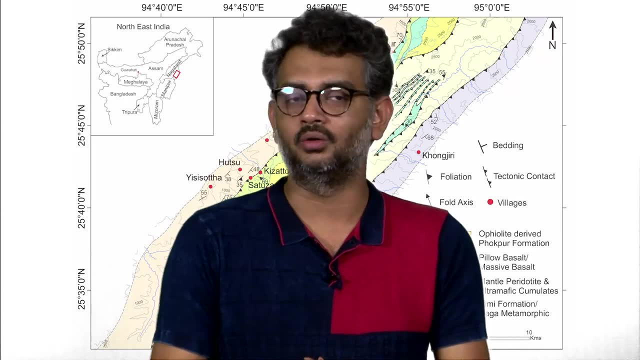 One can have some idea about lithostructural mapping. We will learn some very basics. we will not go into the complex structures. we even do not go. even deformed structures, For example, we will not going to. 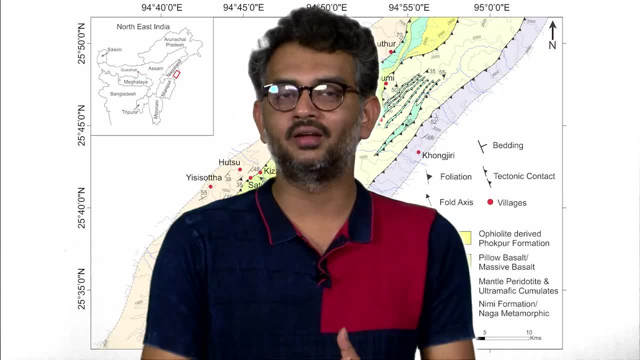 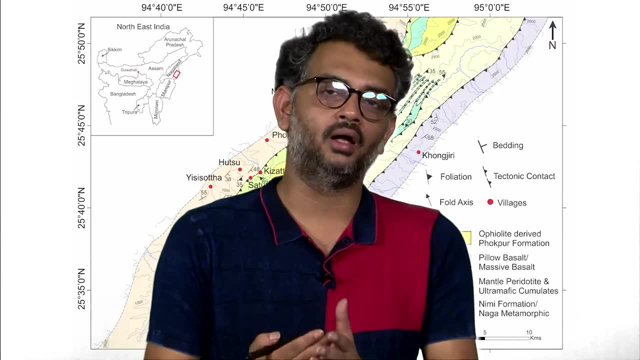 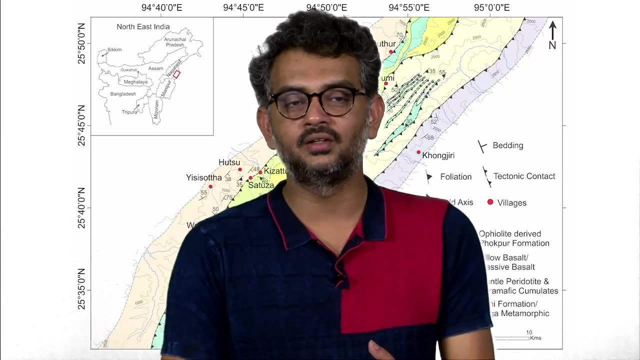 include fold fault and so on, but we mostly restrict ourself on a flat bed which is dipping differently and we will see how and why we can interpret different structural features out of it. Continuing this, we will learn in this lecture some very basic formats and composition of a. 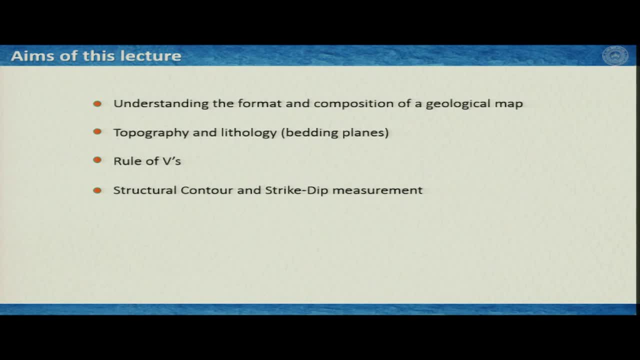 geological map, Then we will try to understand what is a topography and its interaction with the lithology and mostly bedding planes or any planar fabrics, that how they interact with each other. After that we will see. when you are discussing this topography and lithology, 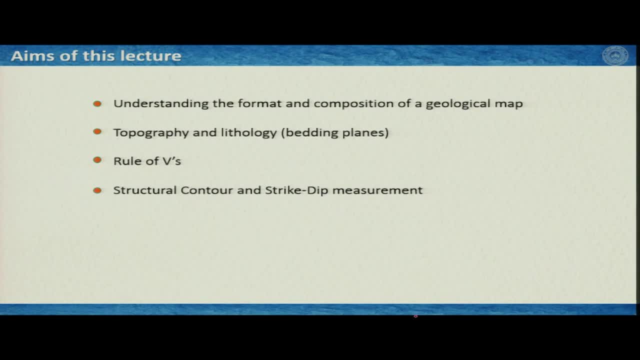 we will discover that there is something very interesting which is rule of V's. And finally we will. we will figure out that even if a bed or a feature is not exposed on the surface, that where you cannot measure, dip and strike, but you can have the line which is connecting. 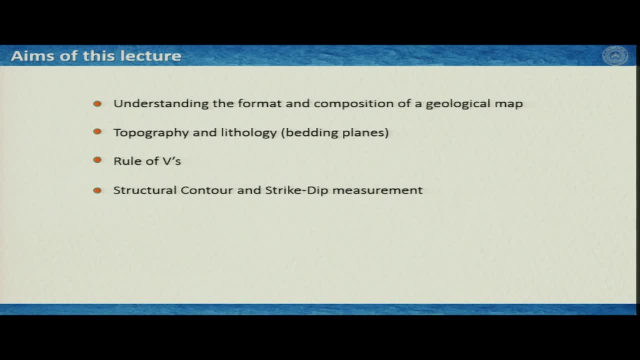 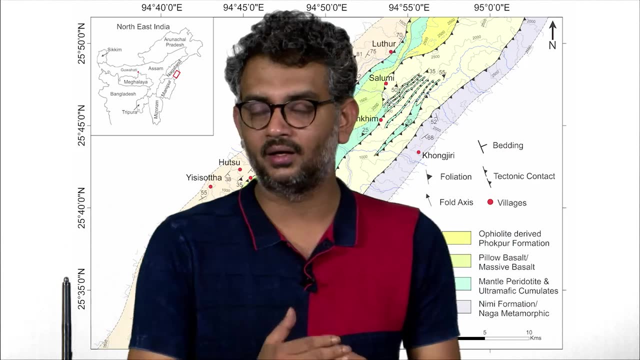 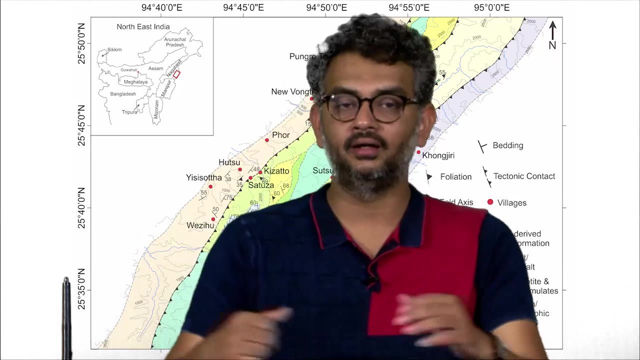 the two different lithologies on the surface of the earth, which is contoured, which is which has a topography, then how to calculate the strike and dip with the help of structural contour. So let us start with the very first idea, and the books I have suggested you at the very beginning of these lectures may not be very. 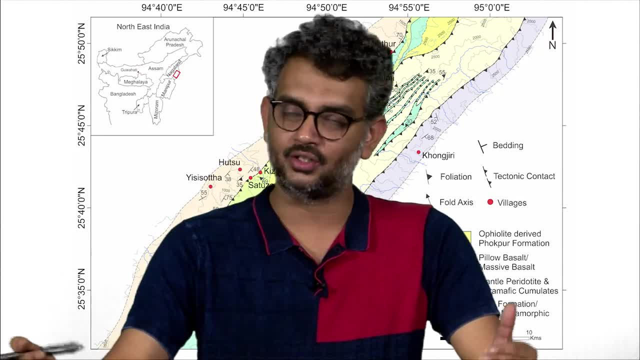 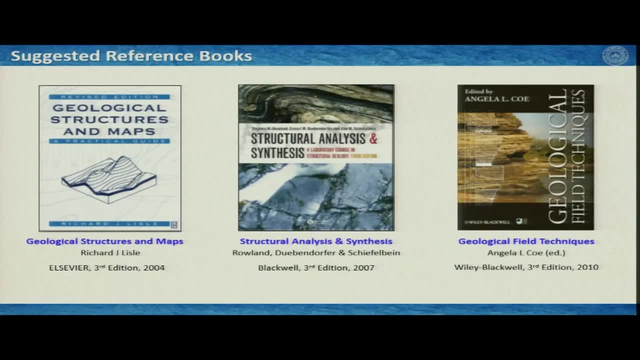 very helpful in understanding this lecture, or feature analysis related to structural maps and so on. So here are three books that I personally like, and I also would like to recommend these books for this particular class and also for your feature references. The first one is geological structures. 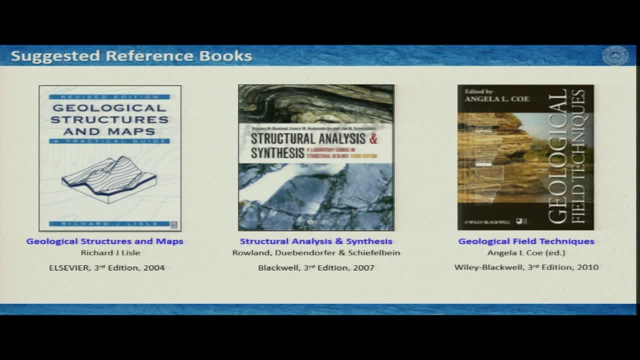 and maps written by Professor Richard Lyle. This is published from Elsevier, third edition, 2004.. The second book is Structural Analysis and Synthesis. It is written by Roland Etel, published in 2007 from Blackwell, And the third one is one of the latest ones. 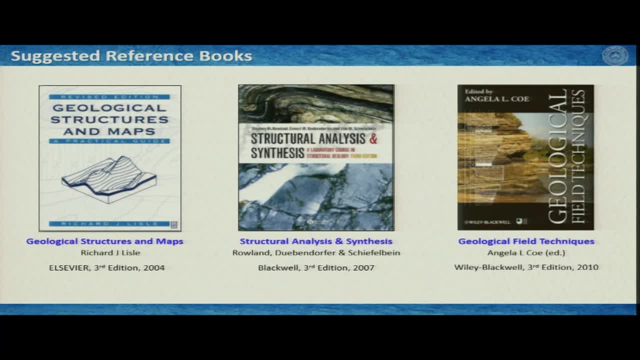 It talks about geological field techniques. Angela Coy edited this book along with four or three co-authors- I exactly do not remember, but this is published in 2010 and it is from Wiley and Blackwell Now. I personally would recommend the first book, a must to have if you would like to continue. 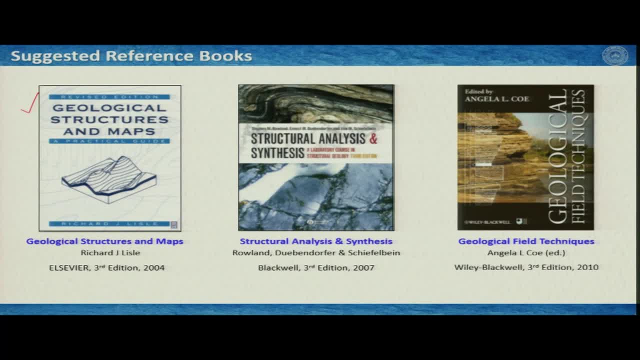 with geological mapping and, to be very specific, with the structural geology. The second and third book interestingly deal with many, many techniques that you should learn in the field. It gives you the very basic ideas: what is deep, what is strike, how to measure it, how. 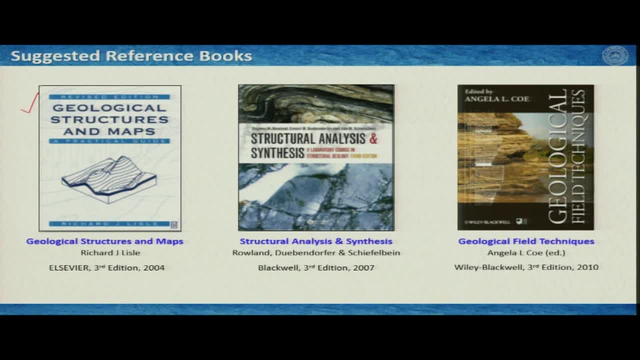 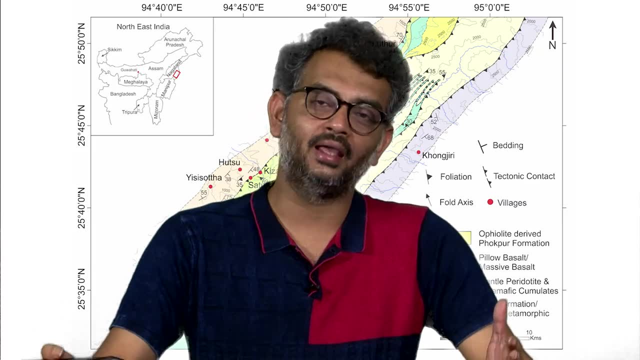 to hold the compass, how to take the reading, How to take the reading on the notebook, how to interpret them, how to construct things in the field directly, and so on. These are very handful, but again, these are not the scope of this lecture. 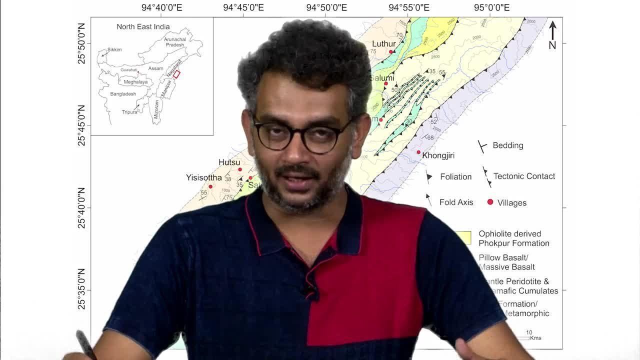 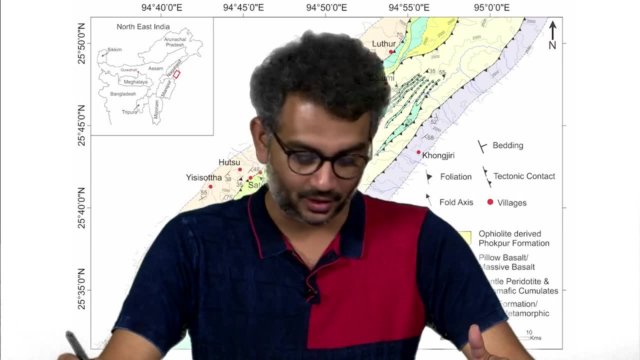 I hope in future I can come up with another course- I have to design it differently- on geological mapping and so on, particularly with the emphasis of structural elements. But these three books are very, very important and in this lecture, whatever I am going to, 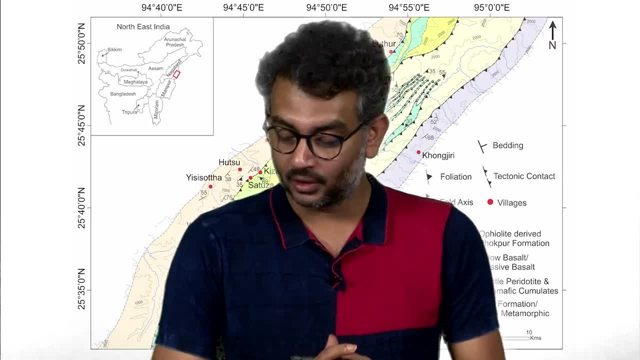 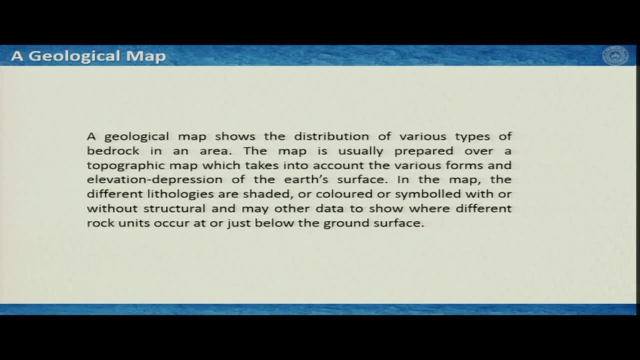 show you is mostly derived from the book, From the book of Professor Lyle, The illustrations and diagrams I have redrawn it, but it is essentially from his book. So what is a geological map? You know all this. what is? but this is how more or less you can define it: a geological 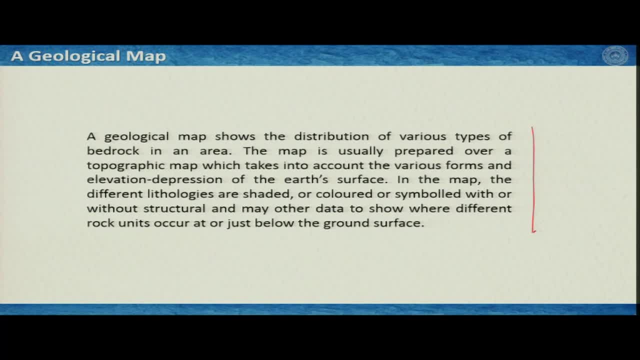 map or describe it in a way. you do not have to define everything. A geological map shows the distribution of various types of bedrock in an area. The map is usually prepared over a topographic map Which takes into account the various forms and elevation depression of the earth surface. 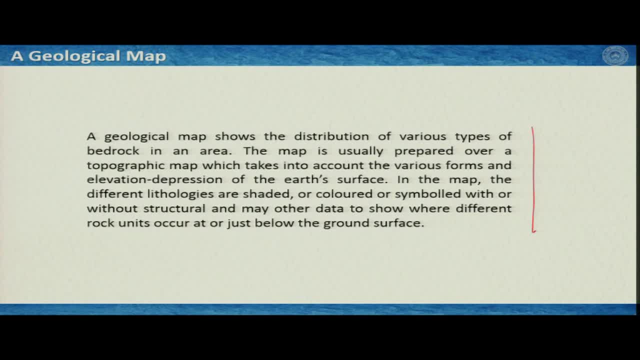 In the map, the different lithologies are generally shaded or colored or symboled, with or without structural data and may other data to show where different rock units occur at or just below the ground surface. So many things are written here. Let us let us take the highlights of 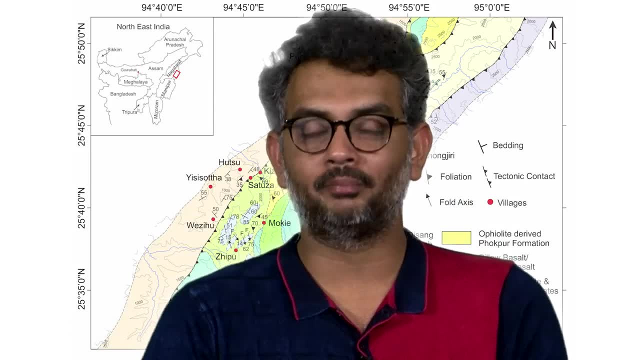 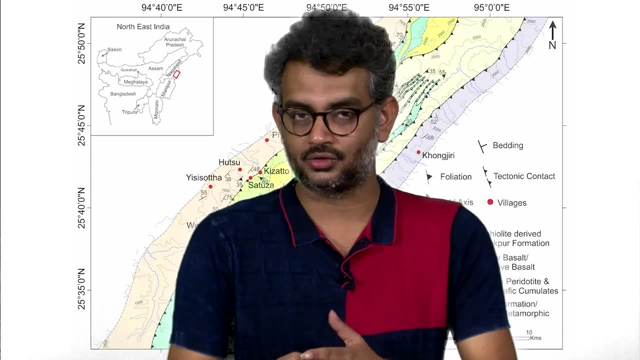 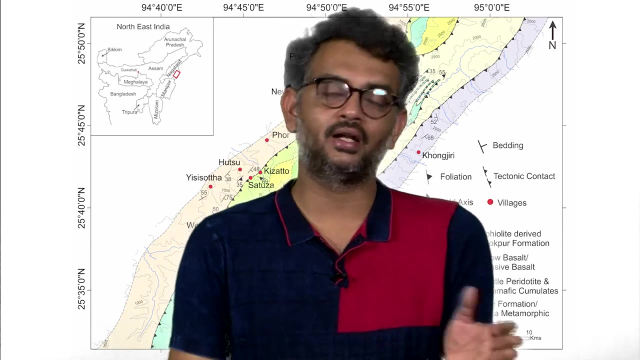 Of these statements. So, first of all, a geological map essentially gives you the surficial data, Maybe few meters or few tens of meters and so on. So what you see on the surface is essentially included in the geological map. Looking at a geological map, you may not conclude what is happening at 10 or 15 kilometers down. 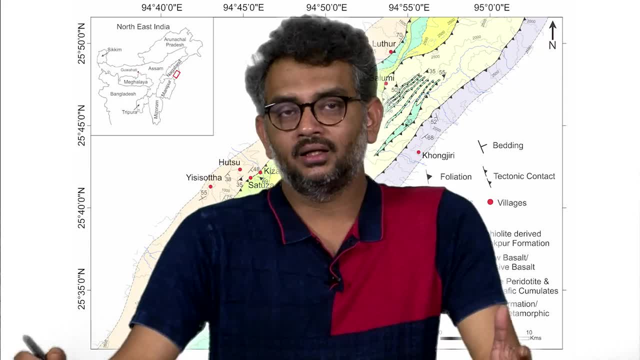 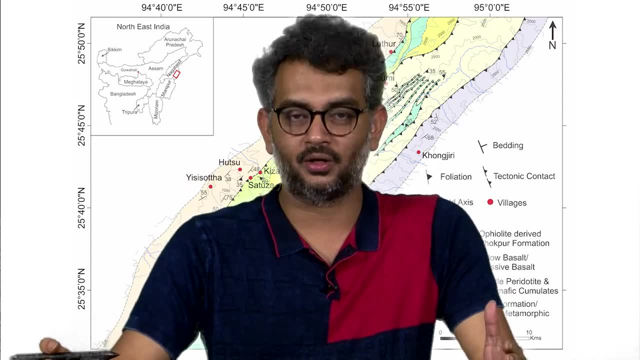 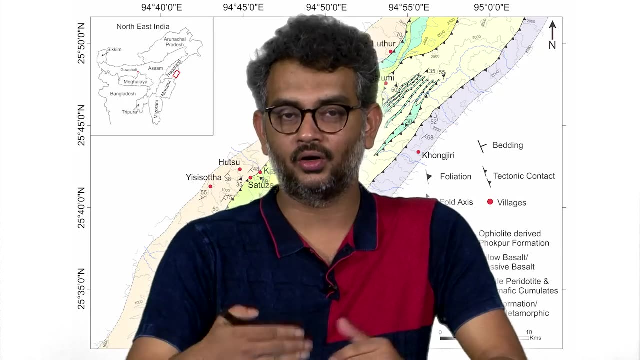 or even 1 kilometer down, it may be completely different. and then therefore, a geological map essentially represents The various features, various rock types that you see in the field and you compose them together with the different rock types that you have seen, their contacts and so on. 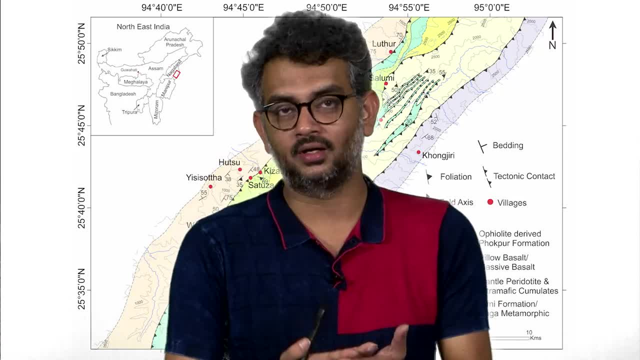 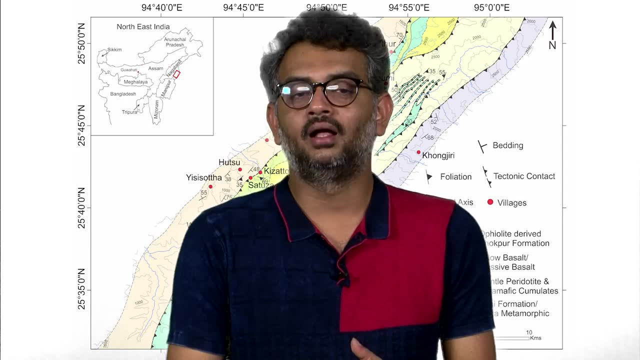 And generally the map. if it is very large scale map, it is done over a topographic map, which you can consider that this is a reference of your area and the topographic map is very, very useful. We have a couple of slides on topography. 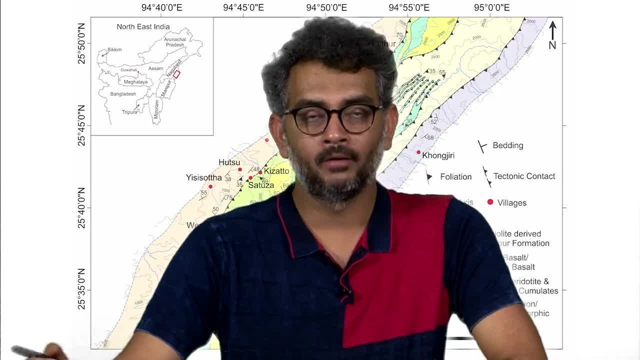 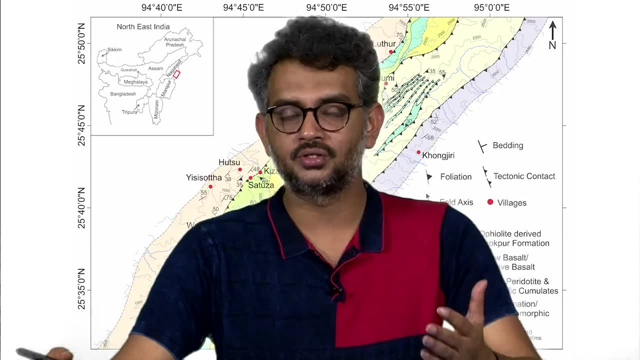 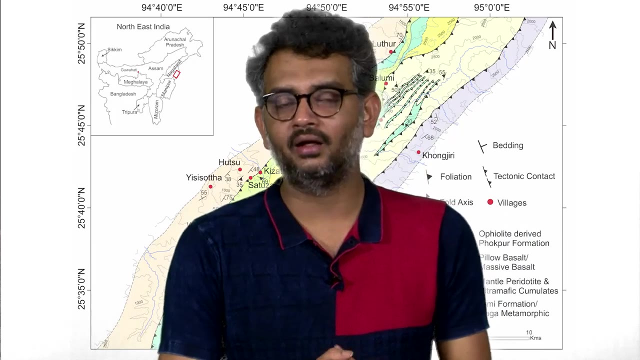 And it is a topographic map and its usefulness and so on. So generally large scale maps are drawn over topography, topographic maps. But you can also consider plain paper mapping and so on. If you have to do a very detail mapping in say a 10 meters by 10 meters area, then topographic. 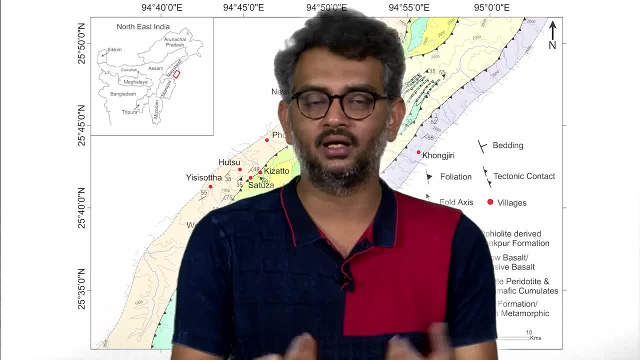 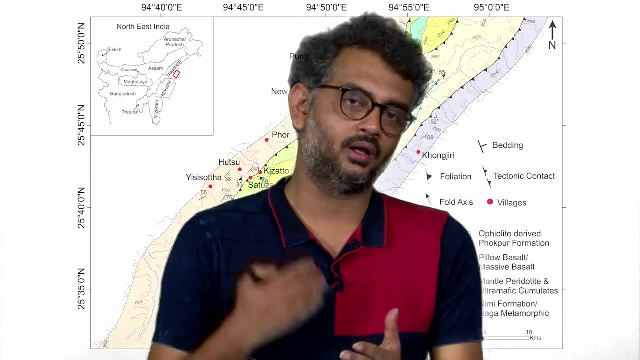 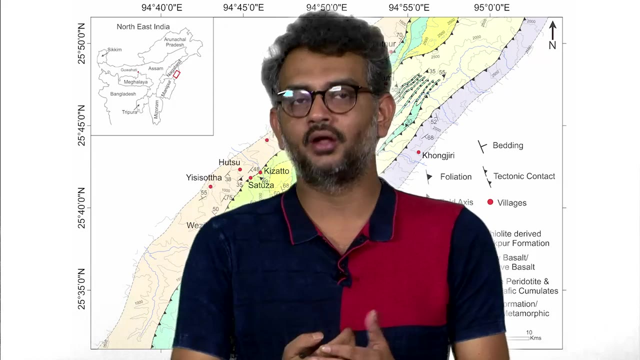 map is not that much useful because topographic maps are generally very large scale. again, these are different techniques, but there are large scale mapping and plain paper mapping. the mapping you need the help of topographic map, but in plain paper mapping, no, The primary thing in a geological map is mostly the lithological contacts and their disposition. 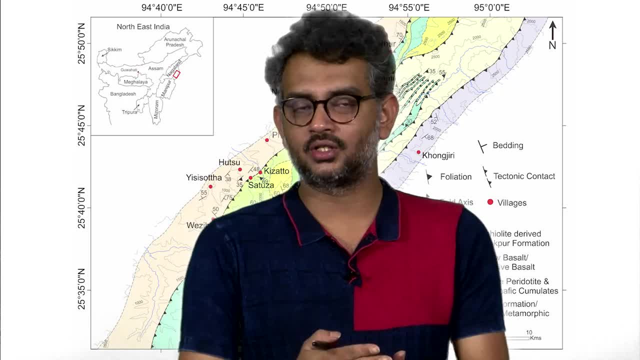 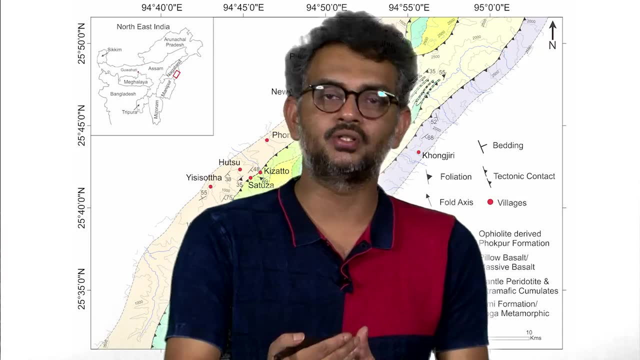 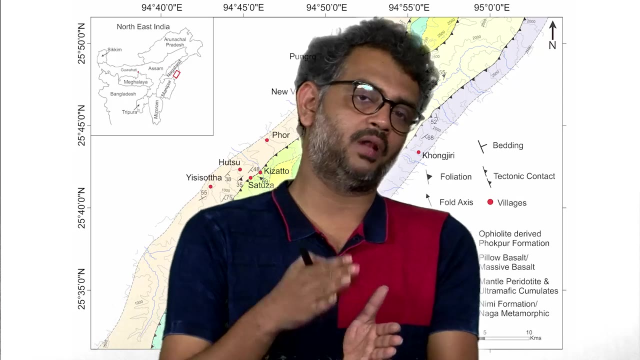 on the surface. but if, say, a lithological contact is faulted, then you can use some symbols and therefore you start introducing the structural elements on your map. or maybe you have series of lithologies, planar lithologies, and they are deep into a certain direction. 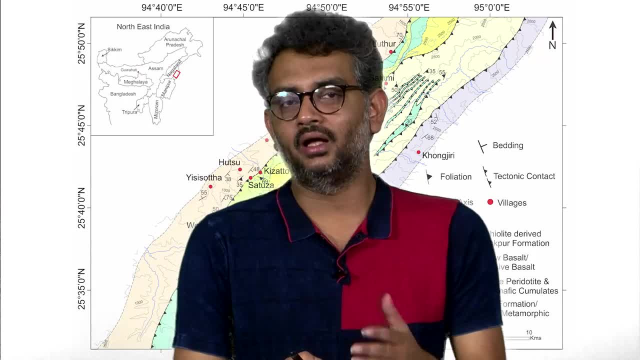 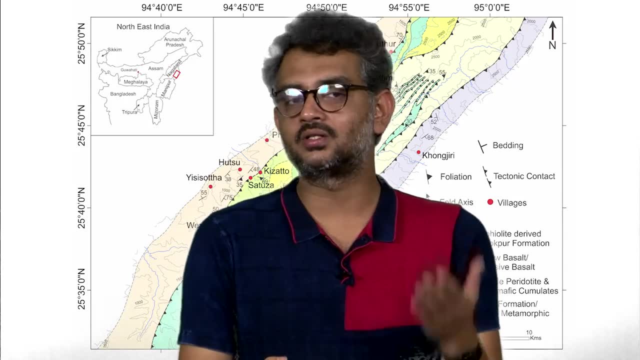 So you can include the strike and dip in the map and therefore you again introduce the different structural features. For example, you see that in the field this is a sin form, So you can use the symbol of sin form, you can use the symbol of anti form, and so on. 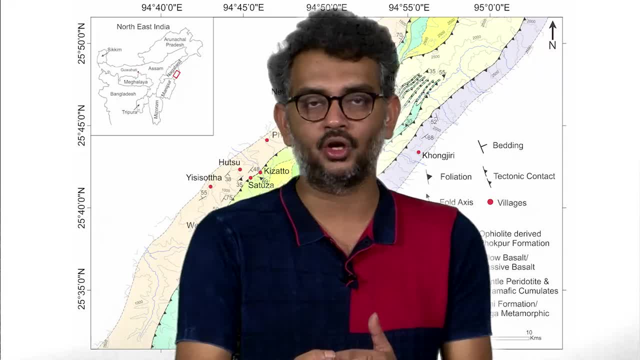 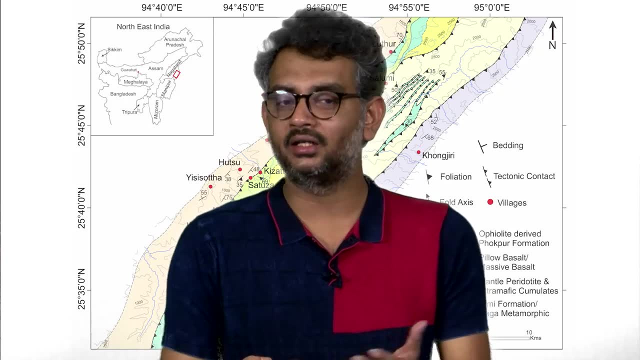 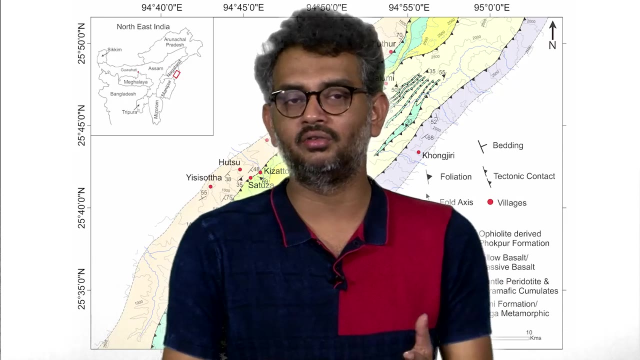 and by this you slowly add many, many, many information as much as you can, based on your need to the geological map People also add. So you can add many other features, say geophysical measurements, say you can add density. you can add many other features: conductivity in the corresponding to particular lithology. 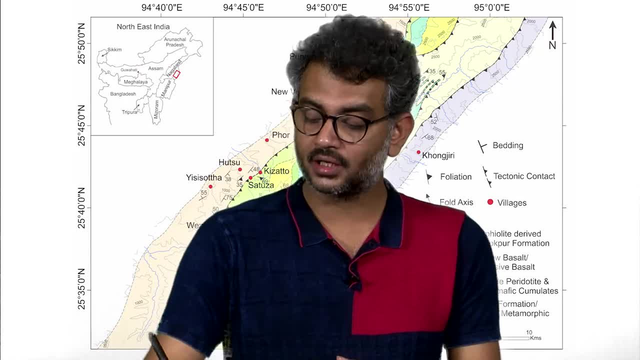 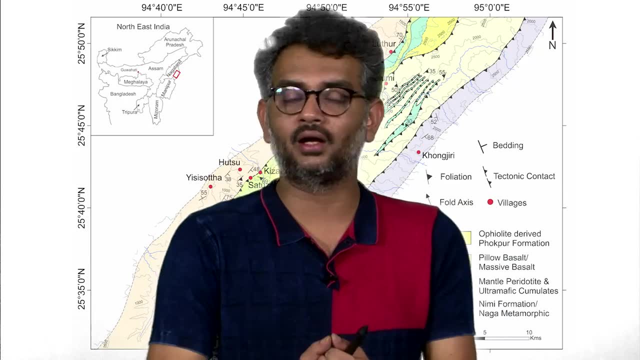 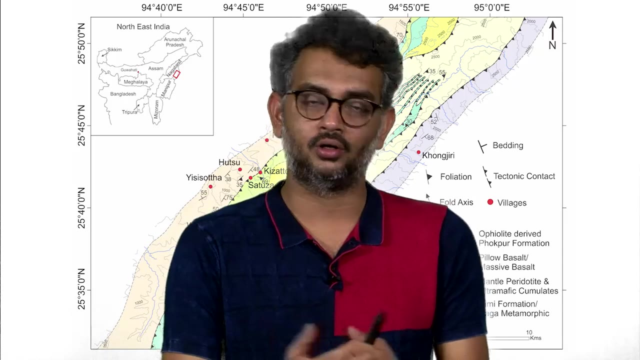 or particular feature of your map. So geological map is essentially very, very important, not only for geologists, not only for interpreting the structure or regional tectonics or know what is there, but it is essentially important also for engineers, for constructing dams or buildings or roads. 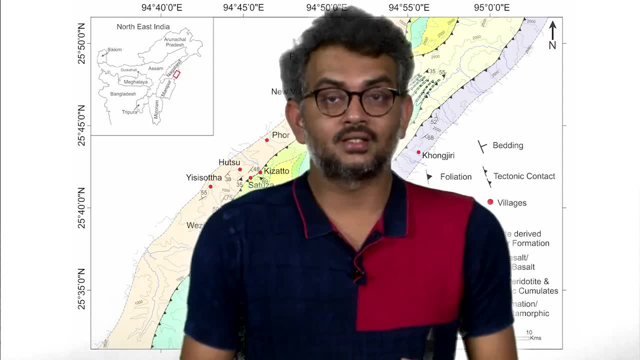 So, yes, this is very, very important. We have to learn how to read and how to interpret and how to prepare it. As a geologist, that is the primary job of us. So here is an example of a geological map. I took it from geological survey of India and this is what you see: the map of Sikkim. 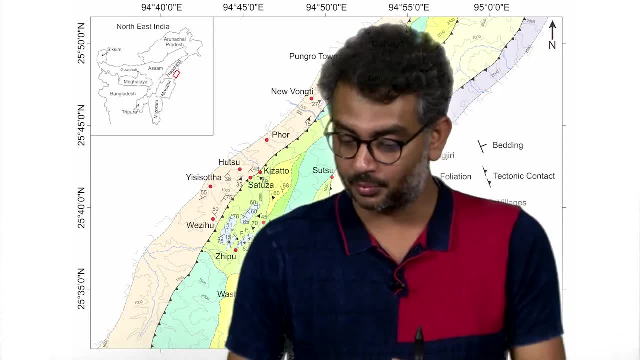 It is a state in the north eastern part of India, So the state is like this. this part is the whitish part that you see. these were snow covered and people could not figure out the lithology, So the state is like this. 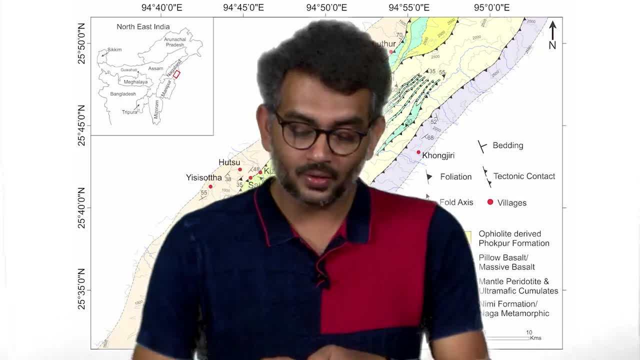 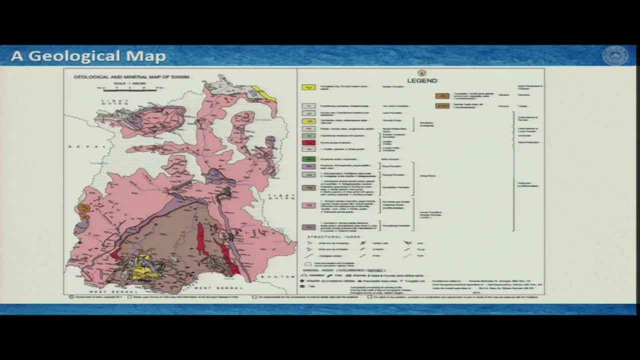 This part is the white ish part that you see. these were snow covered and people could not figure out the lithology. So this is what you see, This is the black lithology, and so on, but you see that this map shows very nicely. 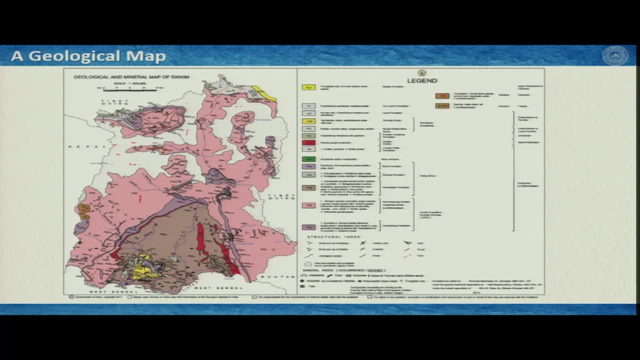 the different lithologies with different colors. So this pink has a different lithology, This purple has a different lithology, This red has a different lithology, This grey has a different lithology and they are disposed in a in a different way in the. 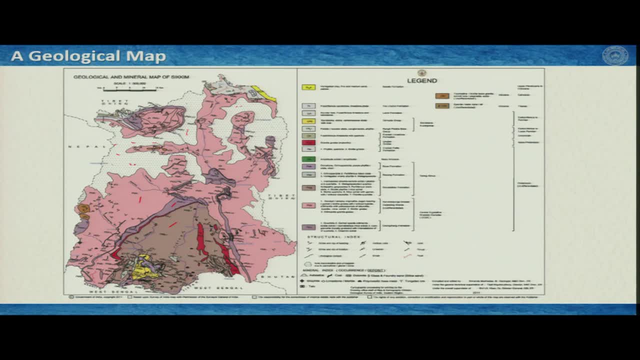 map and you can see many other maps. just type geological map and you will see many different features in this map. Also, you can see that here, these the structural details, the structural data are included there, the deep and strike are included here and so on. 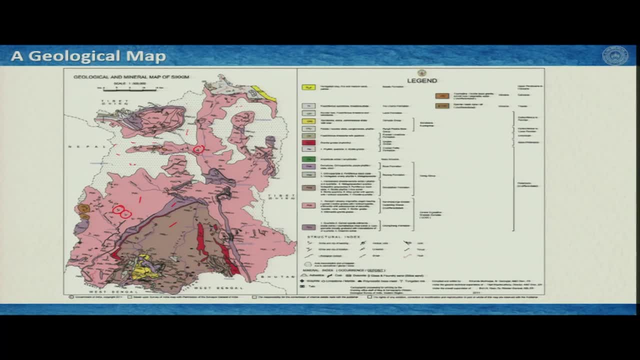 So this also tells you a very, very important information about this area, and a geological map essentially comes with something called legend, So you have to explain what are the different colors or what the different symbols are. you have to explain what are the different features that you are using, the line drawings and so on. these are also very important. and finally, 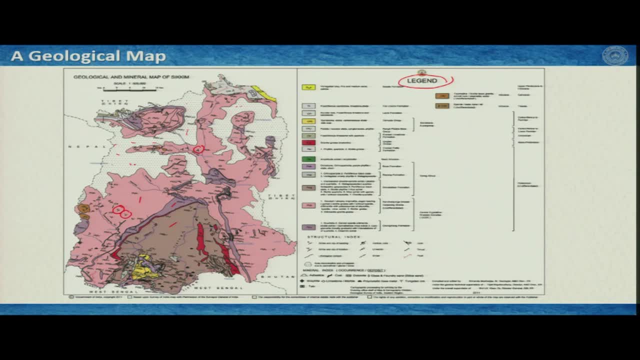 what is most important in any geological map is that you provide the scale. this is very important. we will learn about it that what scale? I am looking at that if I measure two centimeters in this map, that means how much I am measuring in the real scale. is it 100 meters, is it one kilometer or is 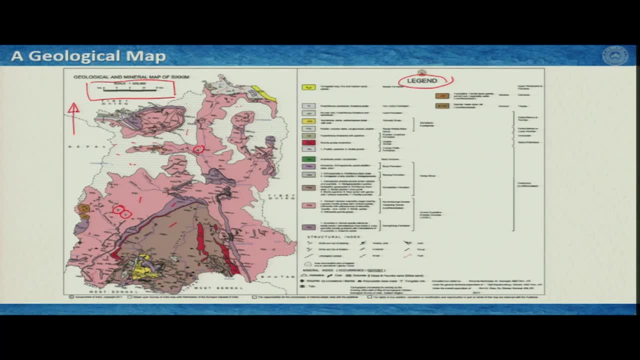 it four kilometers or even more, and this is also very important- that you indicate what is the direction of north. Sometimes people indicate the direction of north. at the same time they indicate also the latitudes and longitudes in the map. that also tells you where exactly in the earth you have mapped, or the map. 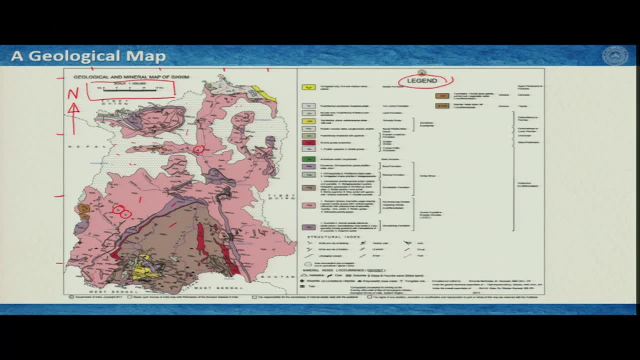 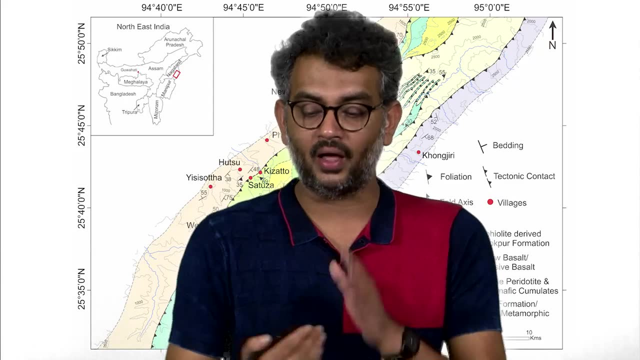 is located. So these are the very important aspects of this map, apart from the different colors indicating different lithologies, the different symbols of structural data and so on. you have to have a legend, you have to have scale in your map, you have to assign what is the north direction. 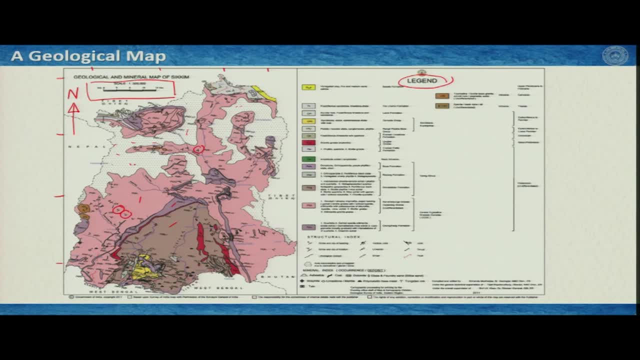 and if you have a legend, you have to have a scale in your map. you have to assign what is the north direction and, if possible, in the map you also, if it is a large scale map, you suggest what is the latitude and longitude your mapping area is. 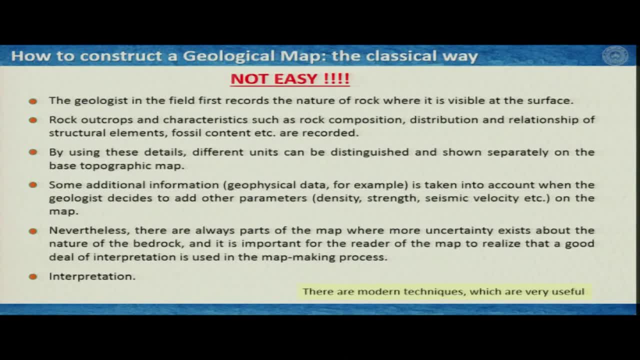 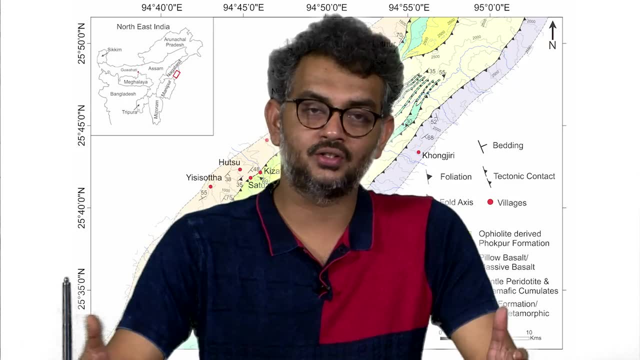 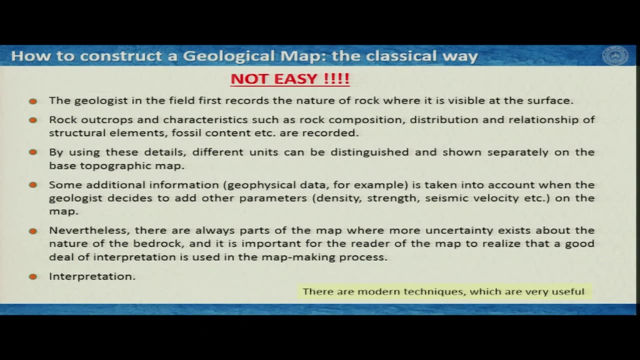 Now how this map is constructed. again, I am not going into the detail, but I tell you it is not a very easy task. So there are series of processes. geologist in the field first has to go and then he has to record the nature of rock where it is visible at the surface and it is not visible everywhere. that is quite common. 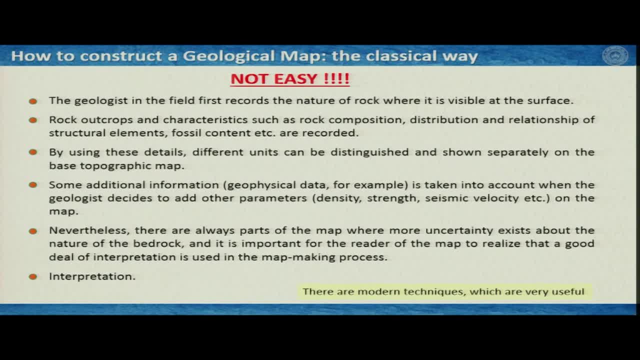 Then rock outcrops and characteristics such as rock composition, distribution and relationship of structural elements, fossil contents, etc. etc. The geologist do record in his notebook and so on, and nowadays may be in the mobile phone or laptop or with some digital mapping softwares. 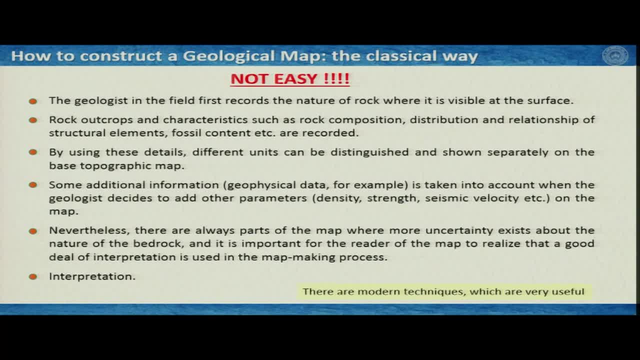 Now, using all these details, the geologist then distinguishes different units in the field that he or she has seen, and then he tries to plot them separately in the map or on the base of the topographic map. Now the geologist can include some additional information. for example, geophysical data is. 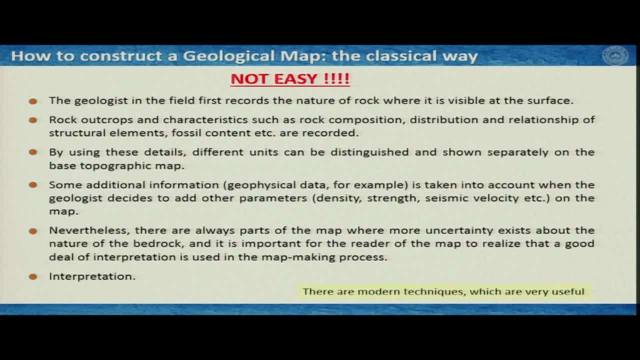 taken into account when the geologist decide to add other parameters like density, strength, seismic velocity and so on on the map. Nevertheless, there are always parts of the map where more uncertainty exists about the nature of the bedrock, and it is important for the reader of the map to realize that. 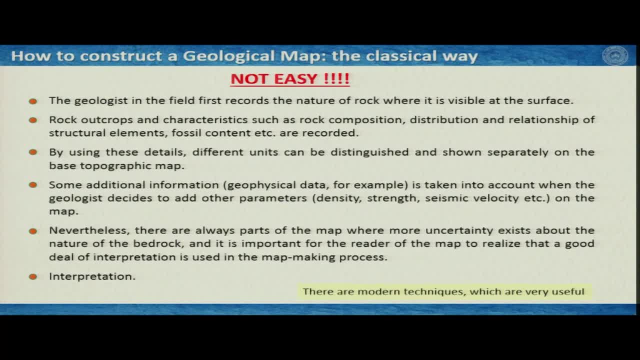 a good deal of interpretation is used In the map mapping processes. what I mean by this? that it comes actually from this place, that where it is visible. at the surface You do not see rocks everywhere, but you map it and then you use your intelligence to interpret. 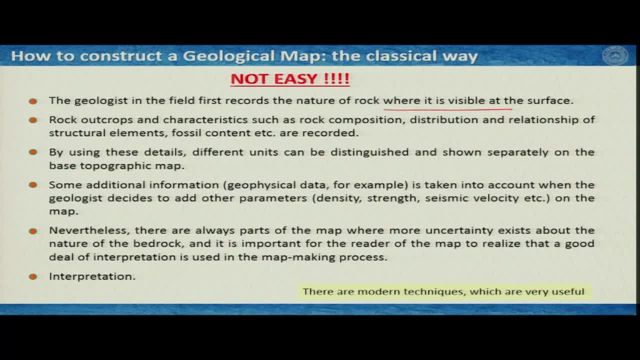 that if I see this rock here and if I see the same rock here, how they are connected may be your interpretation is wrong, but based on your experience, based on your intelligence, based on your theoretical background, you conclude: this is how it should be. someone can challenge. 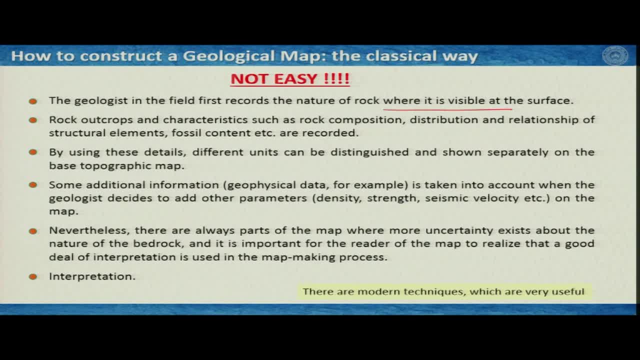 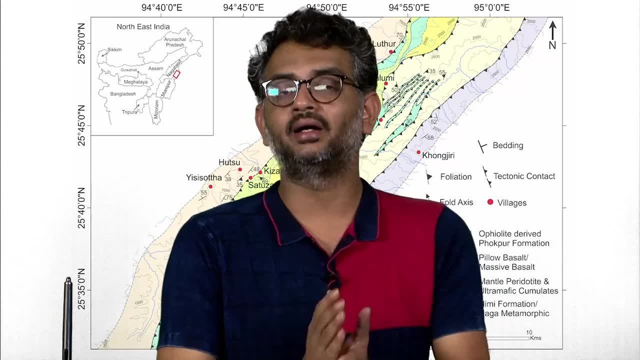 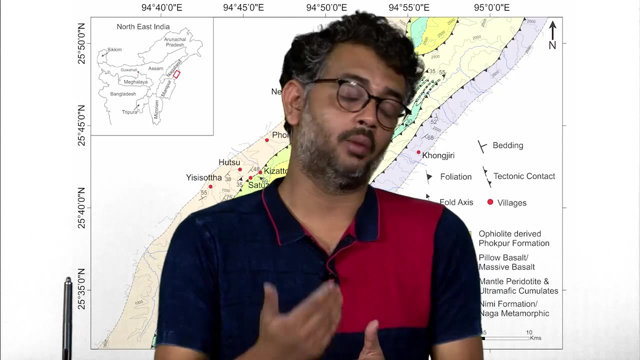 it, It will always work. But once you look at a geological map, you be sure that a lot of uncertainties are involved in this map. So do not take any map as granted, unless I mean particularly if it is really required for some very special job. 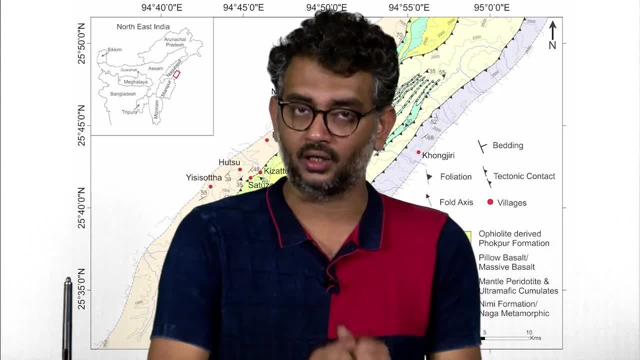 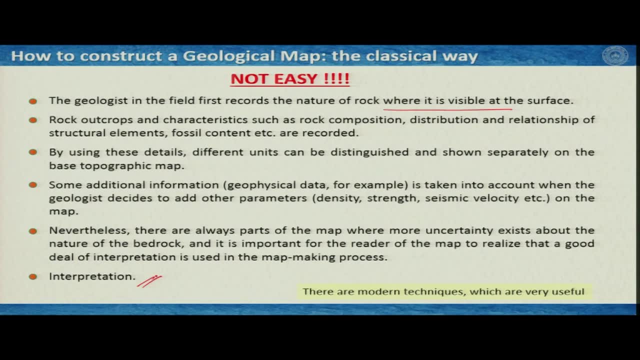 So better you go to the field, match it that, yes, this is what is happening, otherwise you take it if it is from a good source. And final part is, of course, the interpretation That what is happening That once you have a geological map, this is a job done, but after the map is ready, 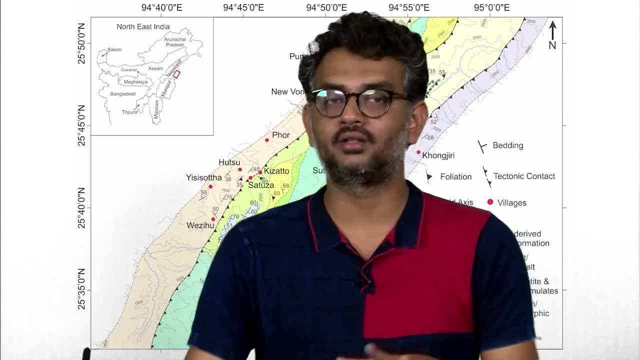 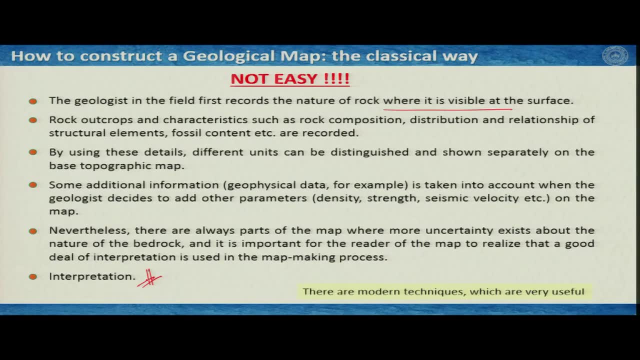 Then it is very important that you interpret the structure, you interpret the feature, you interpret the lithology and so on, but this is something else that you would learn in a different class or different lectures. So, as I was talking about, there are many modern techniques which are very, very useful, but 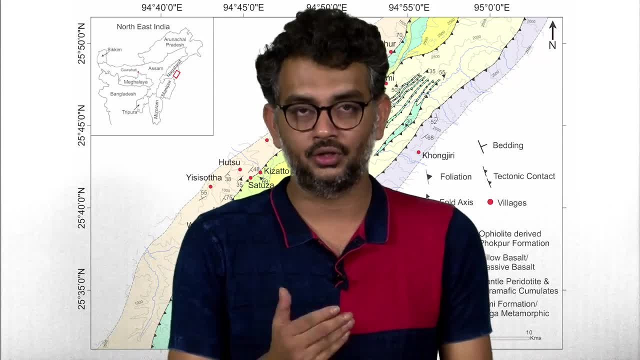 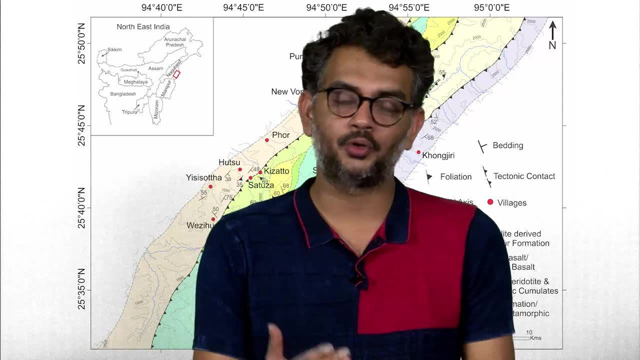 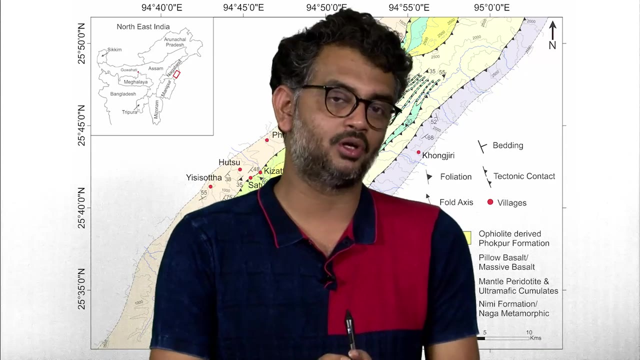 it is also important: as a student, you go to the field with your field instructor, with your teacher, learn how to hold a compass, learn how to take back bearing, learn how to take front bearing. you take your steps with a measuring tape and then do different techniques, because 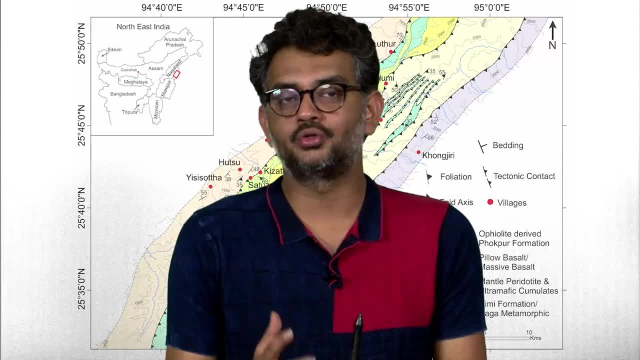 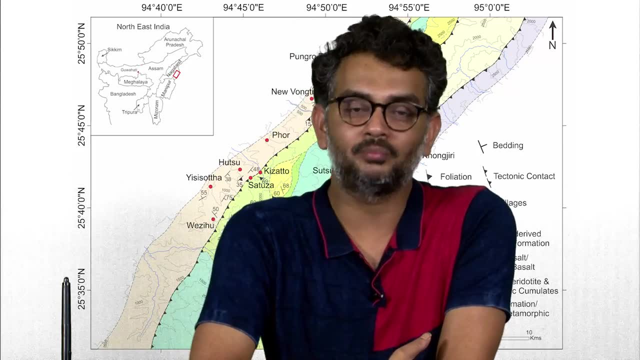 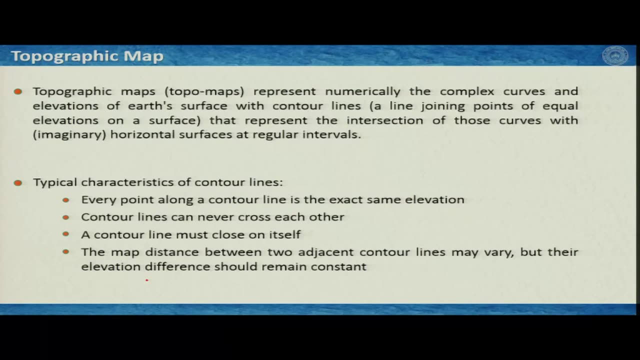 not always, not everywhere you can use all these modern techniques. So let us talk about the topographic map for a while. you know that what is a topo map? we generally call it topo map or topo sheet. So a topographic maps represent numerically the complex curves and elevations of earth's. 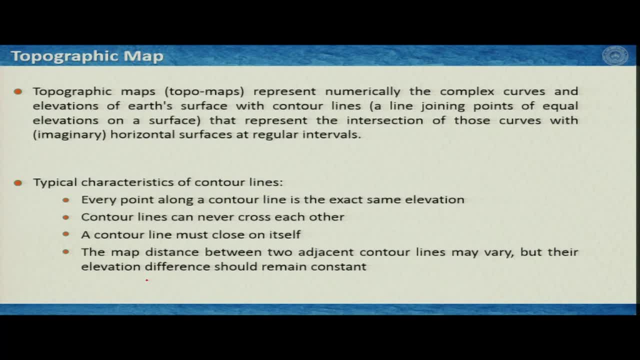 surface with the contour lines. Now, a contour line is a line joining the points of equal elevation on a surface and the contour lines represent the intersection of those curves with imaginary horizontal surfaces. at regular intervals We will see topographic map and other things with some good illustrations later. but a contour. 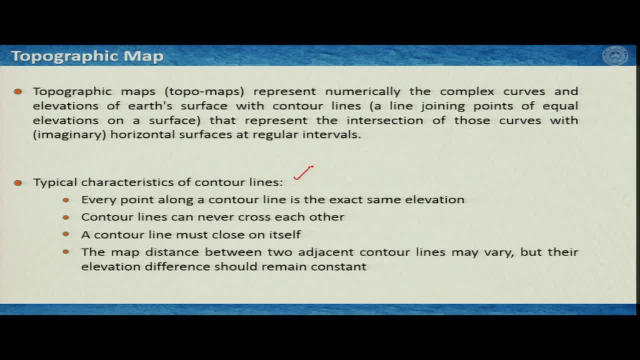 line or a series of contour lines should have some very special characters. because the contour lines indicate equal elevation on a surface. every point along a contour line is the exact same elevation. Contour lines, therefore, can never cross each other. so if you see a contour map going like 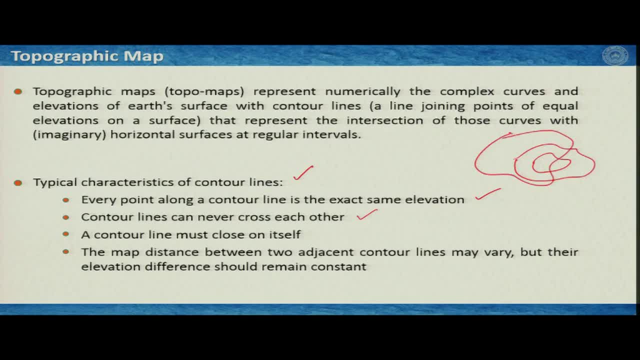 this going like that and then another contour maps like this, then this is something very, very strange and you discard the map immediately. So this is not something you should look at. A contour line must close on itself, so that is also something that you need to see. maybe it is not closing in your map area, but it has to close somewhere, and the lowest closing point is, of course, the sea level. we will see that. 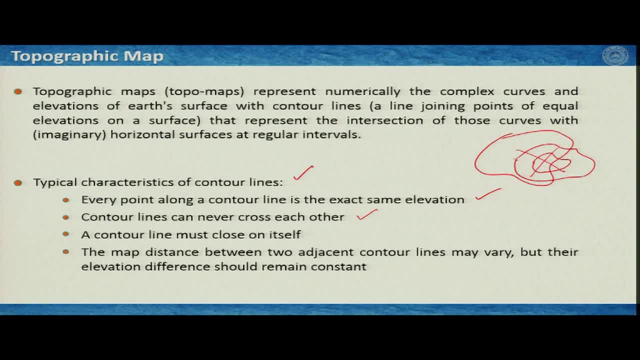 The map. distance between two adjacent contour lines may vary, but their elevation difference should remain constant. what I mean by that? let us say you have a contour line going like this and you write this is, say 80 meters. then you have the next contour line, something like that: this is 70 meters and this is you are seeing on a map. say this is you have a scale for that? 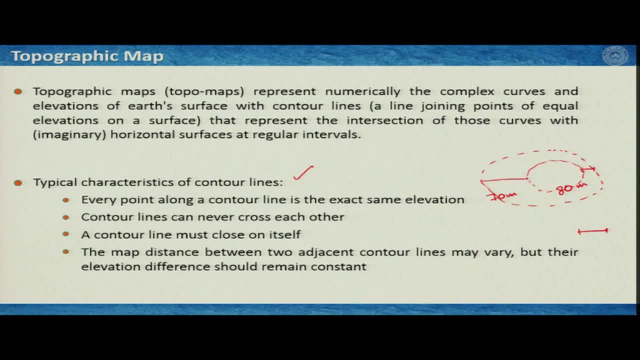 So in the map Scale this distance and this distance is essentially different, but the change of elevation from here to here is 10 meters and here to here is as well 10 meters. so does not matter how far the contour lines are, but two adjacent contour lines always should represent a very similar elevation, and that gives you an another idea. when the two adjacent contour lines are closely spaced, that means: 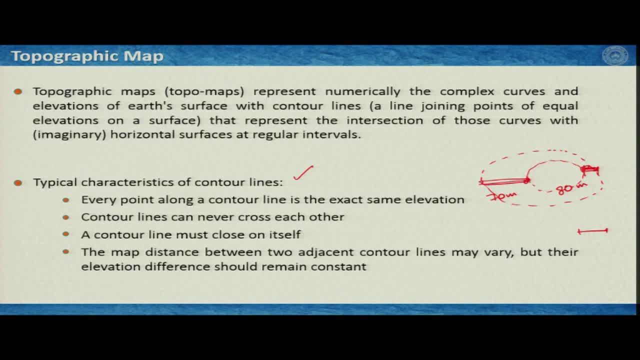 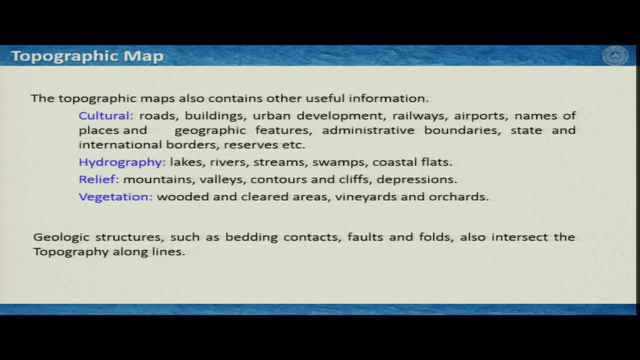 This Is steeper compared to when they are spaced far from each other. that means they have a gentle slope. we will see this soon. so the use of topographic map is very significant, and topographic map also do contain significant information. it tells you about the roads, buildings, urban development, railways, airports, names of the places and geological features. geographical features, then administrative boundaries, state and international boundaries. 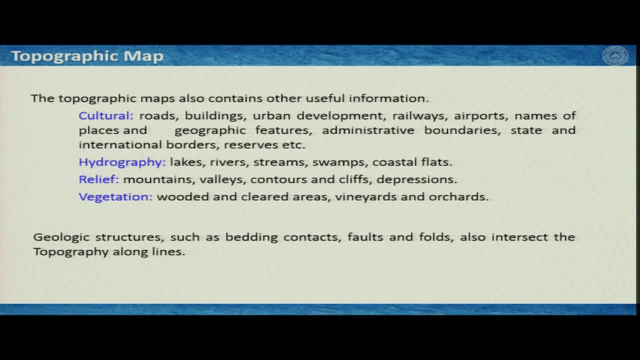 Reserves and so on. It also tells you about what her body is of the cereal, like per真的是 streams, some systems, a coastal last upset. I should write it in a conceals you, because it is a topographic map of what the relief of this revision say: mountains, Valley's contours and, please, depressions. Mac done so on it only so tells you about the vegetation of the area of so weather missile. he is a younger Marian, he's a for us. 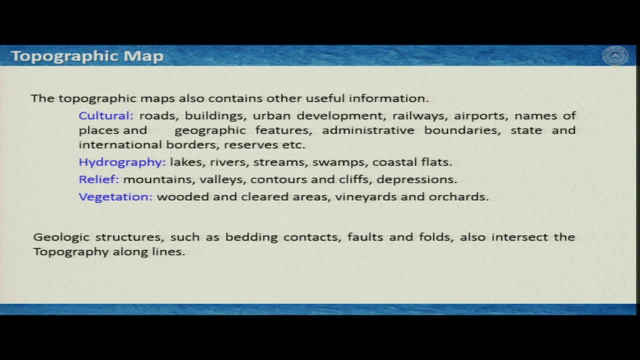 Gravel and orchard and so on. Okay, And so on to the area I mean In terms ofidade, Will able to live, Abolishing life With mycketworld nights, all these things, all these information you get from topographic map. 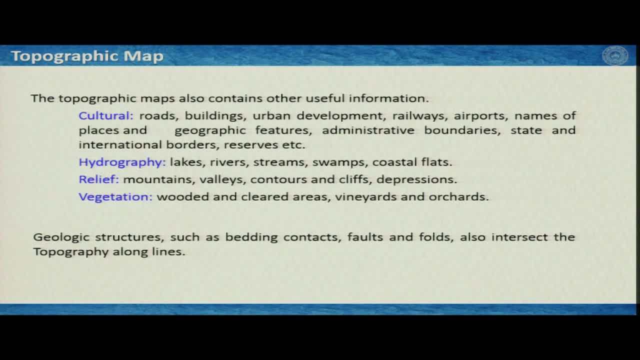 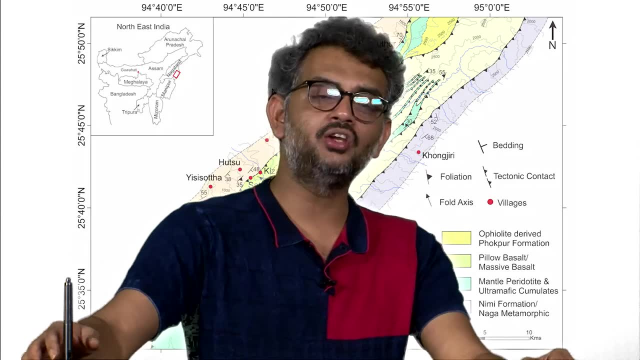 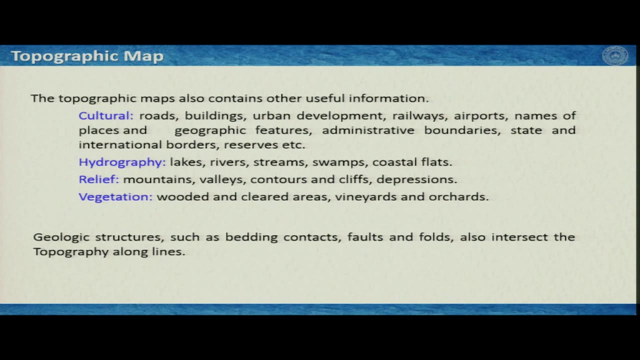 So a topographic map? it is not necessarily we geologists use. it is used in every community, particularly those who deal with the nature. In addition to that, geological structures such as bedding, contacts, faults and folds also do interact and intersect the topography along some lines, and this is exactly what 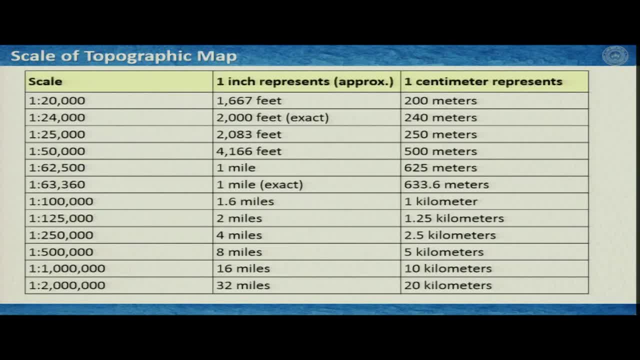 we are going to learn in this lecture after a while. So topographic maps generally come with different scales and the scales are given generally in this form that what topographic map you have, and I said 1 to 50000,. what does it mean? 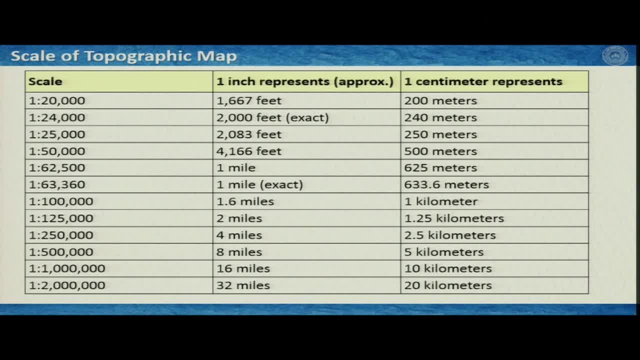 It means that 500 meters is equal to 1 centimeter. so this is: how is it given? So if I tell that I have a map of 1 to 50000, that means in the map if I measure 1 centimeter. 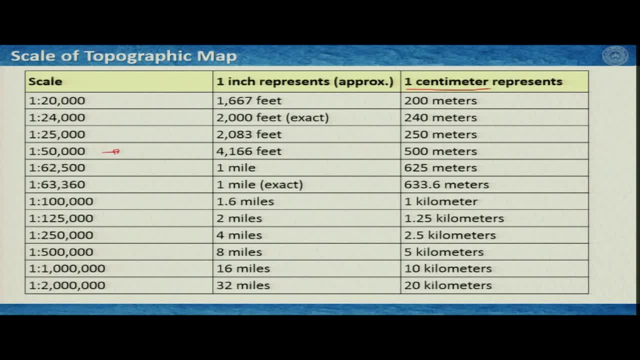 by my scale or ruler, that distance represents 500 meters in the actual area. So similarly you can have 1 to 20000, that means 200 meters. 1 to 24000, that means 240 meters, and so on, and then finally 1 to 20000 ratio, that means 1 centimeter in the map is. 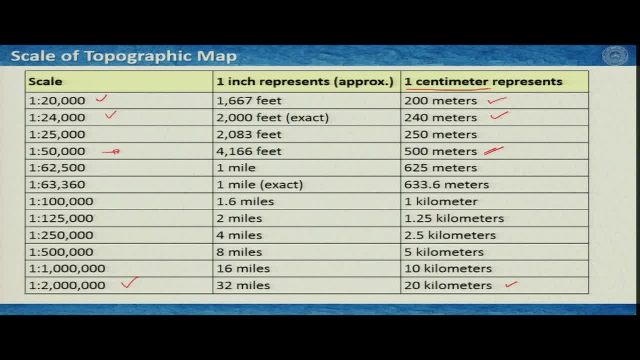 equivalent to 20 kilometers in the region. So this column represents these things, These things in centimeters or meter scale, and here it is inch and mile scale. So, very similarly, 20 kilometers in 1 to 20000 map scaled map. it should be 1 inch in the map. 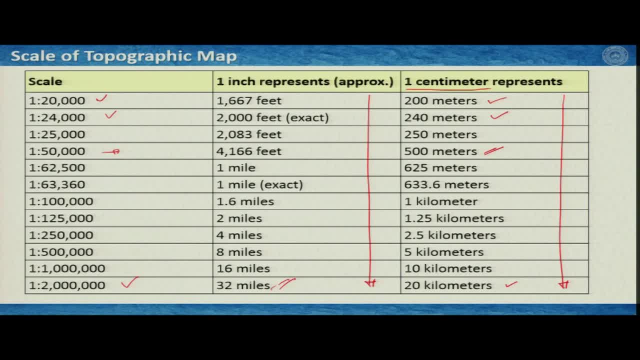 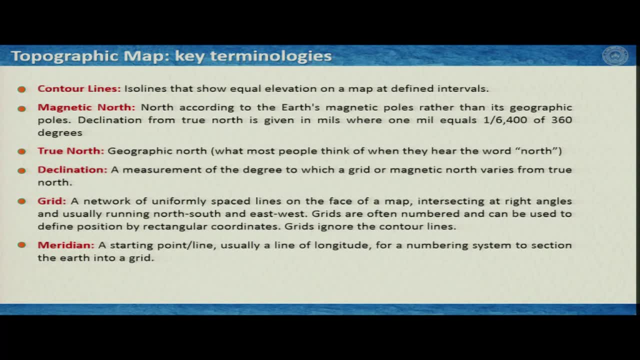 if you can measure, that represents about 32 miles in the actual area. There are some terminologies that involves in the topographic map, So we learnt few of them, but let us have a look in this list. So, contour lines: contour lines are iso lines that show equal elevation. 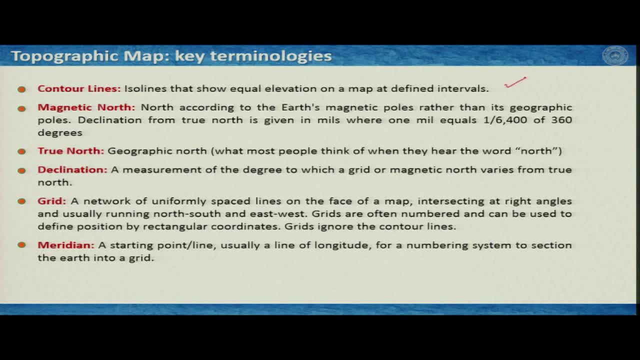 Elevation on a map at defined intervals. this we have learnt. Then magnetic north not according to the earths magnetic poles rather than its geographic poles. Therefore, if you have magnetic pole, then you must have a declination. So declination from the true north is given in mils, where 1 mil is equal to 1 divided. 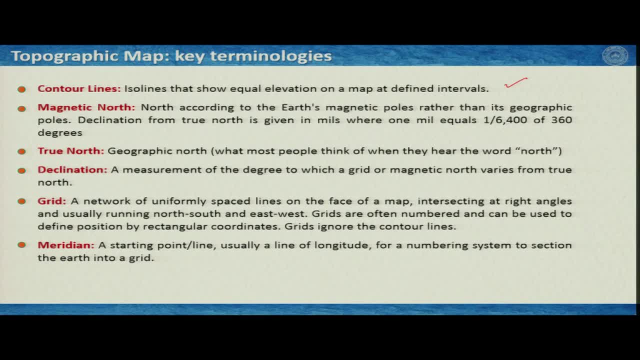 by 6400 of 360 degrees. The true north is the geographic north, And this is what we all understand when we talk about north Declination. we have learnt So a measurement of the degree to which a grid or magnetic north varies from the true. 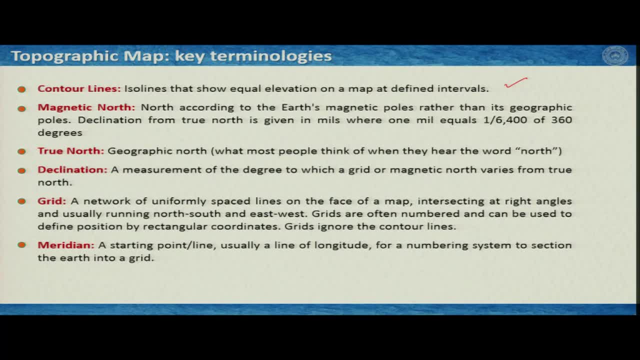 north, Then grid is a network of uniformly spaced lines on the face of a map, intersecting at right angles and usually running north, south and east west. Grids are often numbered and can be used to define position by rectangular lines, So this is what we all understand when we talk about north. 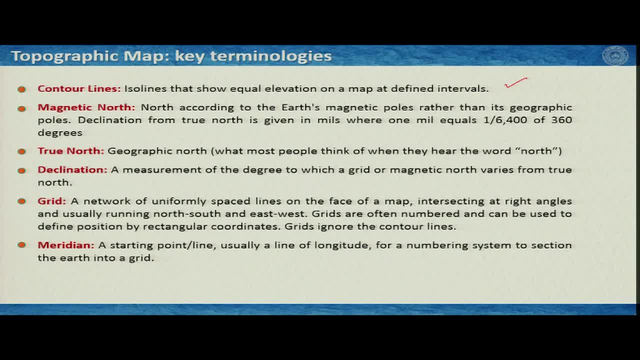 The grid is generally a network of the three rectangular coordinates And grids generally does not care about the contour lines, So does not matter how steep the slope is or how gentle the slope is, or whether it is flat or not. grids ignore everything and generally run either north, south or east, west, or if 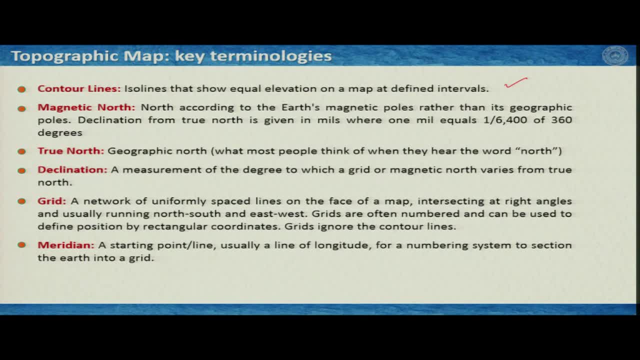 you have defined them in a different way. And then you have meridian. Meridian is a starting point or line, usually a line of longitude for a numbering system, So keep the numbers continued to the section of the map. If the number is continuous, it is considered to be a line of longitude. 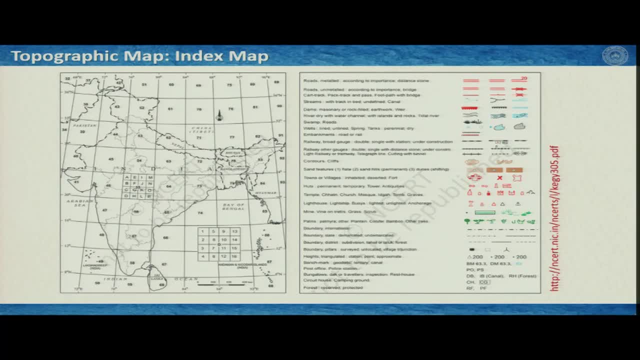 of the R into a grid. Now this is how the topographic maps are indexed. So this is our India. So India is generally gridded with these numbers. For example, we can have this 45 here, or 63 and so on. Then this is a single grid. Now, within this grid, you actually divide this. 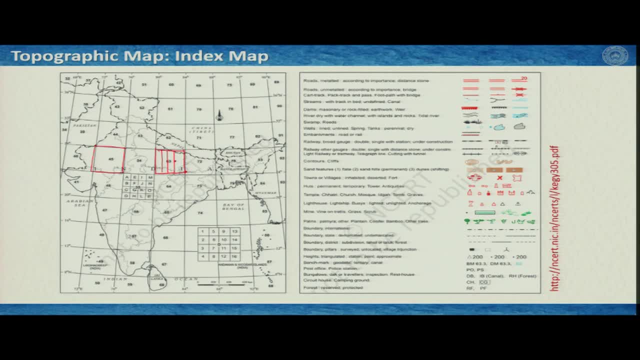 grid in 16 subgrids, and then you define them as it is written here: A, B, C, D, E, F, G, H, up to P, and then each of these grids- A for example- here it is given here- then again you subdivide it by: 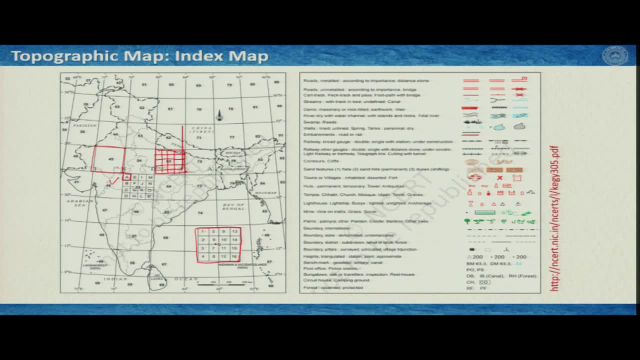 16 grids and then you again number them: 1,, 2,, 3,, 4,, 5,, 6,, 7,, 8 and so on. So this process continues. So, for example, if I want map of D here, then I have to say that I need 55 D, and if you need a map of 55 D3, that means 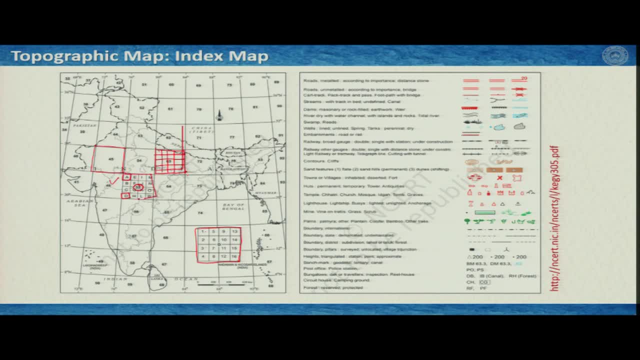 you have this grid 55, then you have this D, and then D is divided again in 16 segments and then you are looking for something here. So more numbers and alphabets, you add to your topo map more, So have a higher resolution. you go with the mapping process and the topo map as well. 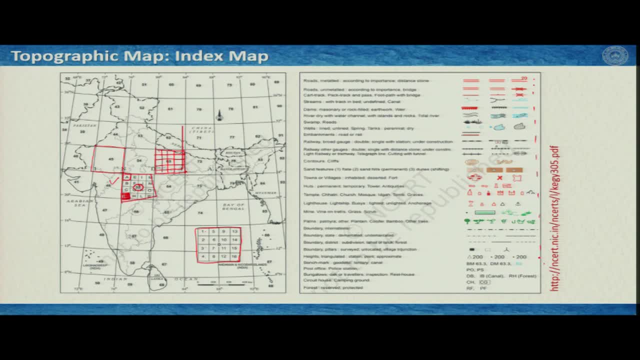 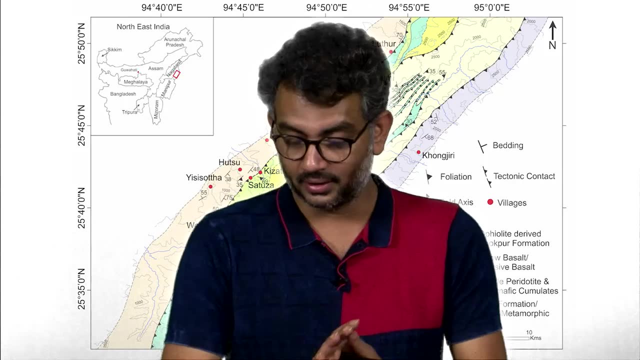 has legends. so these are the different things that you see in the topographic maps. So it is important when you look at it for the first time, you actually read this and see what is what. that is also important. So the that once you read it will you will remember So. 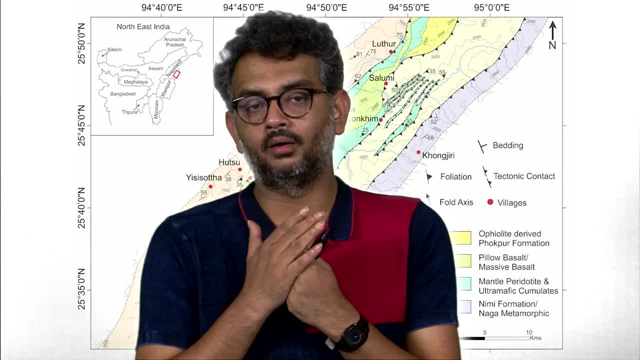 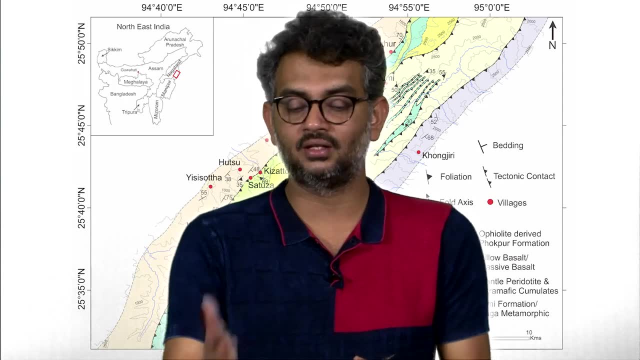 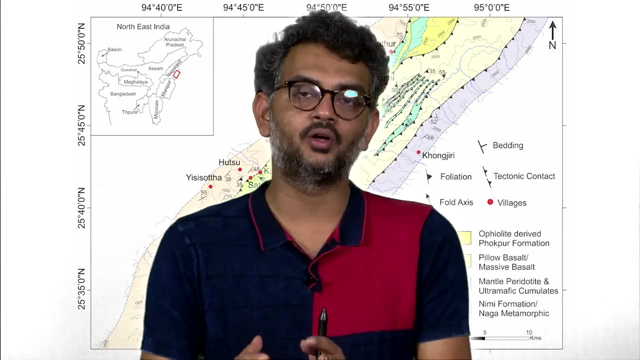 you do not have to look back every time, unless you forget, but it is important. once you read a map, you see what it is. this legend is attached. maybe you scan something or you crop something, and then the scanner thought that okay, legends are not important, So he cut it out or cropped it out and you 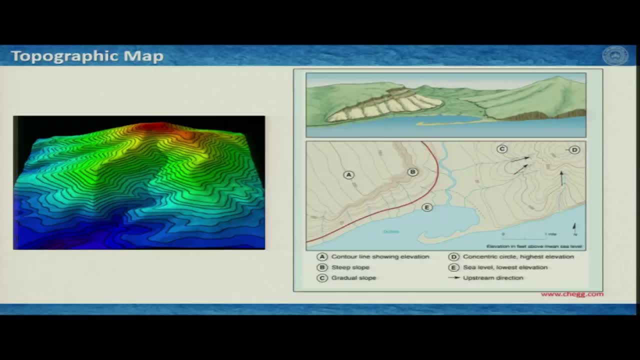 do not have it, So it is better you remember what is what. Now, this is how a topographic map looks like. So this is something digitally constructed. So you see the colors are varying. So the highest elevation is marked by red and slowly. 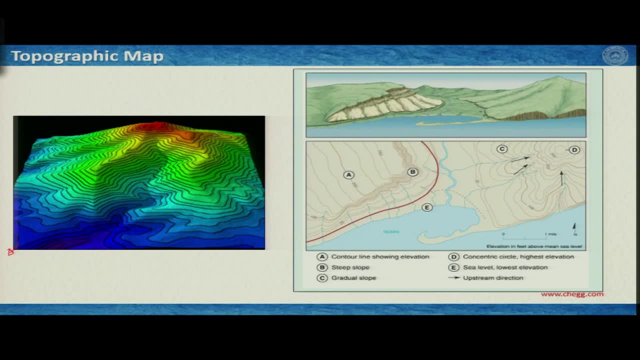 it is going to the cooler colors, to the blue, and you see that these black lines, these are actually making your equal elevations in this region. but this image here is representing in a much better way. So what we see here, we have a valley, a river is flowing through. 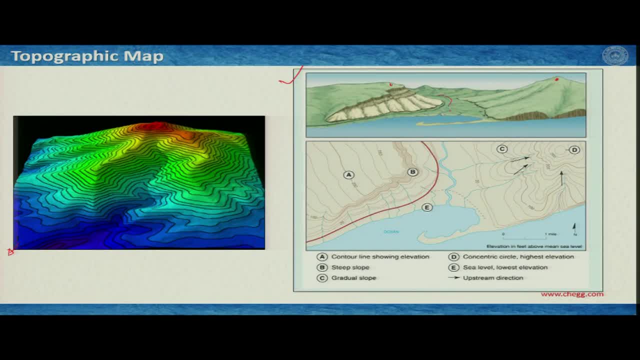 this valley and we have two little elevations here. We also see that in this elevation the slope is going down here. the slope is going down here, it is going down this side. this is one of the maximum elevations we see. We also see that slope is here very gentle here. 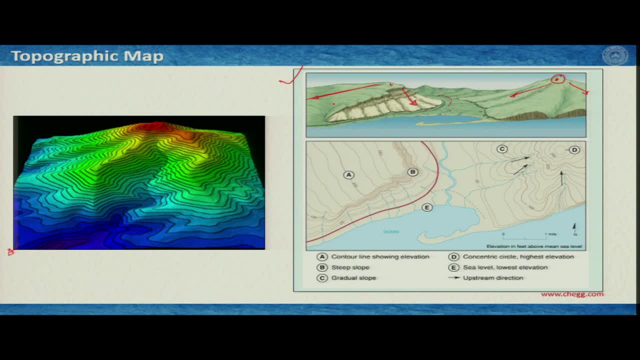 the slope is extremely high. We also see some little rivers or whatever channels are flowing along this, valleys and so on, and this is where you have the sea, and on the sea you have also some cliffs where the slope is almost perpendicular. Now, if I have to represent in the topographic map, then it looks like this. So here you. 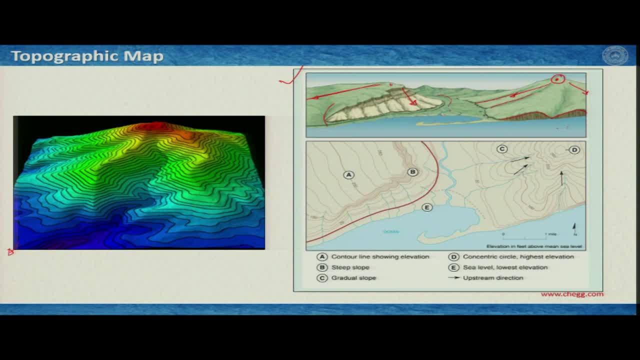 see that it is contours Contoured and by this you can actually figure out- though it is a map view, but you can figure out towards which direction the slope is changing. For example, this is 260,, this is 200,, this is 100.. So you can clearly figure out that this is how the slope is decreasing and once 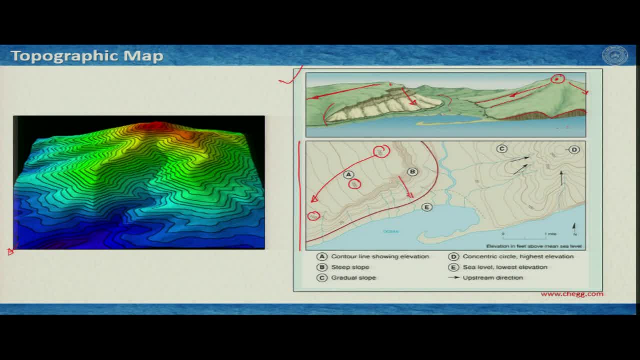 you know that, then you can also figure out that this is how it is decreasing here. but here you see, the spacing is much, much higher compared to the spacing here. So this is a steep slope. So that is the the trajectory here, and this is exactly what we have seen here Now. this 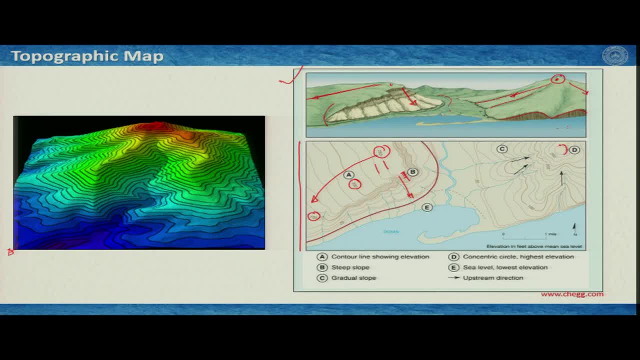 yes, the river is flowing and we also see that here we have the highest elevation and at highest elevation, if you see a concentric circle, that is the highest elevation of this region and that must be closed by a circle, and then the other contours should follow. 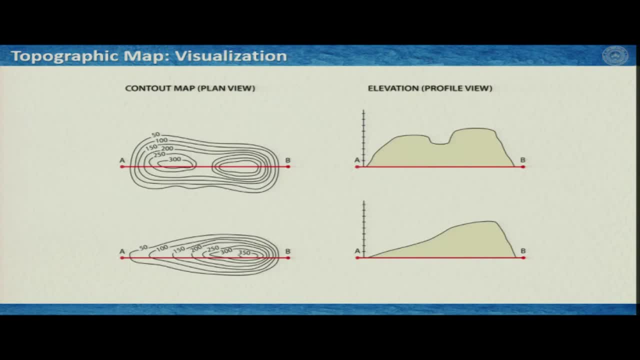 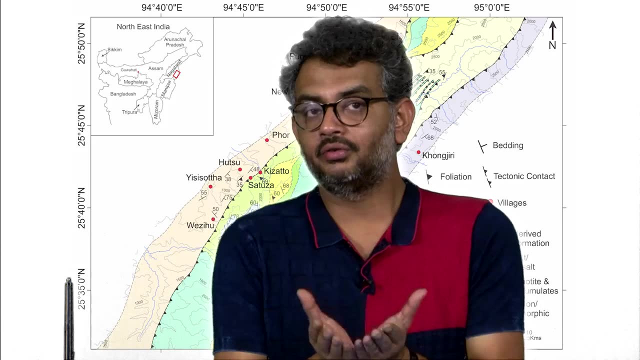 it in different ways, but this is how it is Now. it is also important that you train your eyes, So when you look at topographic map, you try to visualize Indonesia. 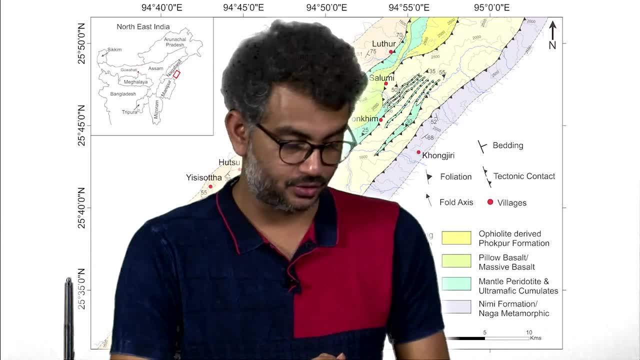 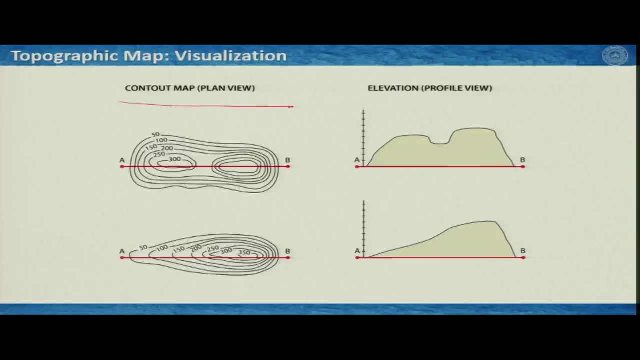 that, what is the elevation of that region? So I have given four examples here, So two are in this slide. So the first column is the outcrop map or plan view and you see here, from 50- that is the lowest elevation in meters- to 300 it is going. So 300 is the highest. 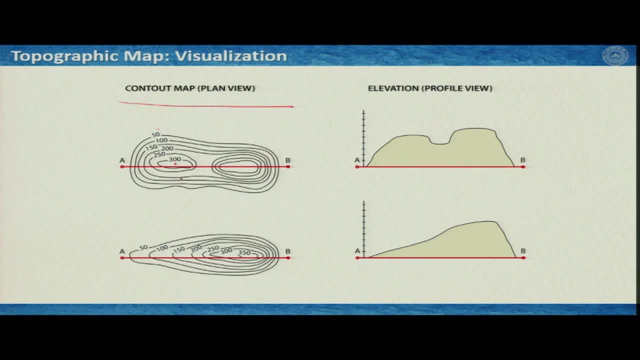 peak here and here is the highest point and it is marked by a concentric circle. Now, if I have to make a cross section from A to B of this region, then I should get something like this. So if I see something like that and the values are given, then it should be. 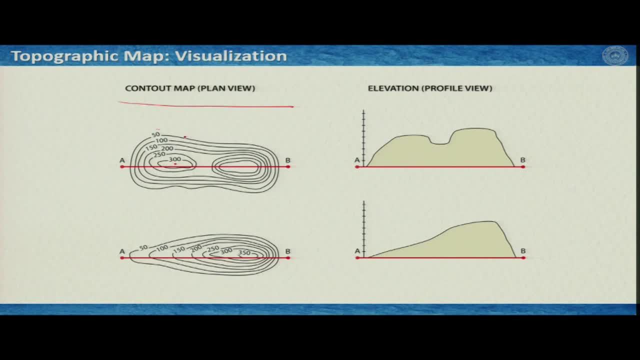 like this. Now, if the values are opposite way, for example, this one is 300 and this one is 50, then A to B in this case should be something like that. So these are actually depressions, but here the values are increasing towards a core of this contour. So this is: 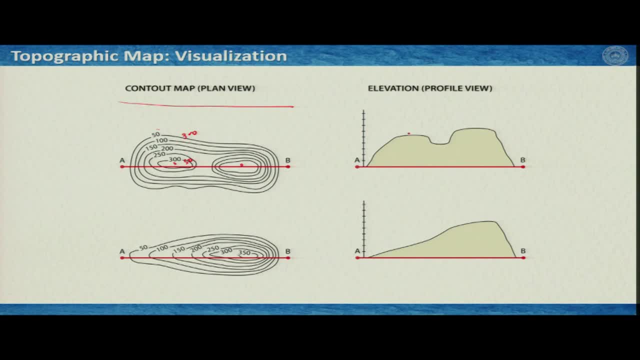 you have two hillocks here, one hillock this one, another hillock this one. So this one and this one Very similarly, you see here as I talked about. So here we start again at 50 and end up 350 meters. In this side the contours are closely spaced. in this side contours are 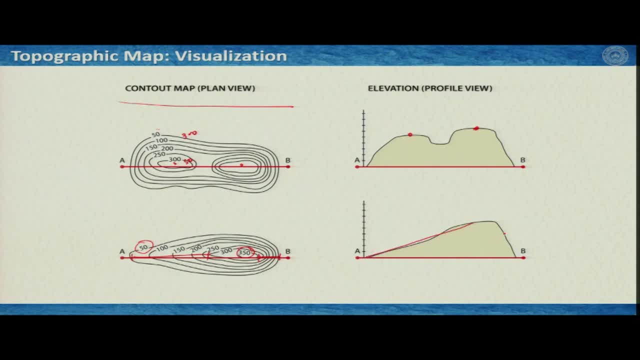 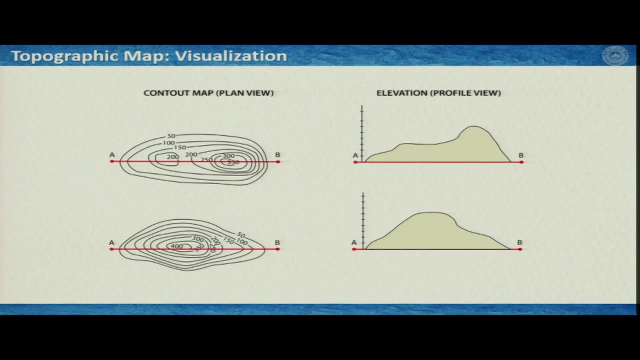 not that closely spaced. So here the slope is very gentle, here the slope is extremely steep. So just you look at this contour pattern and you can figure out what is the section or how it should look like when you actually see them in the field. This is another one. 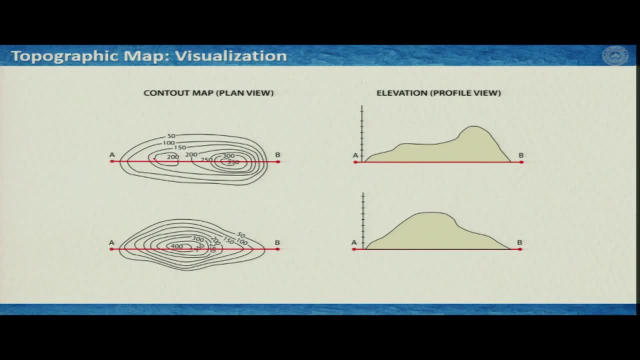 So you see, we have two concentric circles. So you see, we have two concentric circles. So you see, we have two concentric circles, But this concentric circle closes at 200 meters and this closes at 350 meters, So therefore, this must be of higher elevation compared. 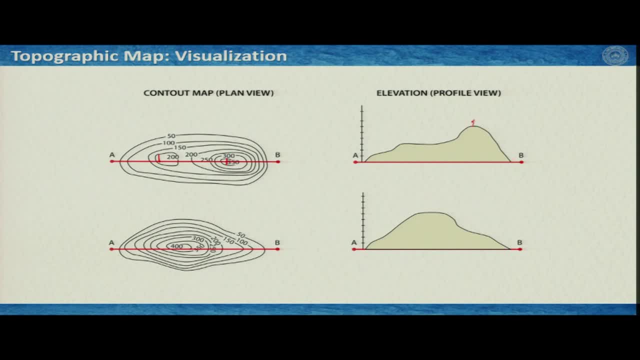 to this and if you make a section, you actually can see that this is your 350 and this is somewhere is your 200. So this is how you actually visualize. and this is another one. we have a single peak and we get a single peak here. We will see in one of the next. 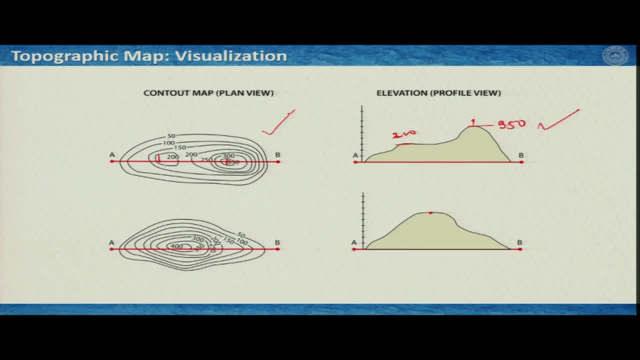 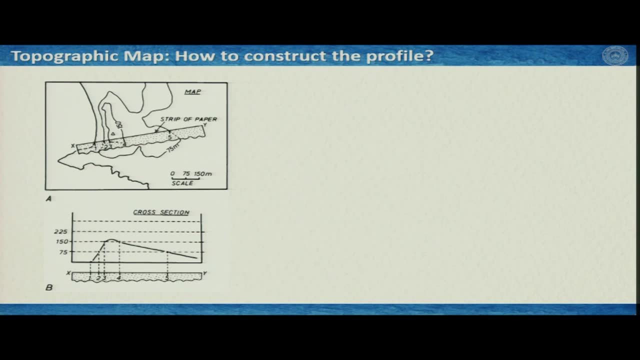 slides that how to construct. So we have to construct this elevation map, profile map from this contour maps and this is exactly where it is. So we will have a lab demonstration on this, but I explain you briefly. So whenever you see a topographic map and if you have to draw the profile, the 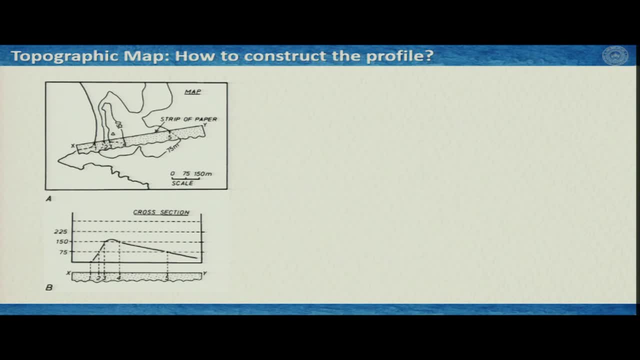 first thing, you have to decide that from which section you would like to draw the profile. For example, here the profile should be drawn along this line. So this is x and this is Y. Now we have series of contour lines. So, for example, this contour line is 75 meters. 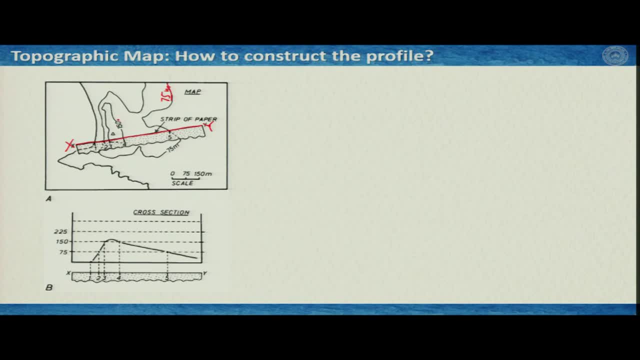 and then this contour line is closing here, and then we have 150 meters here, which is this one, and if this is 150, this is 75, then this one should be even lower. but if we do this, then we can figure out that it is cutting across this xy line. the number of contours: 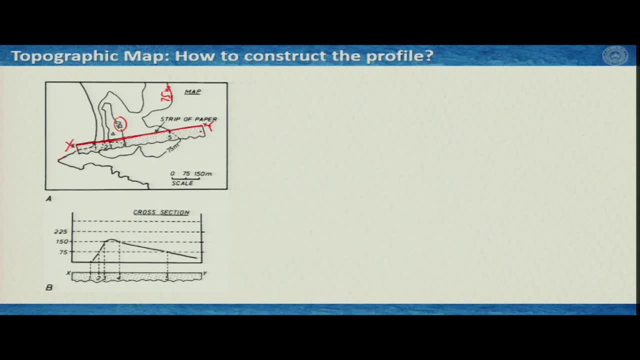 So what you do? you take a strip of paper, which is this one, and align the edge of this paper along xy line and once you align it, then you mark this places or points where it is interlinked, So intersecting the contour lines. So here, for example, number them 1,, 2,, 3,, 4,, 5 and. 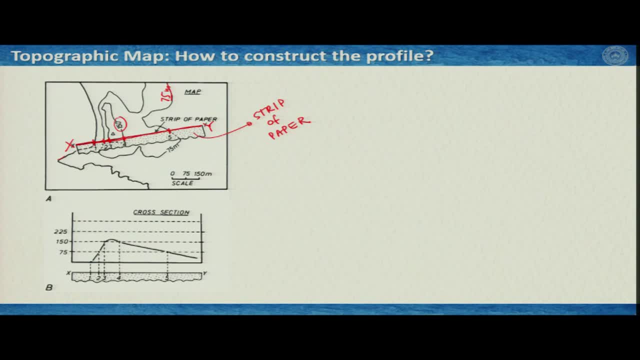 so on. Once you are done, then it is important that you draw a Cartesian coordinate system where your horizontal axis should be the distance xy and this should be your elevations, and this distance you can fix by yourself, depending on the scale you would like to see. but may? 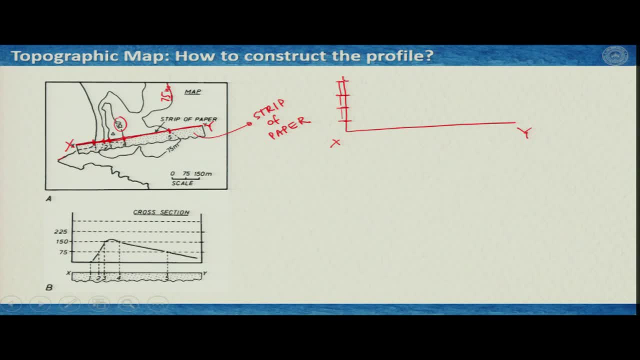 not make sure that these are all equal. say, for example, you can figure out that this is 75 meter, this is 150 meters, and so on. Now you arrange your strip here, this paper strip that you have, where you have marked this one, then 2,, then 3,, then 4, and then 5 intersections of the strip of the paper. 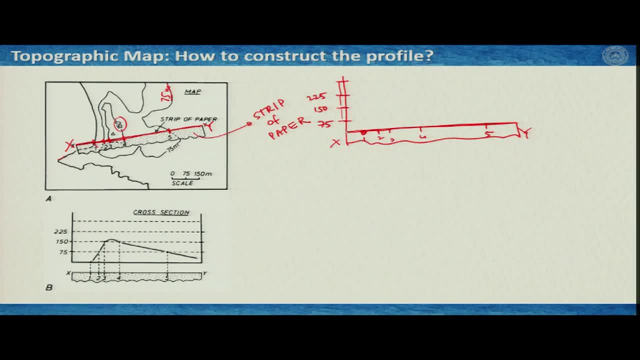 So this comes here And you see that at 1 your value is almost at the C level. So because this is C, So this is close to 0. So at 1 you have somewhere here. Then at point 2, here the value is 75. 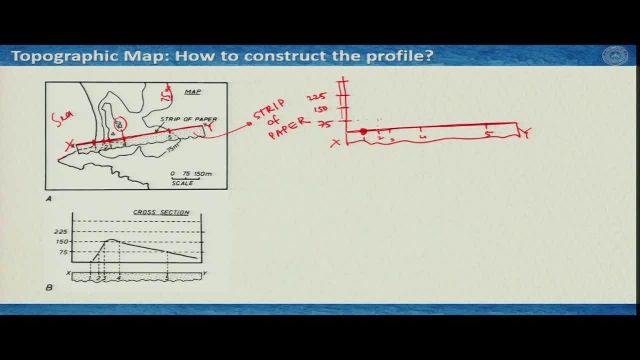 meter. So you have to plot a point here at 75 meter. At 3, your value is 150 meters, the value of the point 3.. So you come here and the value is 150 meters At 4. again this contour. 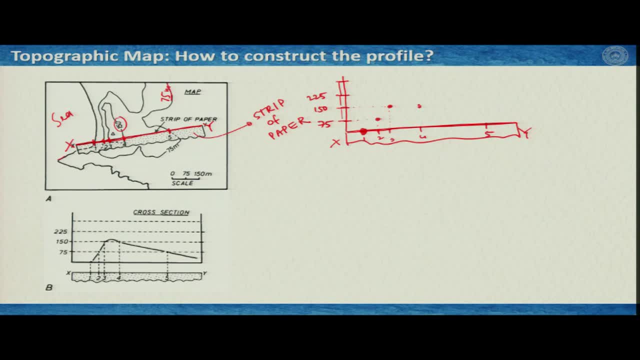 is coming back and we are at 150 meters. So we come here and plot it like this, And then, at 5 again, we are touching the 75 contour. So it is like this. Of course you can grid your map first, So that you do not have to do it, but once you are expert, you 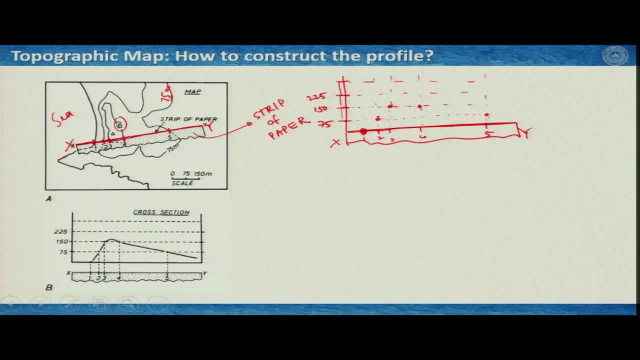 can do it just by putting your scale accordingly, the way you need. But these are the points that we got and simply you can connect these points like this: Now here, you can make it flat or you can make it little curve. there is no harm. So this is the elevation or profile. 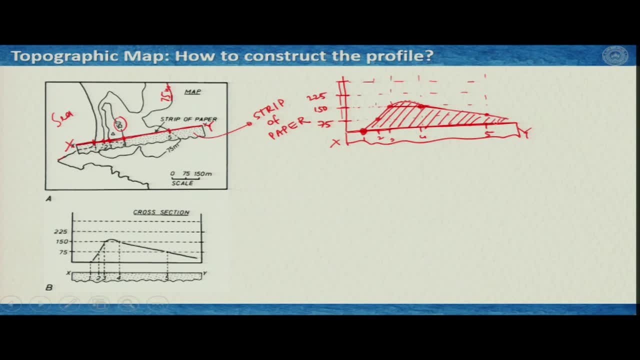 along x-axis, Y line of this. So does not matter how is your topography and so on. You can cross section, say A to B, say this is 20, this is 30, this is 40,, this is 50 and this is 60. So if you 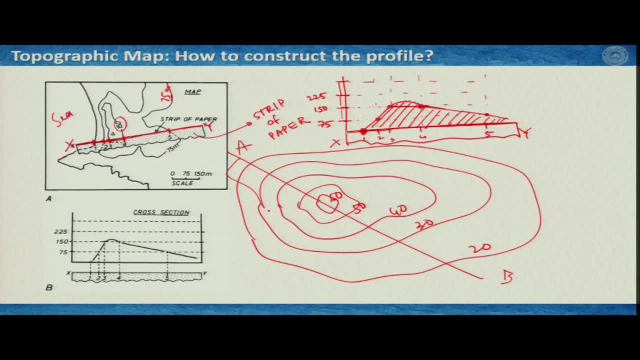 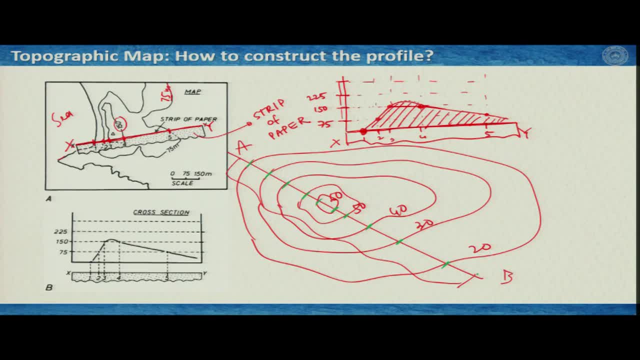 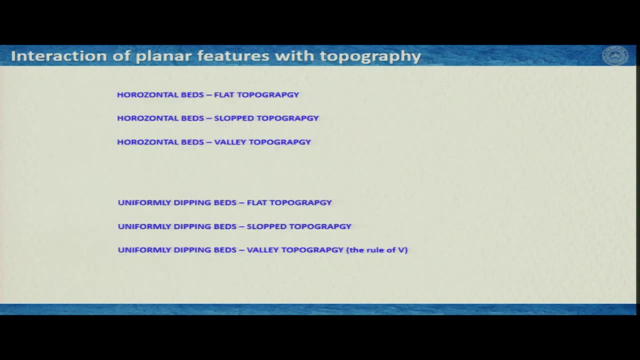 again make your grid and then you know the values. you plot it, you will get series of points and then you are done. But we will have little lab demonstration on this, that- how to construct the profile from a topographic map. Now let us come to a very important part: that so far we have figured out what is topographic. 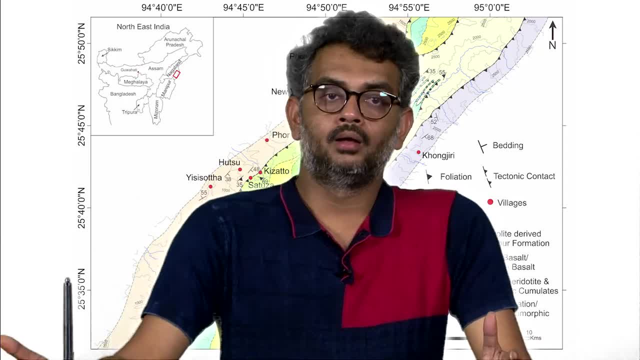 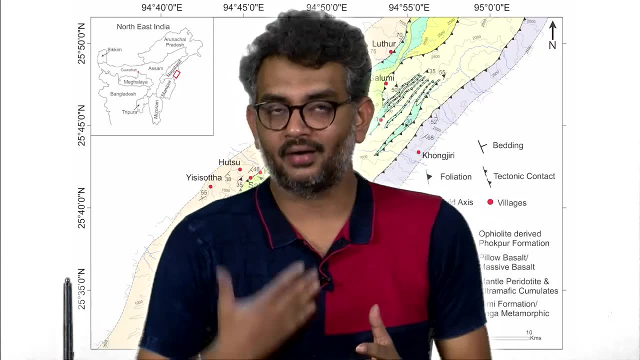 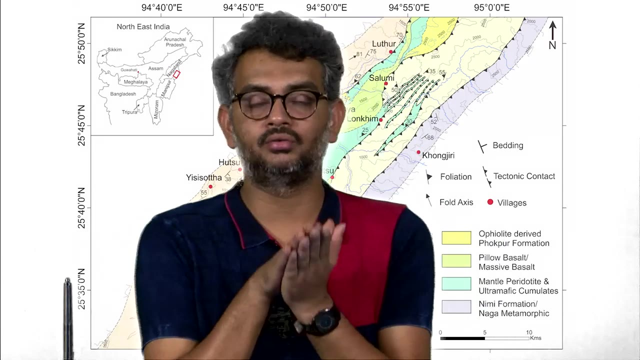 map, how to get the profile and so on. But you may have different lithologies which are intersecting or interacting with the topography. For example, if you have a flat horizontal bed and if you have a flat topography, then you do not see. 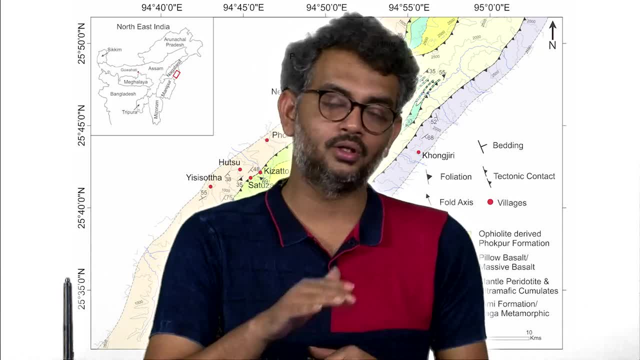 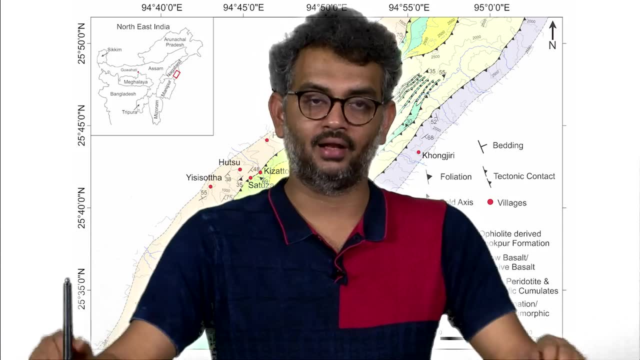 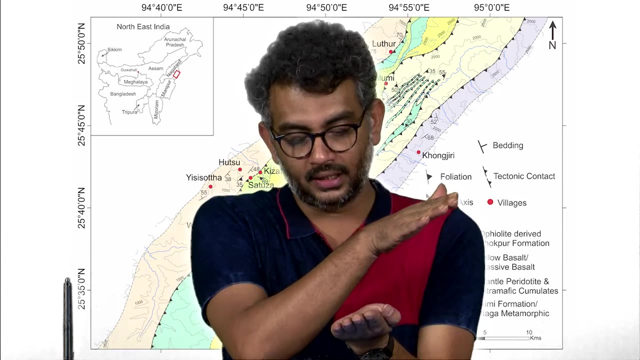 The other beds, which is below the flat bed, because it is only single bed. you will see, because bed is flat, topography is flat. Now, if your bed is again flat, but your topography is in a particular slope, in a very gentle slope, then topography would go down and at. 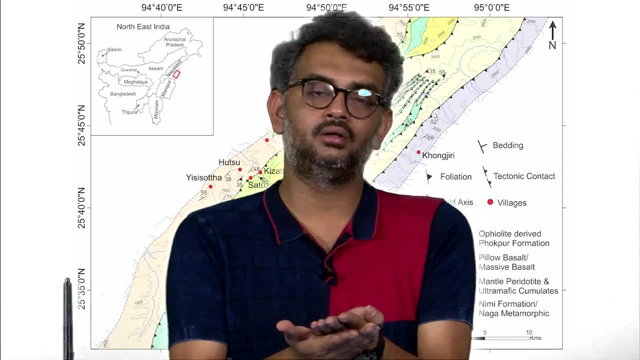 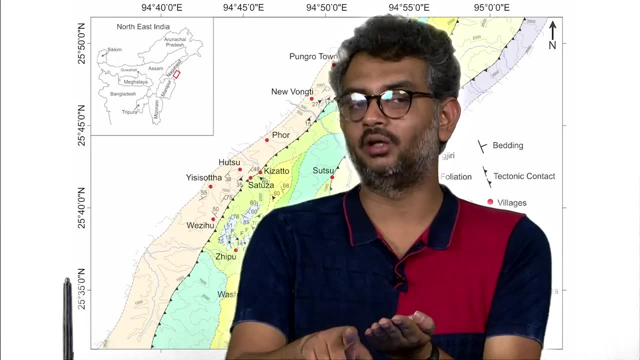 one point of time it would cut the contact between one bed And then your topography will also cut the contact between the 1 bed to other bed. So other bed will be exposed on the topography and this can be a valley topography, a mountain. 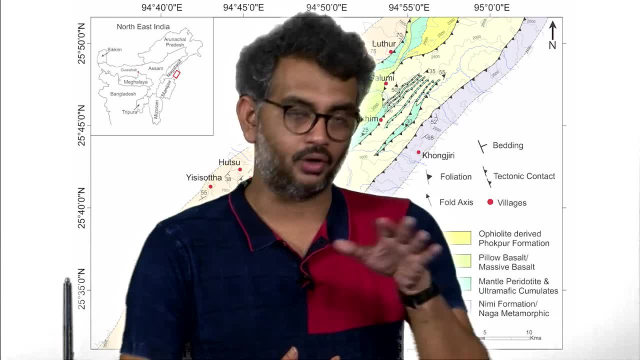 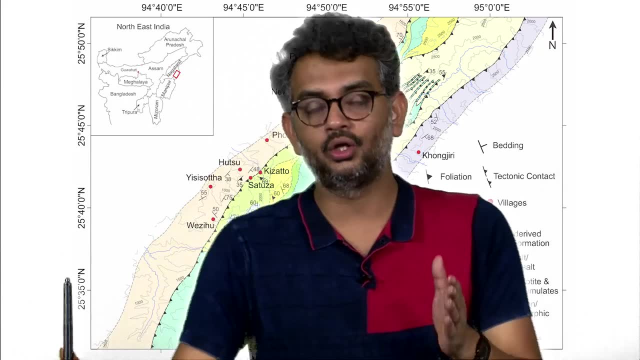 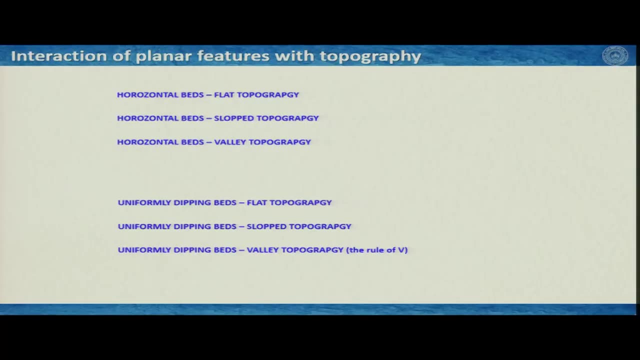 topography and so on. So there are 3 possibilities that you have horizontal beds with – 1 is flat topography, slop topography and valley topography. Then you can have uniformly dipping beds and again you can have flat topography, slop topography and valley topography. 사람. 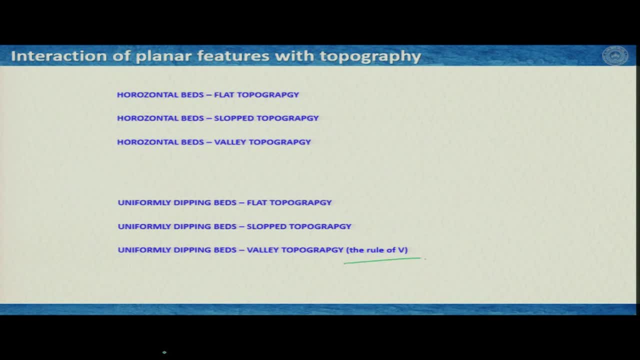 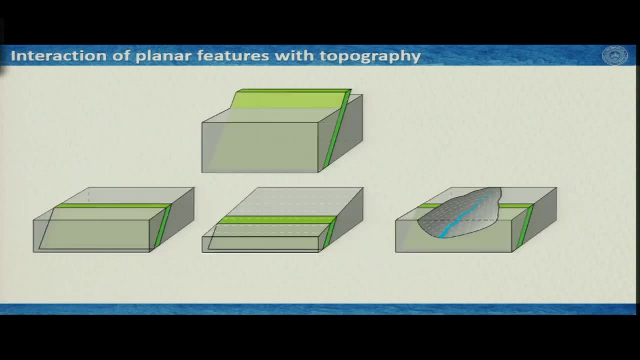 106.5.. rule of V is: we will learn about it soon, But let us try to understand this process in a better way. Say, for example, you have a bed here like this, which is the green one, which is sloping, and this is some other rocks. So we have a bed which is sloping in this. 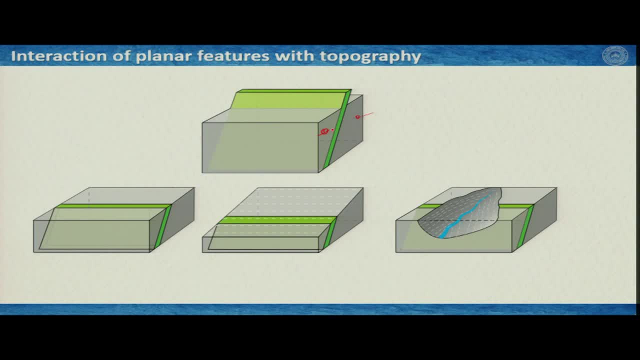 way and then you have some other rocks around this. Now, with time, what can happen? it can erode uniformly. So you see that this got eroded and because this bed is sloping, then you can clearly see that this is a horizontal surface. So you see that you have, say lithology. 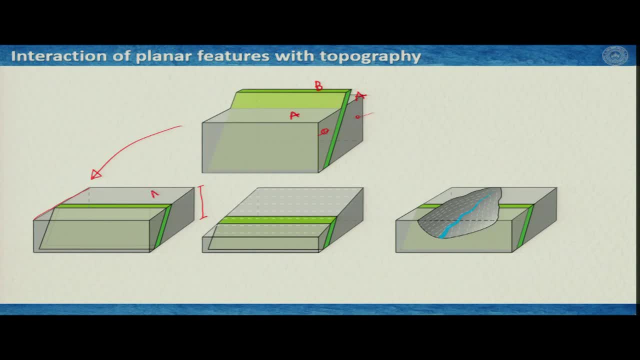 A, then lithology B and again lithology A. So you have A, then B, then A, and they are absolutely fine. no problem Now if the erosion happens and you get a slopey topography. So the topography is uniformly sloping here. 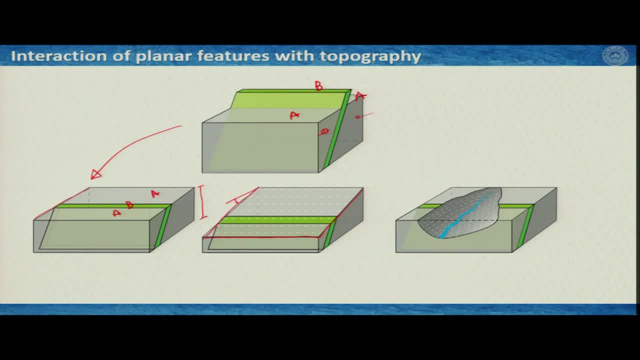 As you can see here. So this is the slope. Then you of course generate some contour lines right. this white dotted lines are your contour lines. And again there is no variation here, except the bed thickness changed on the exposed surface area. But now if there is a river, 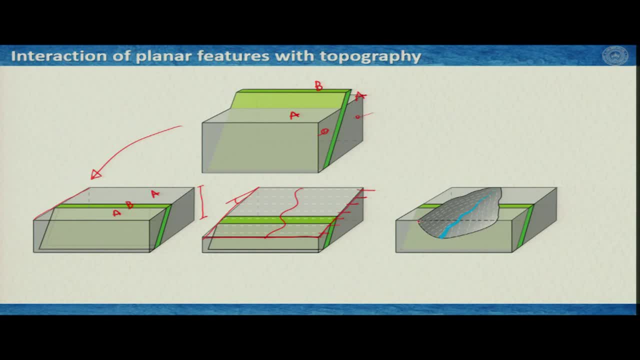 flowing here, as we see here, So it would cut a gorge or make a canyon or whatever. then the question is how, on this river valley, this bed would look like right, because it would have also contours like this. So would it look like this or would it be a straight? 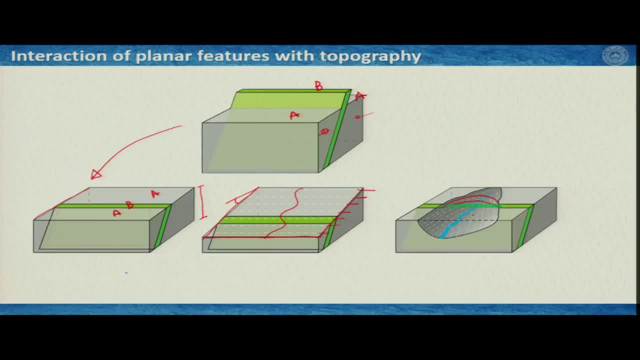 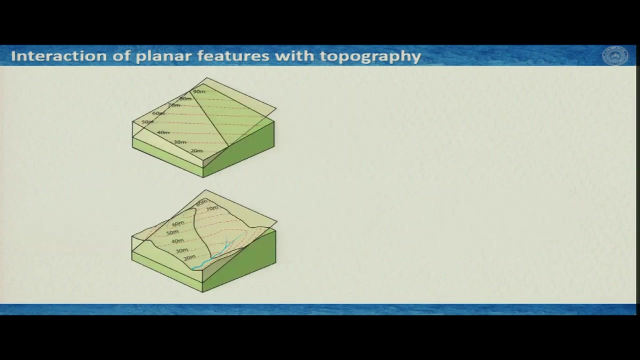 line straight bed, or it would be like this and so on. You may guess how it should look like, But there is a rule, and this rule is known as rule of Vs. We will see this soon, But before that, let us see some other interesting features. 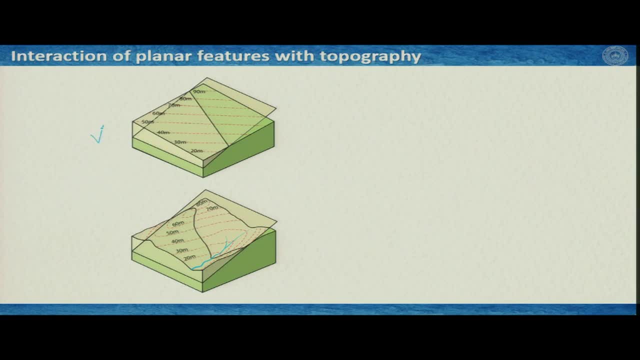 What do you see here in the first image or first illustration, that is, the surface of the earth, for example, which has a flat, sloping surface. And then you have two different lithologies, say Here is the green one and this light cream one is b, and their contact is somewhere here. 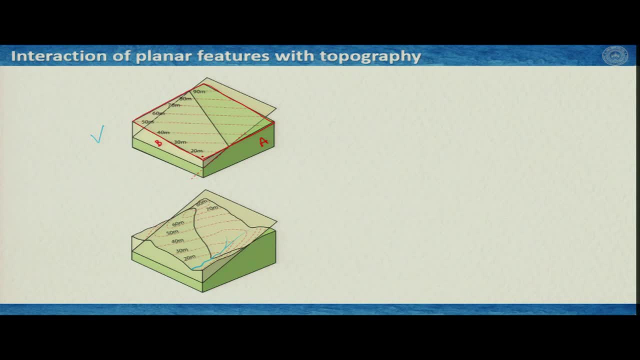 So when it intersects like this- and this is the topography, So this is the lowest elevation that we can see here, 20 meters, and it goes up to 90 meters towards this direction and this is the line it is cutting or intersecting the topography. This point is 90 metres And here you can see the contour lines. however, it is not cut into the topography. Of course. there is noă 3.5 ton at one point in this, anywhere, but in this surface where it is the topography. we had this now for that content that there is something like this seen at thisiert. So when this crossio, 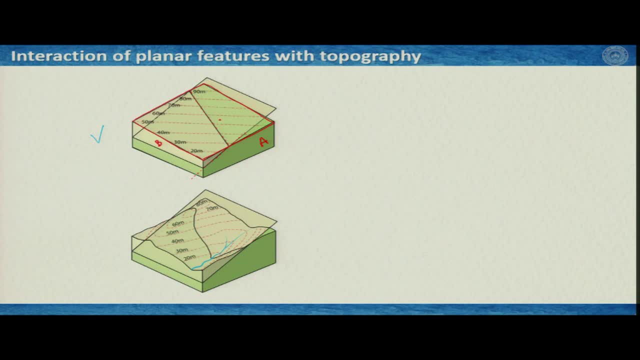 and soil flow into it. so we know exactly what the location of passes are. and thewith The이는com saying objetos: topography, the boundary between A and B. So in this side you have A and in this side you have B. You can also see that if this topography is not as flat as we have seen, 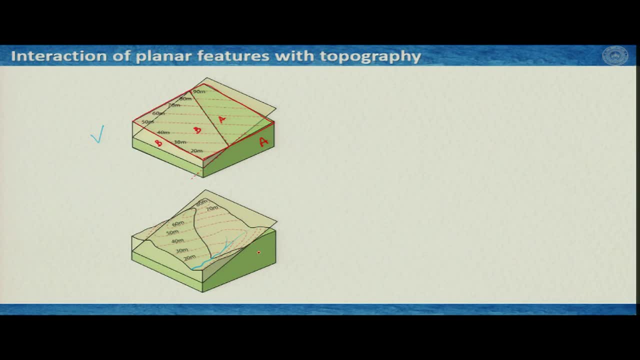 or maybe river is flowing along this. then we have very similar thing: A and B, the beds are dipping exactly similar way. So to strike and dip of these two contacts, lithological contacts, are very, very similar. but if I change the topography, in this case if I have an 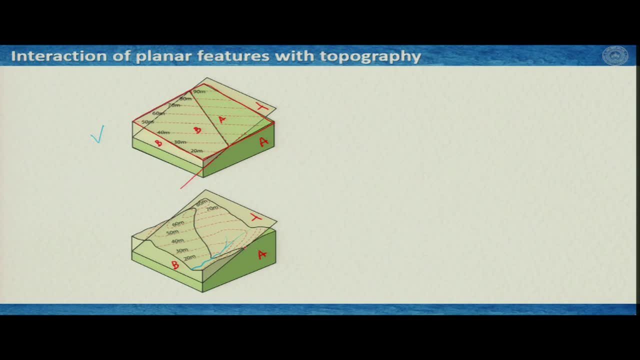 undulatory topography, then the interaction of this topography with this uniformity dipping bed would be along this line. So here you have A and here you have B. So if I try to see them, this is a block diagram. if I see them in a topographic map, their appearance. 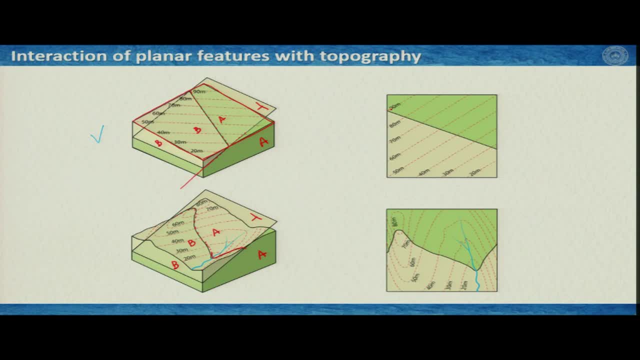 would be something like this, If I have to plot it. So here, because the topography is flat, we clearly see that the flat bed interacting, uniformly, dipping bed which has no deformation, it is not folded or something like that. this is very much straight line. But same flat bed if the topography 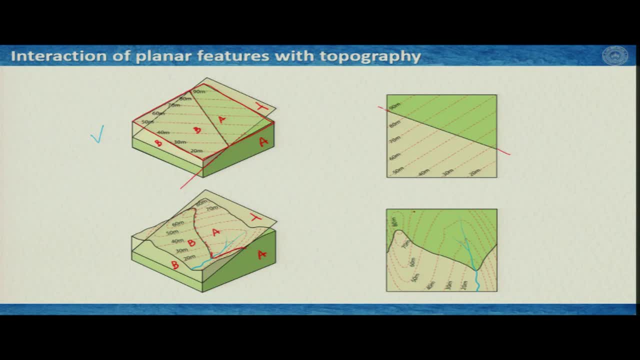 is undulating, then, which is given by this little red dashed lines, then it is not anymore a straight line. So there must be happening something, And I would like to also emphasize the fact that we have already talked about that. you see, here this appears like V or in. 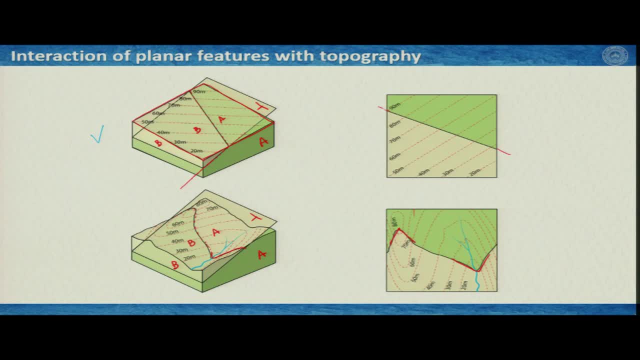 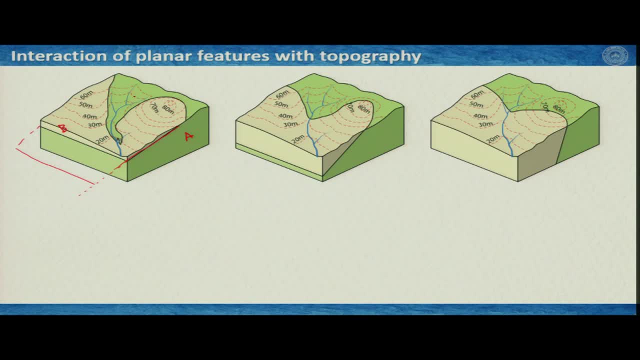 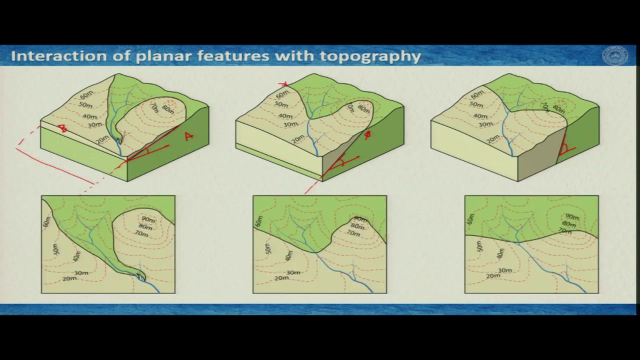 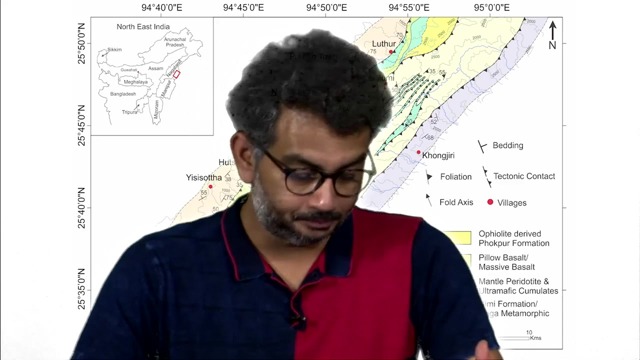 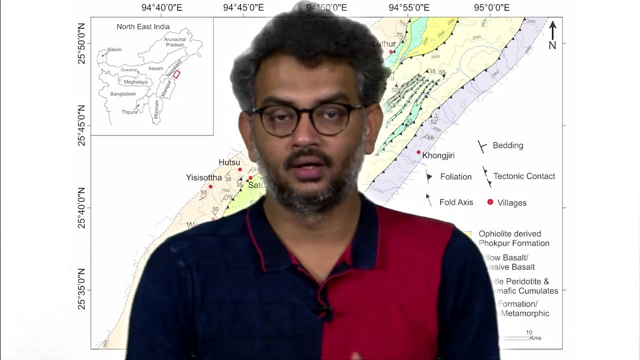 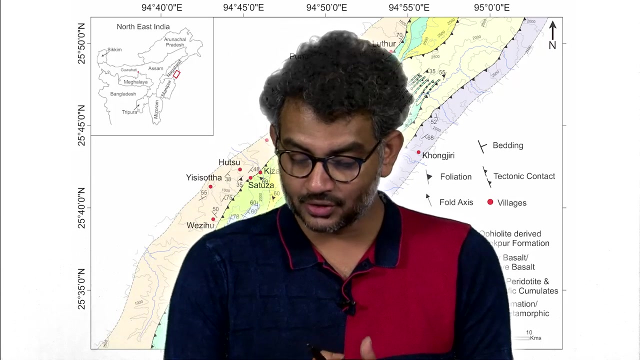 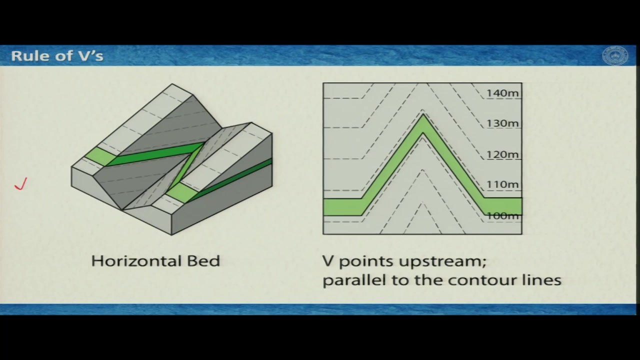 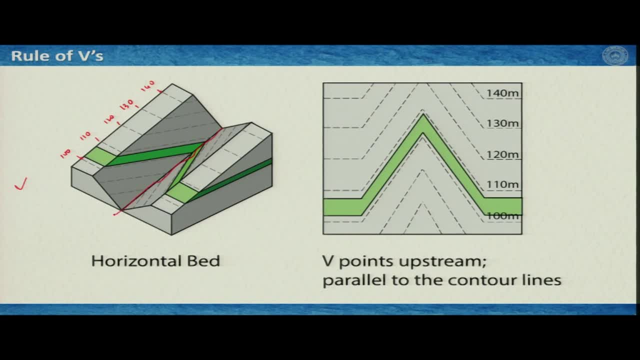 And you can imagine that river is flowing in this direction. so this is the downstream and essentially then this would be the upstream. So river itself has a slope and this is also maintain a slope- the walls of the valley- and this is horizontal. So in this concept, we will first look what happens if we have a horizontal bed in this. 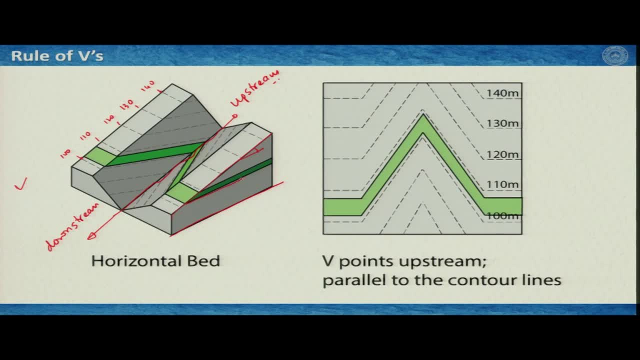 condition. So horizontal bed means that this dip is zero here. And we see, if the bed is horizontal, then the V rule suggests- and this is the top view on the topographic map. so this is the topo map. So the way the horizontal bed would intersect the valley or it is something like this: 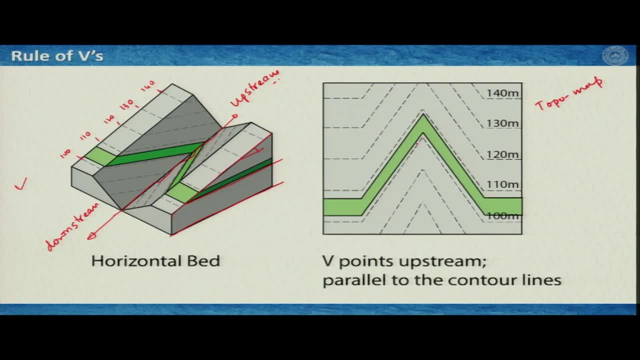 So it would the V that would be created. it would point upstream. So this is exactly Exactly what we see here, and the angle of V is very similar to the angle of the contours or contour lines we can think of. So if this is alpha, then this has to be also alpha. 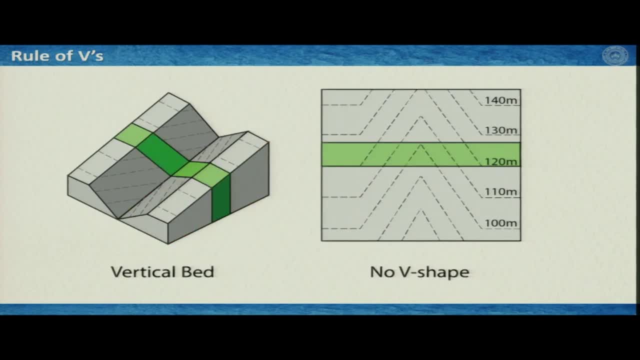 What would happen if the bed is vertical is given in the next slide. If we have a vertical bed, that means this is 90 degree and again, this is the downstream, that is the upstream And the vertical bed, interestingly, would not produce any V in this section, in the top view. 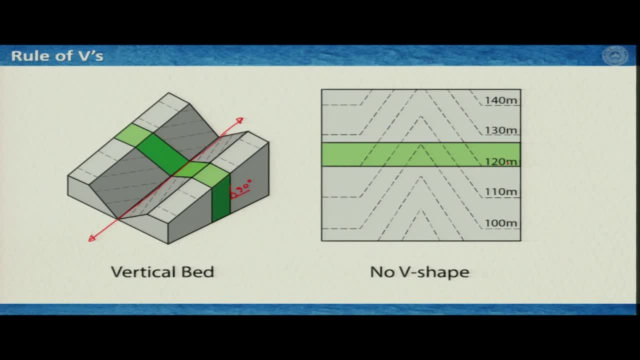 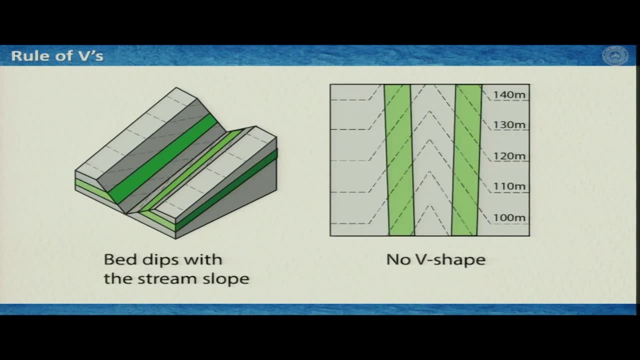 or in the topo map view. So it would not be influenced by any of the contour lines and it would run straight as it was. Now, if we have the beds which are dipping along the slope of the stream, that means the stream has a slope along which it is flowing. 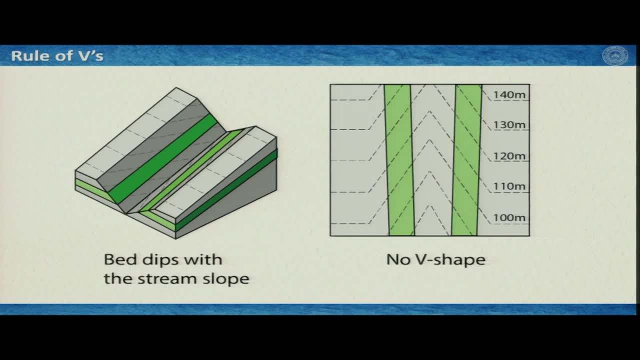 And the bed is 4rags, 5 cages, So we have the loop there and the vertical side should be 2rags and 2ikum Nummer. 2rags distance bed also has a very similar slope of the stream. So this is the deep of the bed and this is. 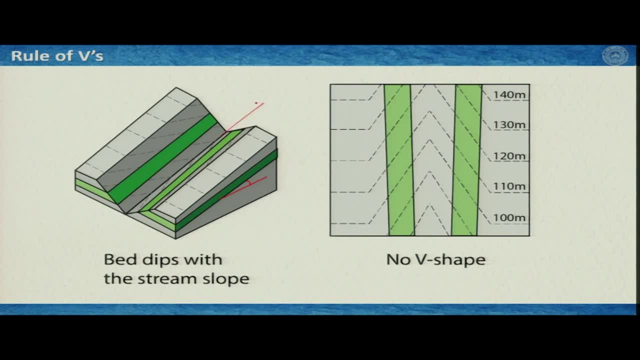 also the stream, the way it is flowing. So if this is the horizontal line, if I can reproduce it here, So this angle and this angle are very similar. In that case, the V rule suggests that you would not produce any V shape. However, the two projections of the beds on this V. 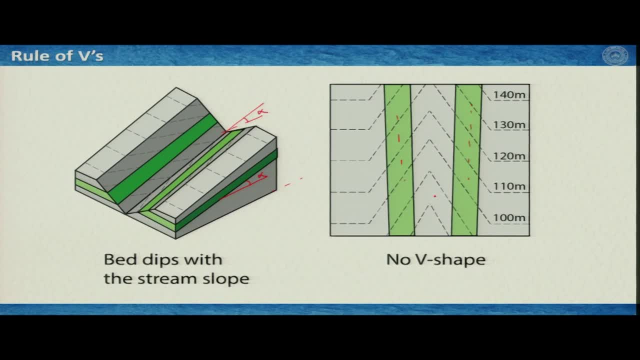 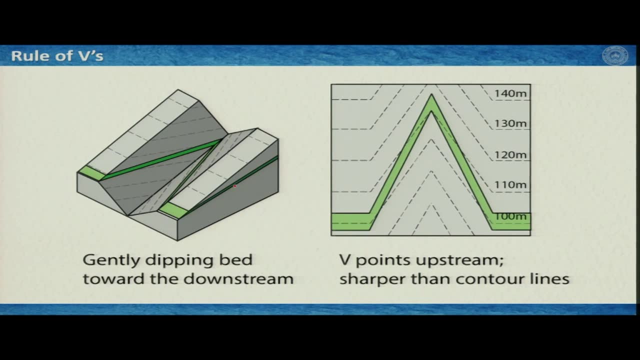 they would slowly try to intersect towards the downstream. if the bed is a gently dipping towards the downstream, So this dip is very, very low, low angle dipping bed, this is again the downstream- then the V would be something like that and in the plan view it would be very interesting that. 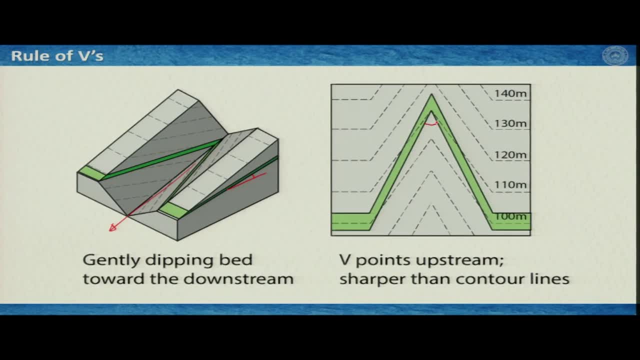 when it was horizontal, we saw that this angle of the V and this angle of the V were equal. But In this case, if the bed is gently dipping towards the downstream, then the angle made by the bed inside the valley, the V angle, if this is alpha and if this is alpha 1, then 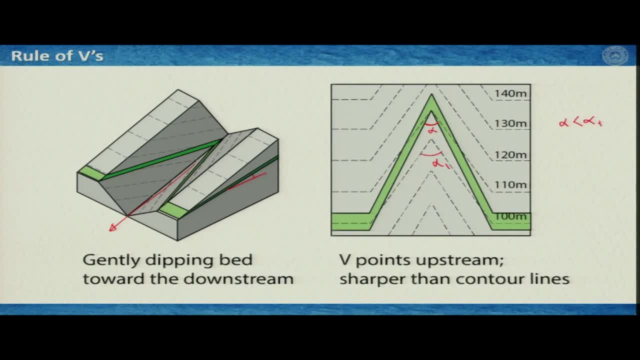 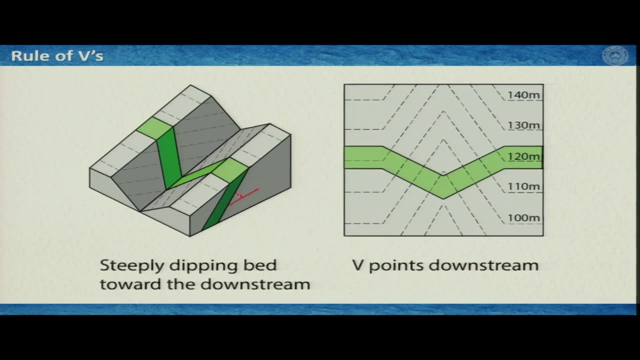 alpha is less than alpha 1.. So V points also upstream in this case and it is also sharper than the contour lines. Now if we have a steeply dipping bed towards the downstream so bed, the dip of the bed is very high. in that case we will see that V is pointing downstream in this manner. 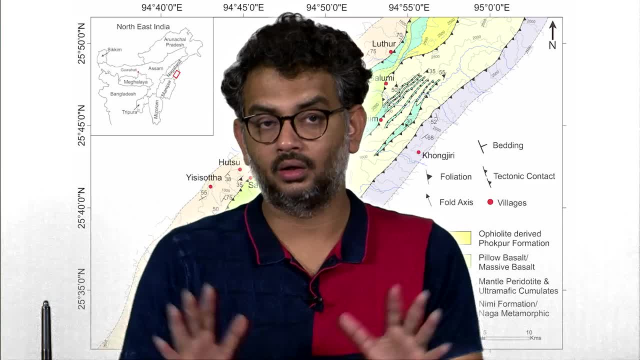 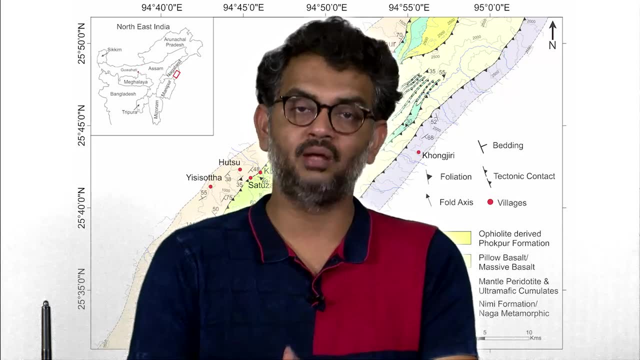 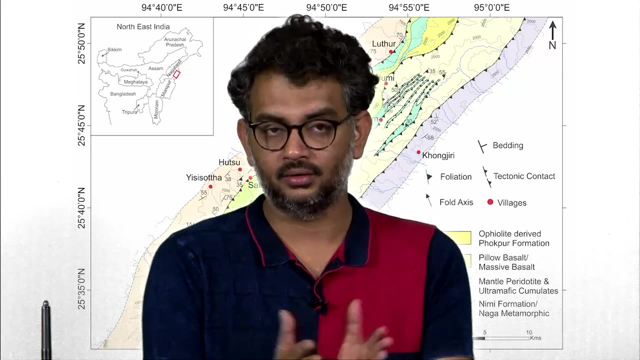 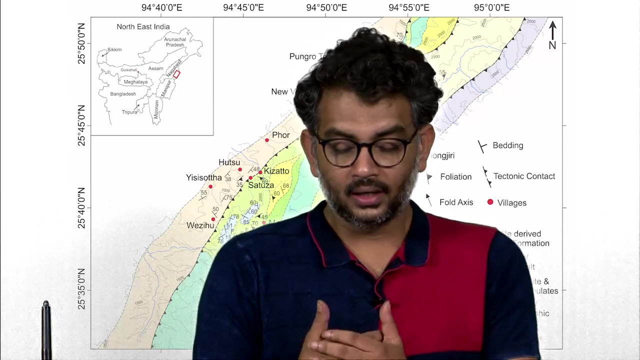 Now we will look at something very interesting, that how we can figure out the strike and then the dip of the bedding plane Which is uniformly dipping inside the surface and it is intersecting with different topographies. And if we remember the definition of the strike, then you can figure out the fact that strike 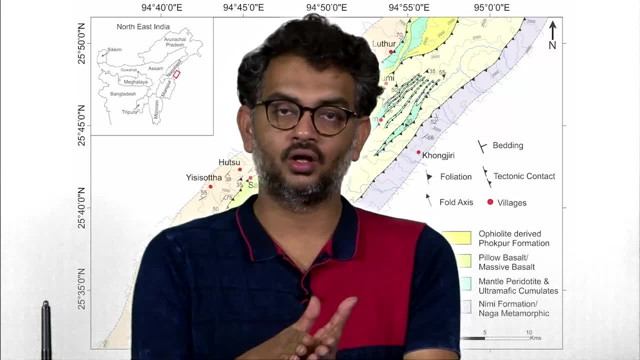 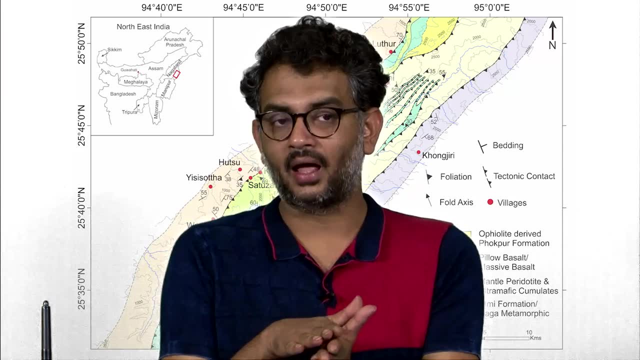 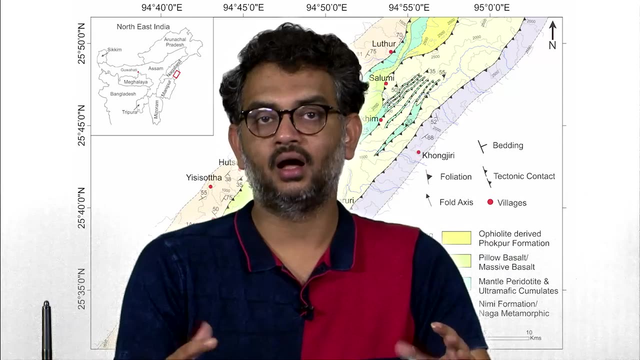 was nothing but the intersection of an inclined plane with the horizontal plane, and the horizontal plane is imaginary. So they would produce a line, The azimuth of the line. The azimuth of the line is the strike. So from that idea of the definition of strike we actually can construct on the topographic 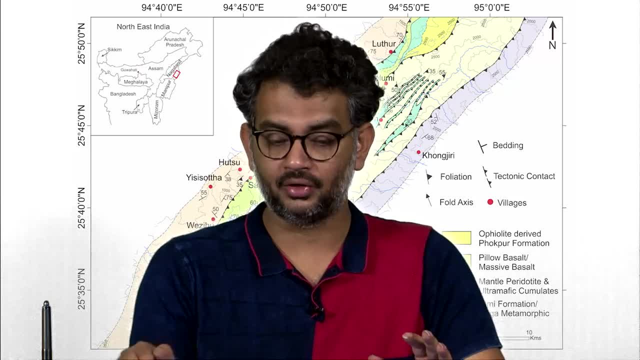 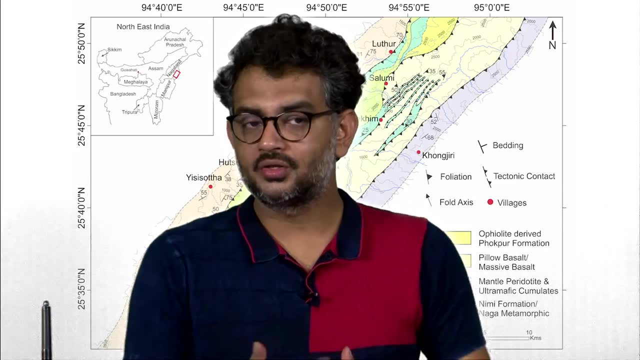 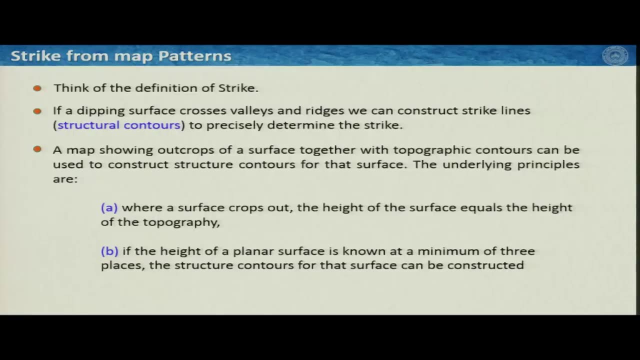 map, even if we do not go to the field. if we have this intersection line on the topographic map of a bedding plane, then we can construct something, what is known as structural contour. So if a dipping surface crosses valleys and ridges, We can construct. 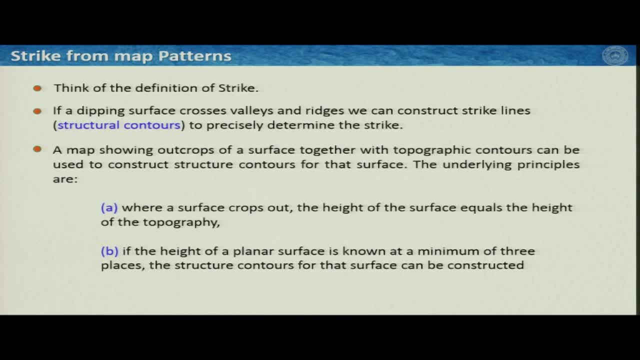 The strike lines, which are known as structural contours, to precisely determine the strike. Now a map showing outcrops of a surface, together with topographic contours, can be used to construct structure of contours for that surface. And when we construct the structural contours? it has two underlined principles. 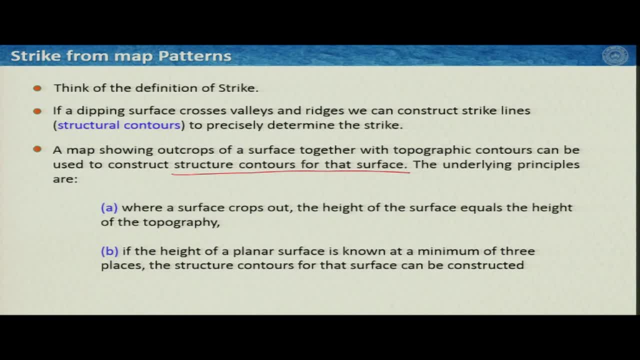 The first principle is where a surface crops out. the height of the surface equals the height Of the surface, Of the surface Of the surface equals the height of the topographic. So that means if I have an intersection point between the contour line of a particular value. 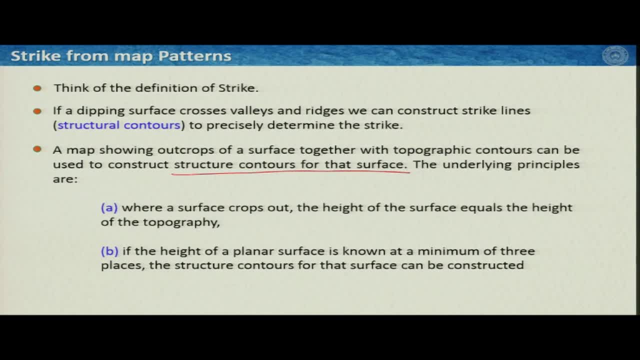 and also the intersection line of the two surfaces on the earth surface, then if I find a similar point somewhere and if I connect these two points, So these two points would have also very similar elevation value. and if the height of a planar surface Is known at a minimum of three places, the structure contours for that surface can be. 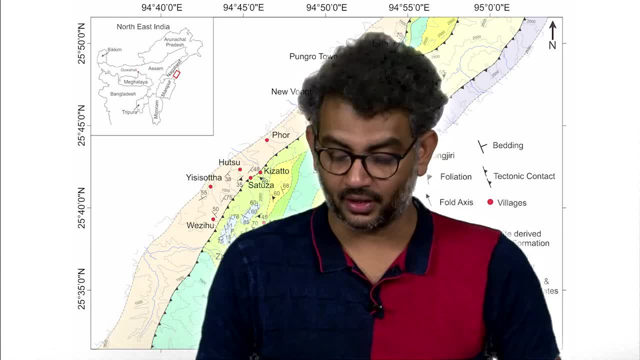 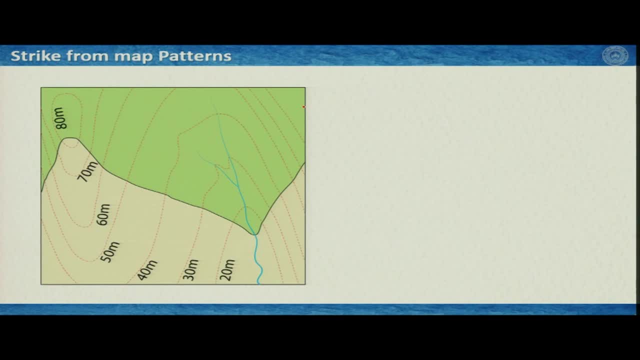 constructed. So let us see how does it work? I think, instead of reading the text, let us do this directly. We have seen this illustration before. this was an uniformly dipping bed. So what is important? to draw the contour lines- structural contour lines- that you have to. 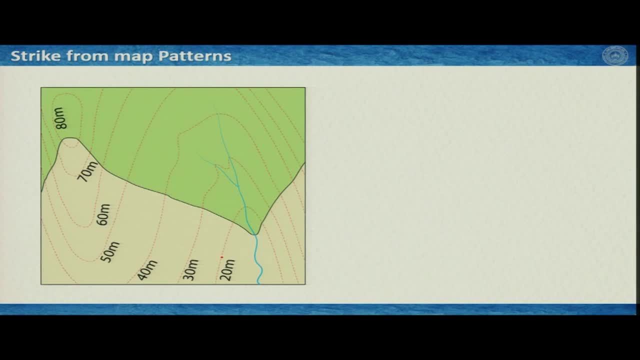 figure out the intersection between a fixed value contour line, For example. These are very common, So these two points are relevant for twenty meter contour lines. Now, interestingly, if this point is a and this point is b, As both point a and b are falling on the contour line, 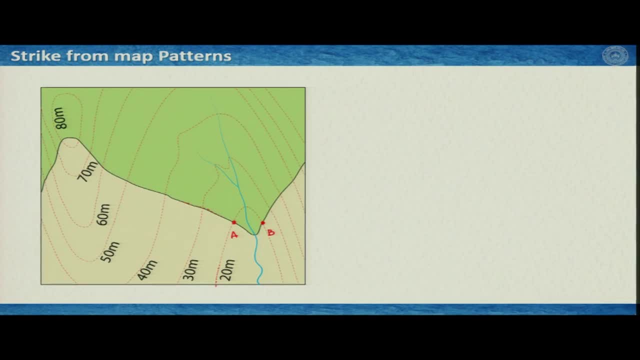 the elevation of A and B should be same At the same time, this point A and B also showing you the fact that the elevation of underlying bed, or the intersection between these two layers, this green and creamy layer, also has same elevation values at these two points. 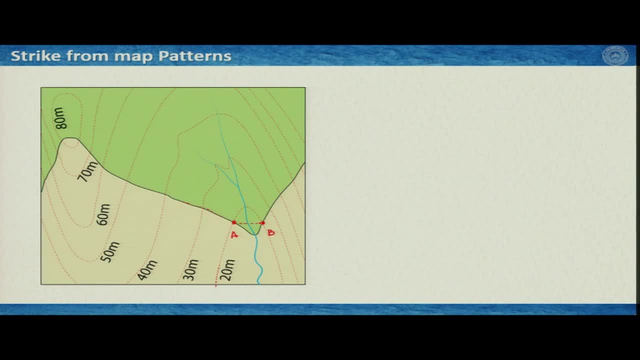 So I can actually construct a line like this, and this line indicates that this bed has, or this litho boundary has, an elevation of 20 meters. Let us go to the next contour, which is 30 meters. Now, again in a similar principle, we can figure out that where this contour 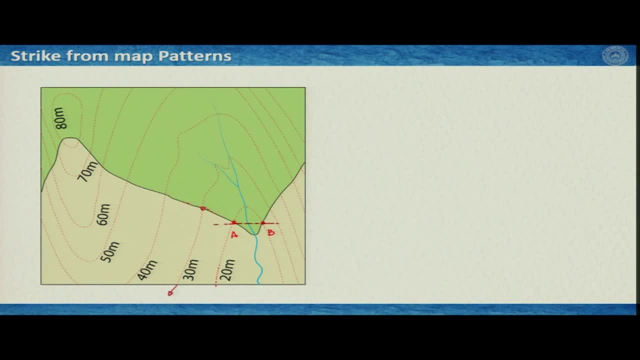 is intersecting the boundaries between the two litho boundaries. So in this case it is here and this is coming around, and in this case this is also here. So, similarly, if I consider this A 1 and B 1, then point A 1 and point B 1 has similar. 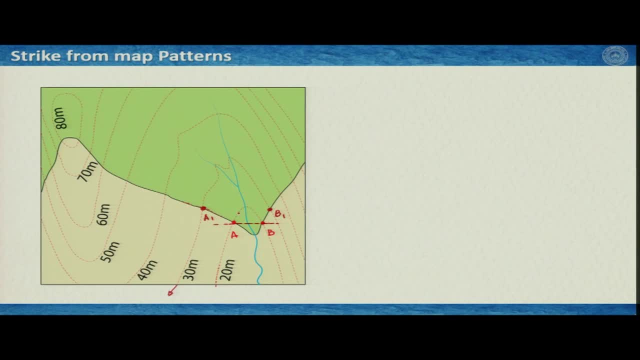 elevation, and because these two points are sitting at the intersection between the two lithologies, So the lithology itself has also similar elevation, So I I can draw another line here, suggesting that this is 20 meters, this is 30 meters. These 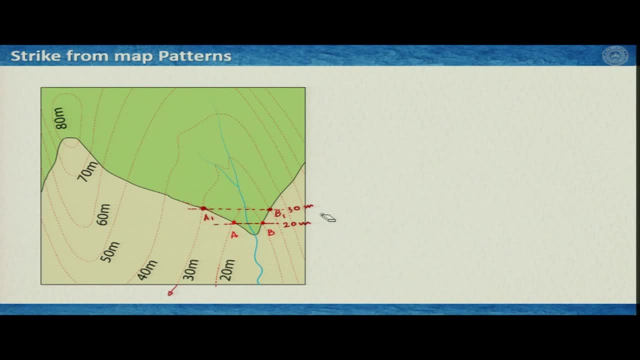 two lines indicates that the boundary between the two litho units have similar elevation along these lines. Similarly we can construct for the 40.. So 40 meters contour. So it goes like this: comes back here again to draw a line. 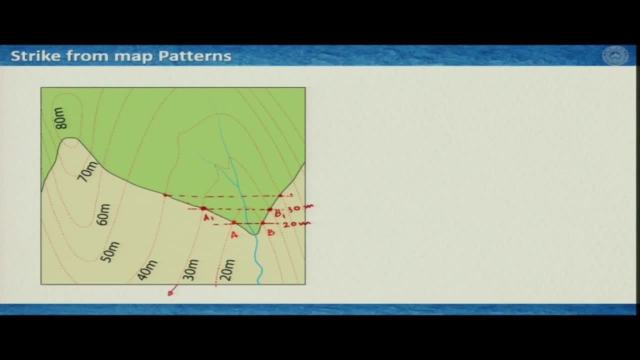 We can draw a line like this: We can figure out the 50 meters here, and then it goes and it comes here again. Interestingly, this 50 meters also crosses another point here, and that is actually the perfect one, because now we have three points So we can construct. 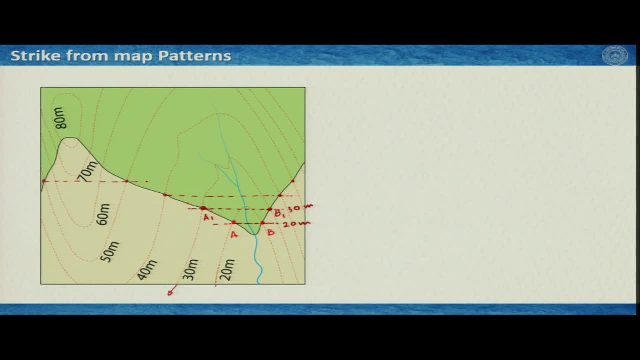 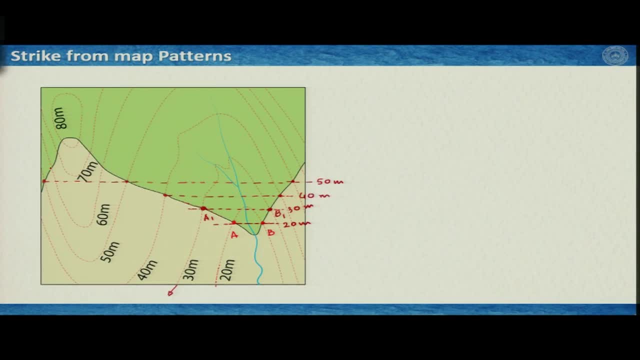 This was of 40 meter. We can similarly do for 60 meters here, here, and it is coming here and again. it is possible that we can. What is interesting, You see that these lines are parallel to each other, dotted lines that we have drawn this: 20 meters, 30 meters, 40 meters, 50 meters and 60 meters. 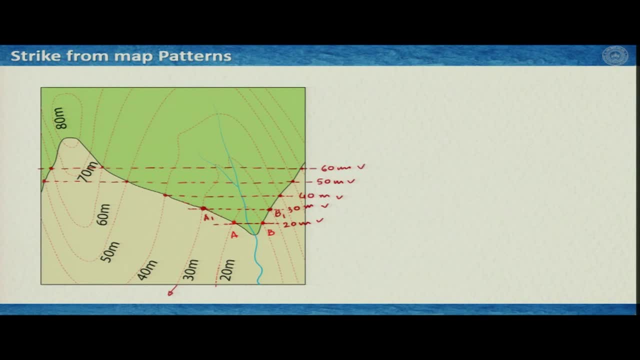 suggesting the elevation of the bed or of the lithological contact. these are parallel. So first hand they are telling you that the bed is uniformly dipping and the next one is 80 meters, and it is also running parallel. Now, these lines, what these lines actually do signify? they signify as I talked about. 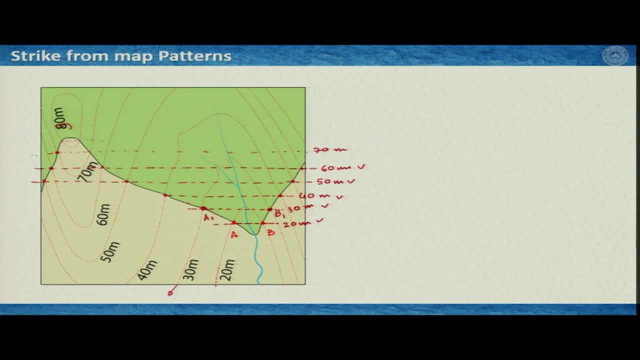 that the same elevation of the bedding plane, The contour lines that we have seen here. these do indicate same elevation on an undulatory surface and these lines indicate the same elevation of contact or lithological boundaries or a bedding plane or an uniformly dipping plane, And these are known as. 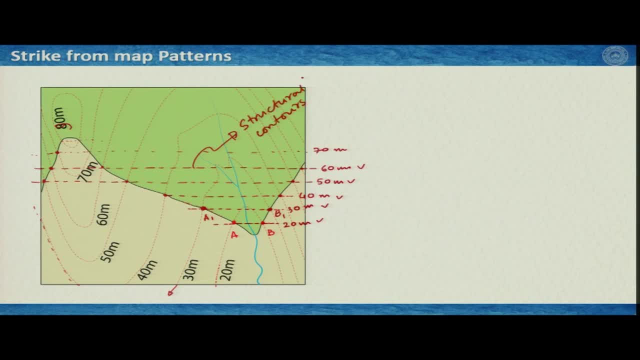 Structural contours And we see that these lines actually are horizontal lines at different elevations. So the bed is inclined and I have their intersection line on the horizontal plane, which are all these lines? So these line, the orientation of this line, if this is, is the strike line as well. 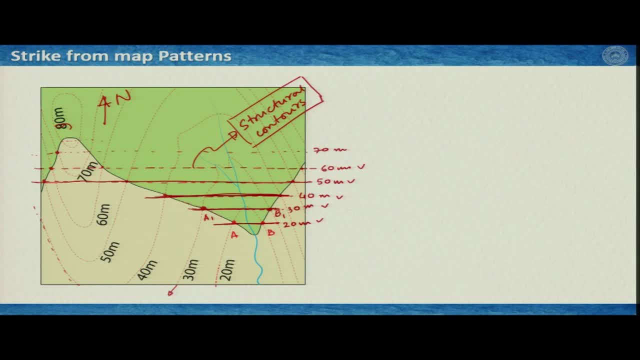 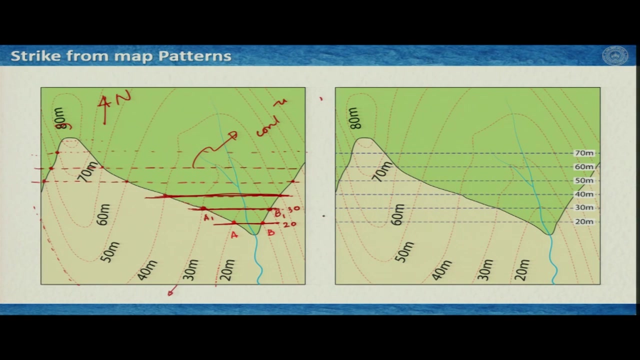 Okay, So in this case the strike line is oriented east west. So this is how you construct the strike lines, and if we have to see it in a different form, it is something like that: So you can construct series of structural contours, and structural contours are essentially 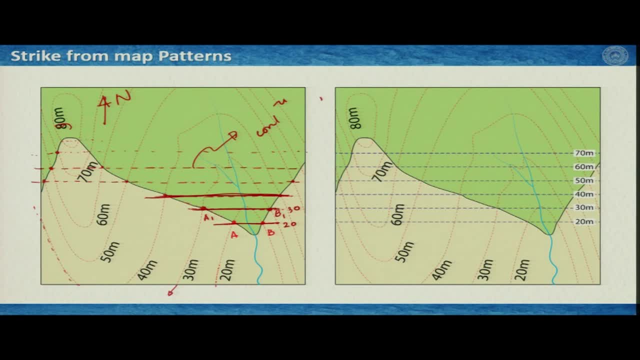 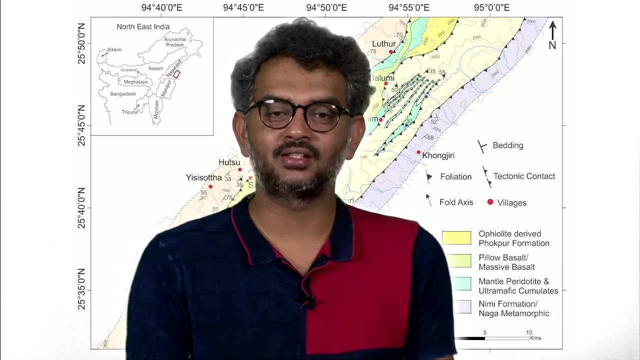 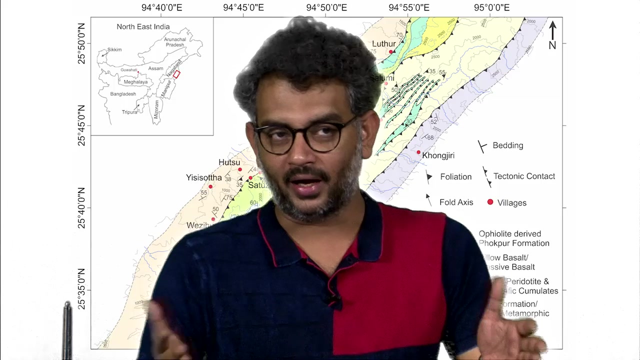 different to that of the topographic contours. unless I let you decide what, it is, Okay. There should be a specific condition, say, for example, if the bed is horizontal, then the structural contour should be exactly similar to that of your topographic contour. Now, this is how we have constructed the strike, and now we will learn how to figure out the. 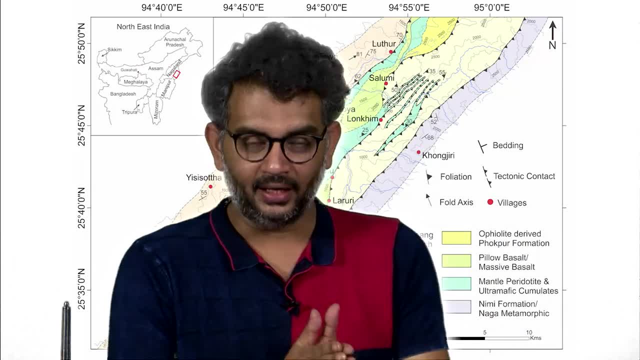 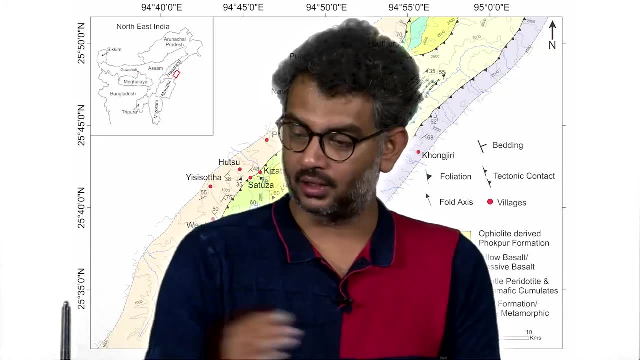 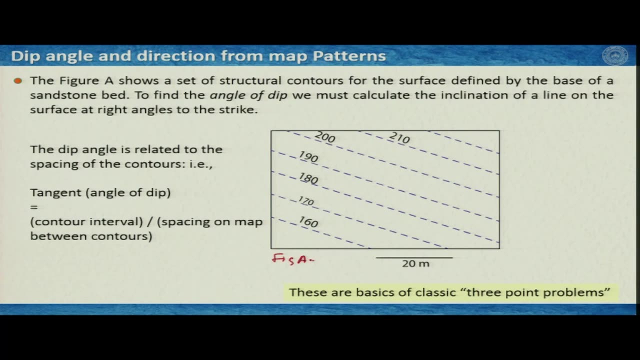 deep angle of the bedding plane or the litho contact from the structural contours. So do you have to draw the structural contours? So in this case, this figure, this is figure A, So the set of structural contours for the surface defined by the base of a sandstone. 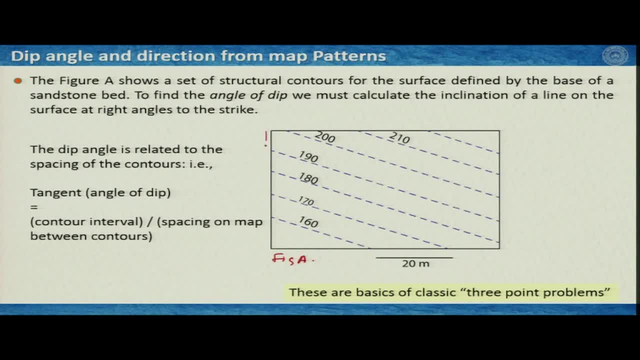 bed. this example I took from the book of Lyle. this is the north direction. So if this is the structural contour, then the strike is 120 degrees. So this is the strike line. So from north if you count, it would be 120 degrees. 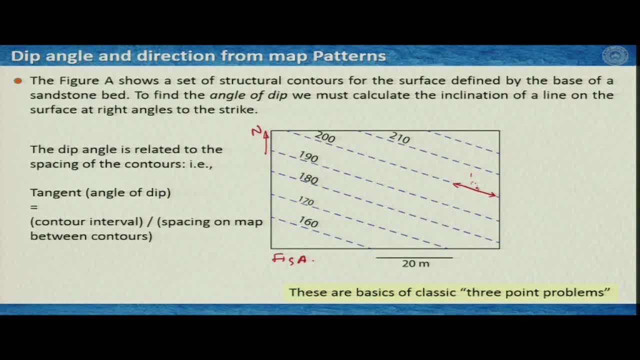 Now, to find the angle of dip, we must calculate the inclination of a line on the surface at right angles to the strike. So the dip we have to calculate at a right angle of the strike line. that is the definition, the true dip. Now one can be confused here. that which 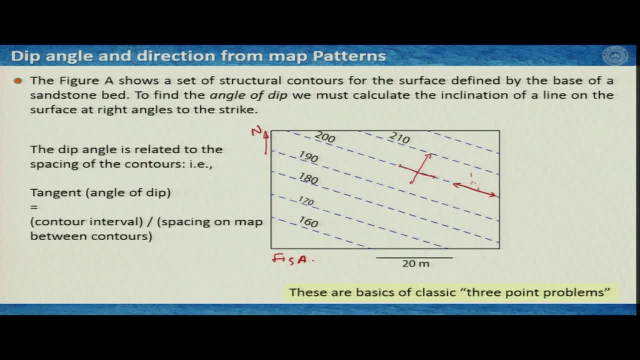 way the dip direction is. it is on this side or it is on this side. Now, that is not very tough job, because you see that structural contour is increasing this side. here it is 160, here it is 210.. So that means that the bed must be dipping in. 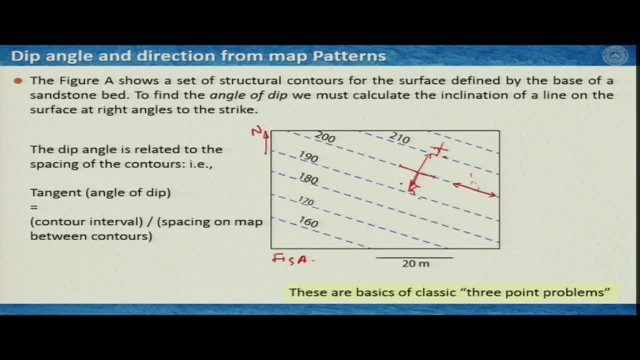 this side, not in this side, So dip direction is towards this side. Now to figure out the dip angle, what you have to do- So this is the section that will be working on- you simply have to draw a line like this: 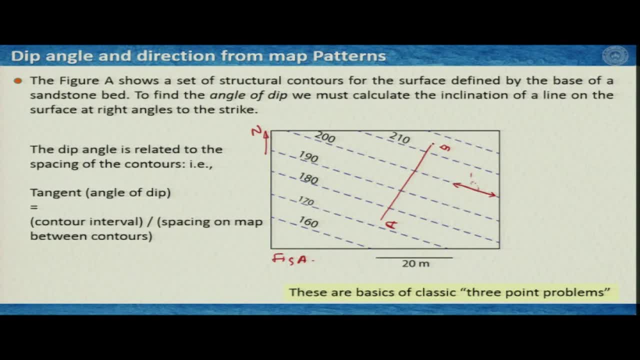 Say, Say A, A, B, and once the scale is given, you can have this distance and in a very similar way, the way we walked on the paper strip and so on. You can actually figure out this thing. So it first cuts 180, then 190,, then 200 and 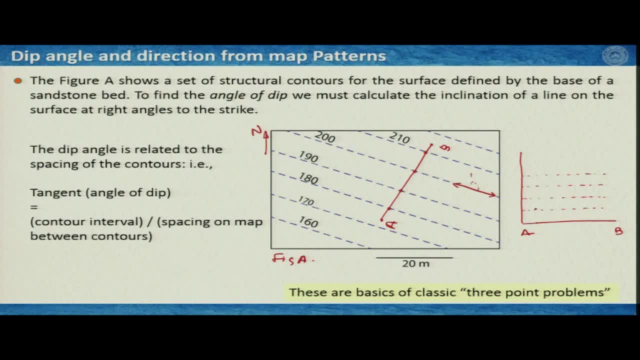 then 210.. At this point it cuts here, say. it cuts here, say this: 1,, 2,, 3,, 4.. So this is 1,, this is 2,, this is 3 and this is 4.. So it is possible that you can get a line. 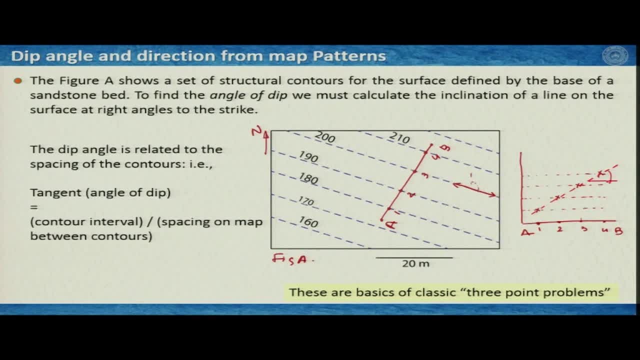 like this: and the slope of this line is actually the dip. Now how to calculate the slope? of course. So dip angle, as it is written here, is related to the spacing of the contours. that is tangent, or angle of dip is contour interval. So in this case this is 10 meters divided by spacing. 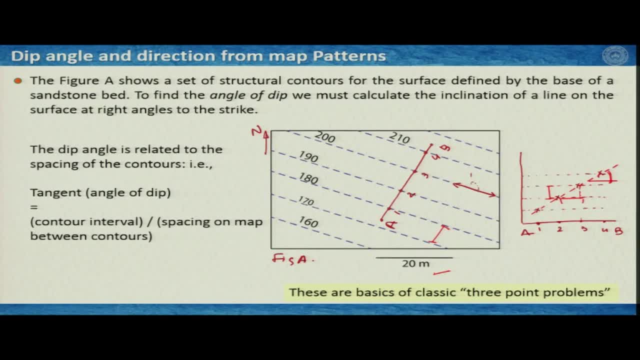 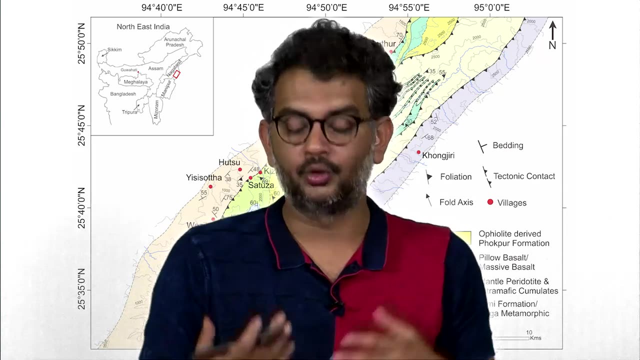 on map between the contours and this is exactly what you can figure out. So once you know the dip and strike from the topographic map, these kind of basics actually help you to understand the problems like three-point problem and so on, particularly when people do borehole in area, they do not see the actual rock. 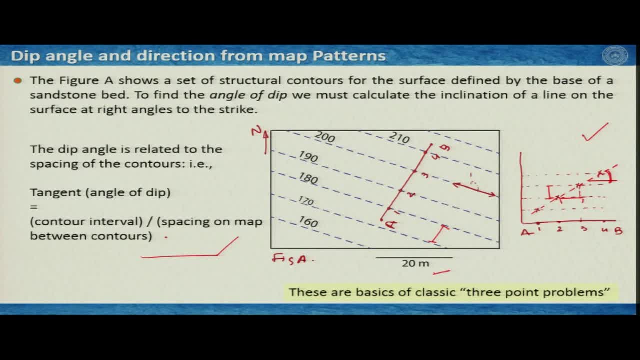 So what I mean by this? let us take a very simple block diagram. So you have a dipping plane at the sub-surface and this is of your interest and what you doing? you doing some bore holes. you have done one. 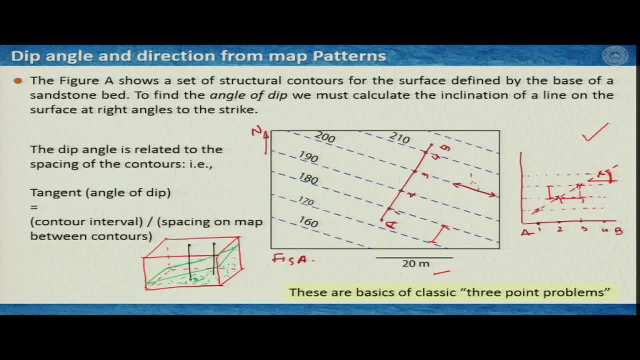 borehole: here, you get something here, you get something here, and maybe one here, you get something here. So every time you touch your desired bed at different points. So here on the plan you actually have three points where you touch the desired bed at three different. 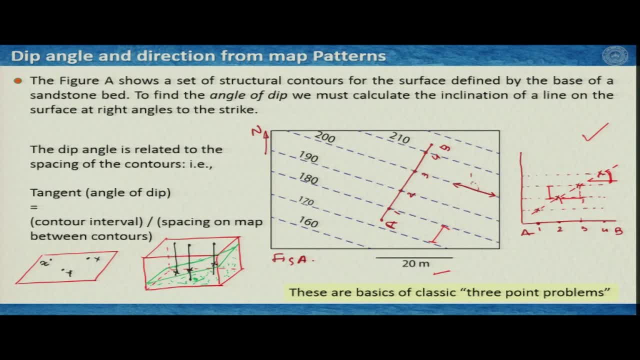 values, say x, y and z, And if you are sure that this is an uniformly dipping bed, then using this basic of finding dip and strike, you can figure out that what is the dip and strike of this bed which you actually do not see? So this is something. 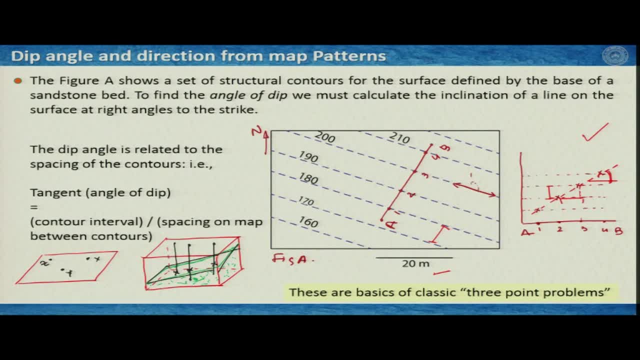 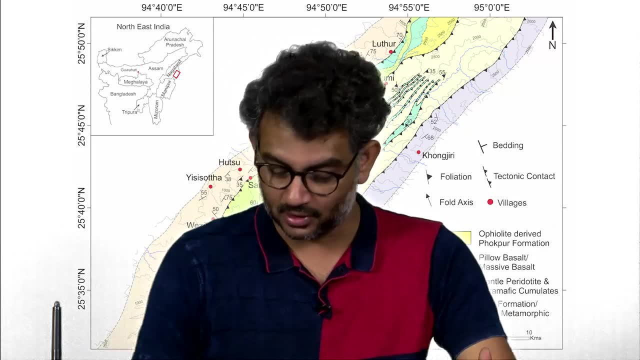 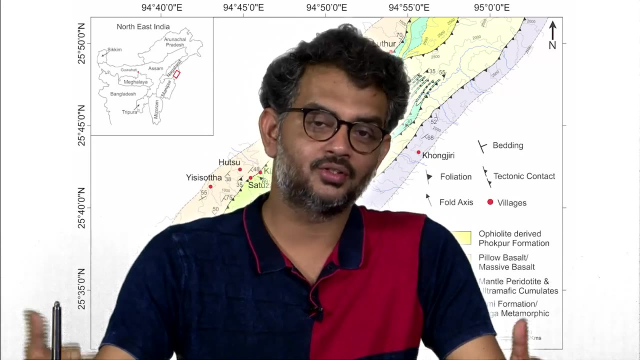 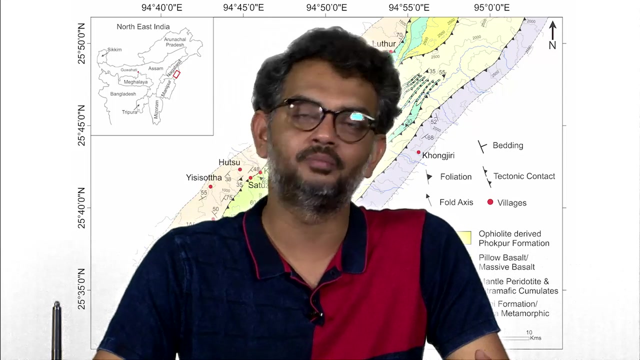 very interesting of this kind of problems. there should be some problems associated with this, and the demonstrations of this lab works would be given along with this this week's lecture series. So with this I conclude this week's lecture, because we will have a handful of demonstrations which are very useful and would be uploaded in this week by the teaching. 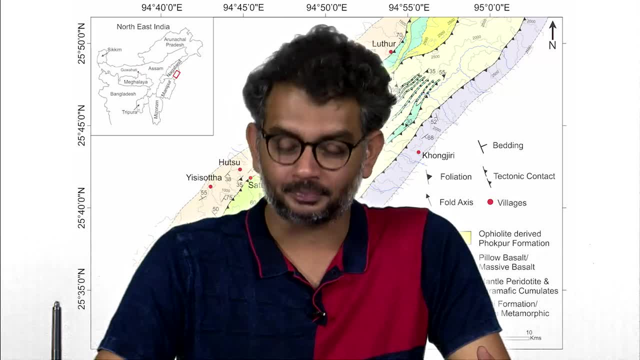 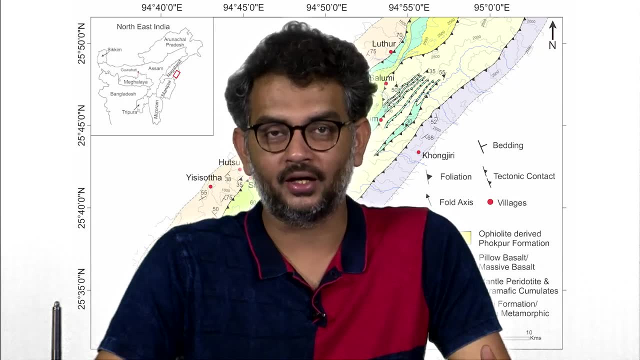 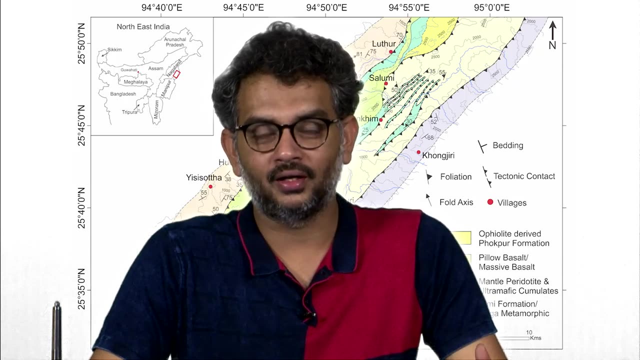 assistants, So I request you to check them and practice. I not only conclude the lecture of this week as your instructor, but I also sign off from this course because this is the last lecture. I thank you. Thank you very much for joining this course and I particularly enjoyed a lot in teaching. 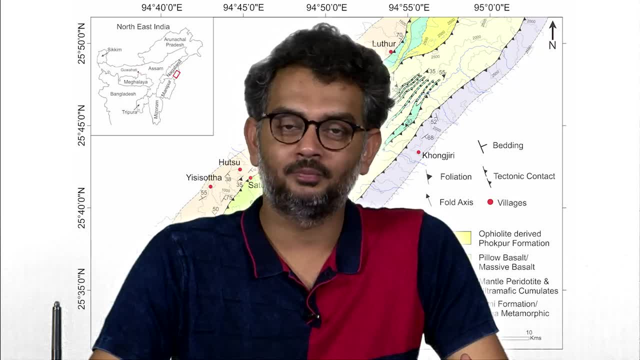 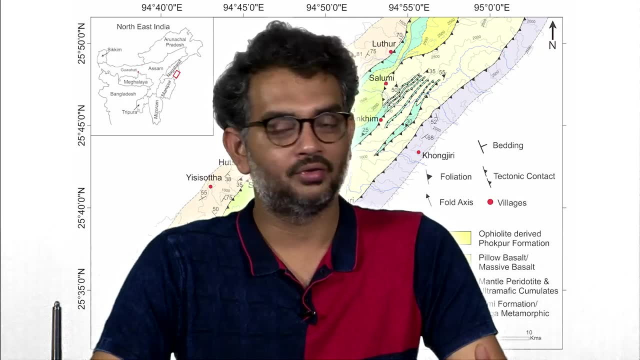 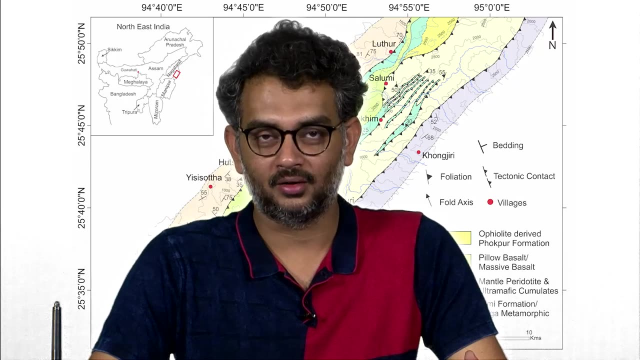 this course, I learnt a lot as well. I hope this course was useful for you, and I still remain at your disposal. If you have any ideas that you would like to discuss with me, you are more than welcome to write me through my email. So thank you very much. Stay well. 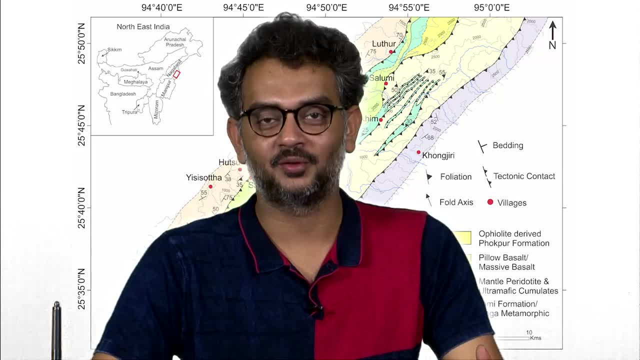 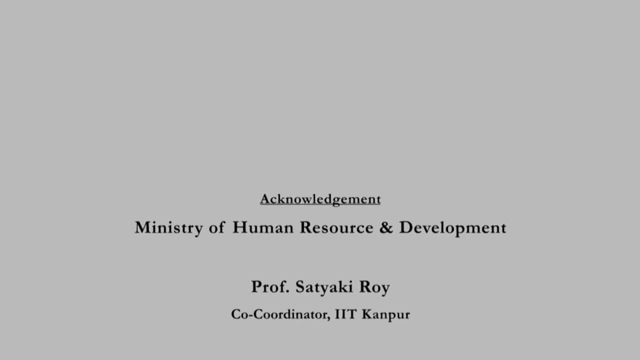 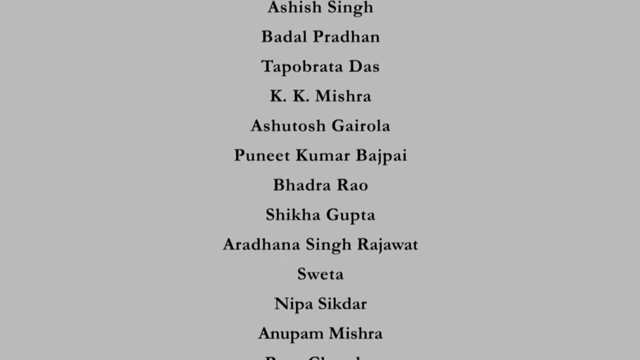 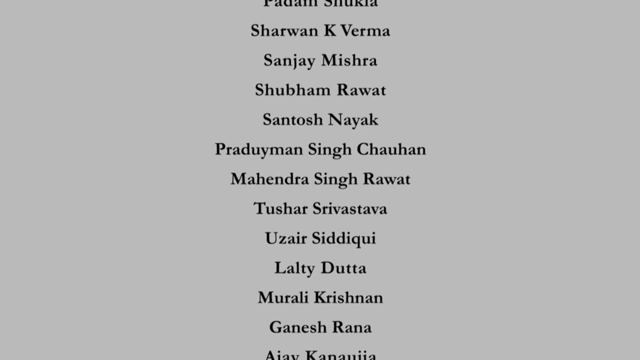 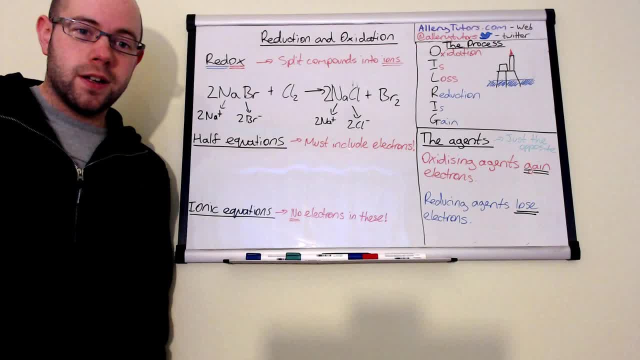 Hi everybody. my name is Chris Harris and I'm from AllergyTutorscom, and in this video we're going to look at reduction and oxidation. Now, reduction and oxidation is a process by which electrons are moved from one chemical and received by another one. So obviously, 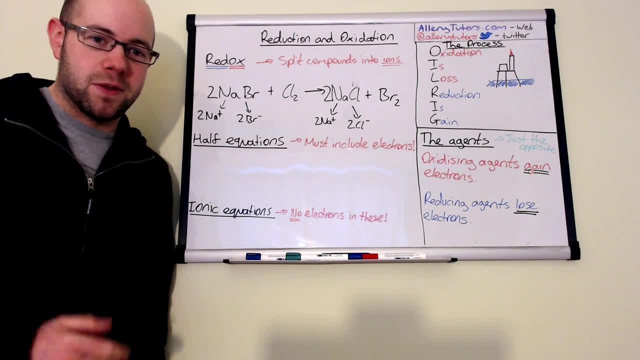 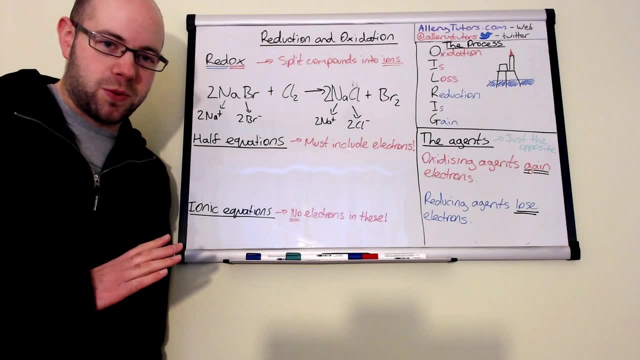 this is a very important part of chemistry, just by the nature of the process. In this video, we're going to look at the process of oxidation and reduction and we're going to look at the difference between that and oxidizing and reducing agents which are slightly different. 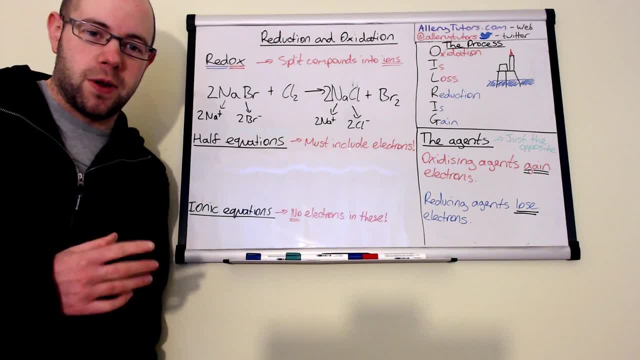 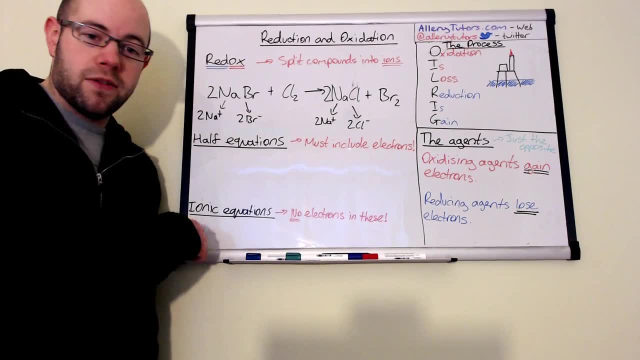 We're also going to look at redox reactions as well and what that means, and look at some of the spectator ions that are in our reaction. We're also going to look at half equations and ionic equations as well, and we're effectively going to construct them from a standard equation.